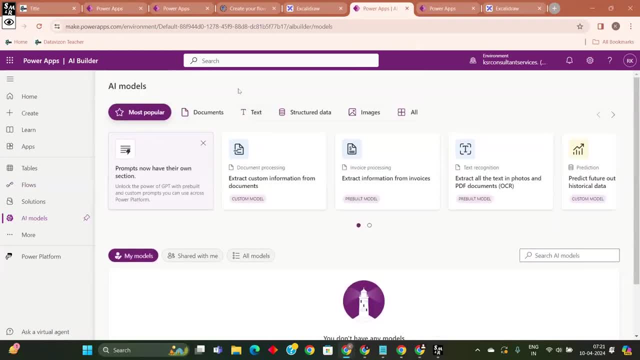 to AI Models. just see, These are the things, Okay. Document processing, invoice processing, text recognition, prediction and Calling� customer feedback. Okay, And these other types Under documents, we have this one: extract custom information from documents, Extra information from Invoices, extract all texts and Prt Disp Х. 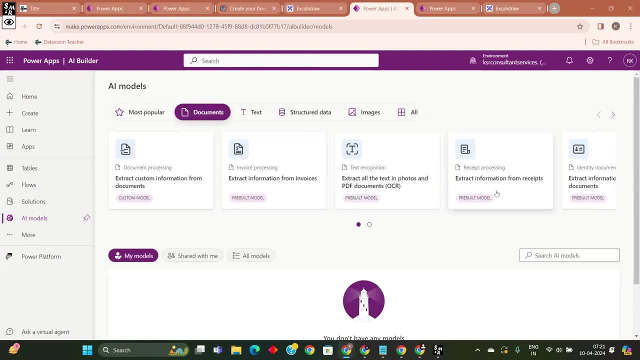 and PDF documents- Nothing but OCR- and extract invoiceíll for thes notes, which I already- information from receipts, extract information from identity document, extract information from business card- here the models are different, but the process is same. text text is nothing but uh, i'll see you in the use case. and here we have structured data. so here the question. 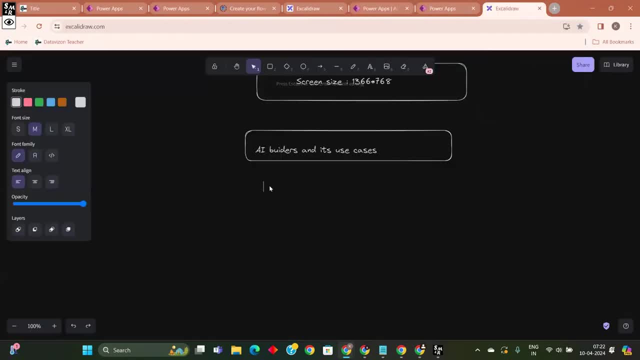 comes. when it comes to ai builder, the question comes in this manner: how many types of data we have, how many depth of data you have processed, processed using uh? ai builders are a builders are how many types of data you, how many types of, how many types, how many types of data we? 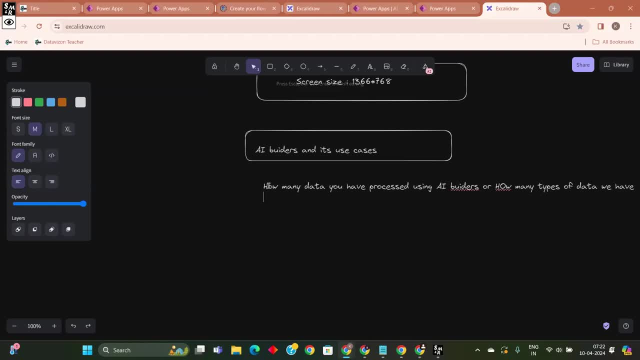 have. okay, so it's gonna be? the answer is pretty simple: structured, structured and unstructured. i'll give you understanding, better understanding, of structured and unstructured data. okay, structured and unstructured data. before i give you something about ai builder, let me give you a use case. 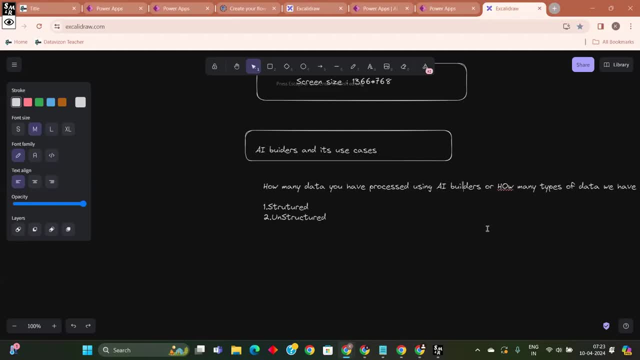 okay, suppose a sales team is there, uh in a company called uh, something we will get. we take in a company called uh, tata, tata water, water, tata water or britannia, what these companies do, actually tata instead of water. i will take it as fmcg. 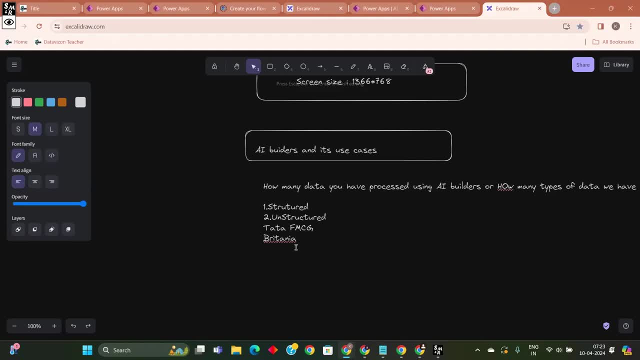 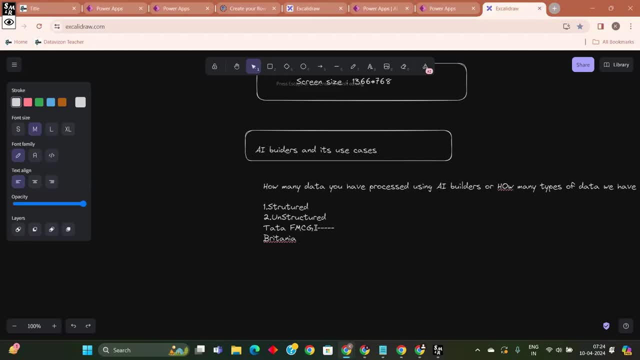 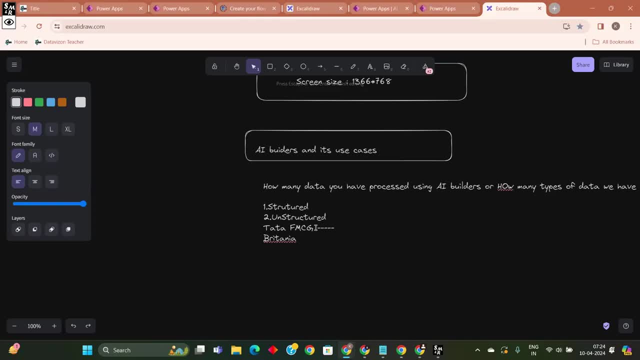 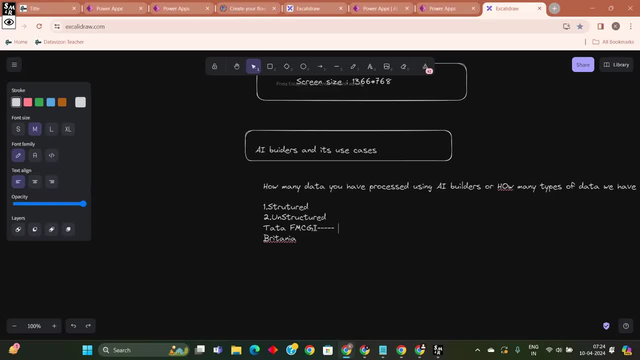 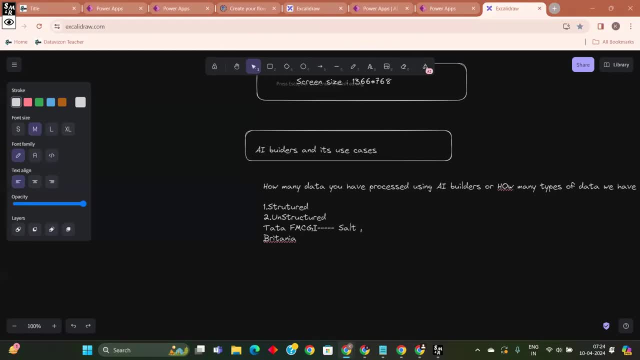 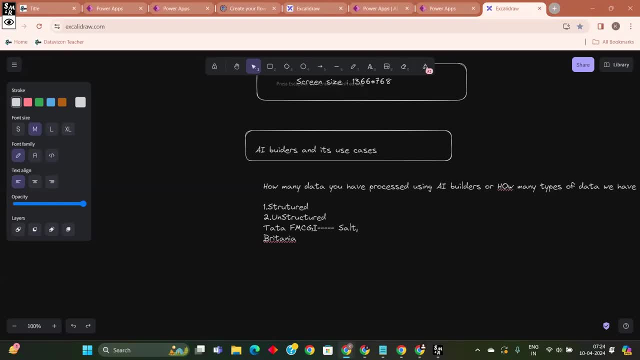 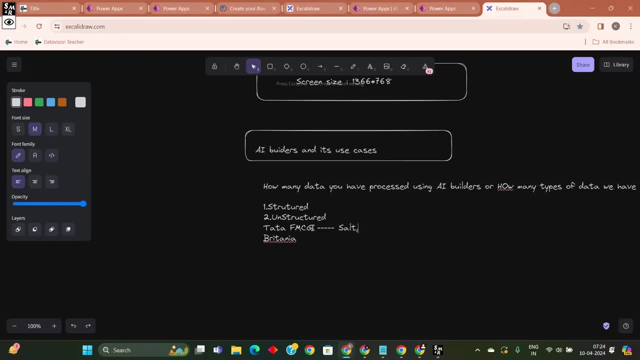 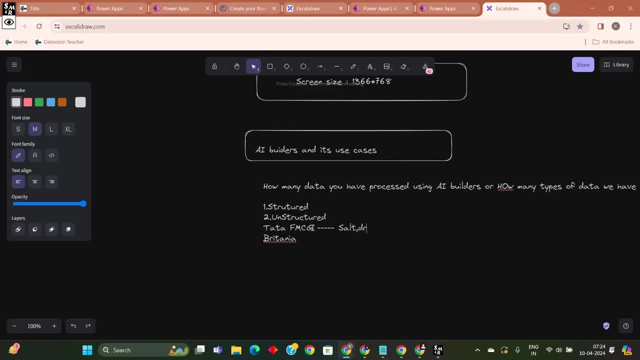 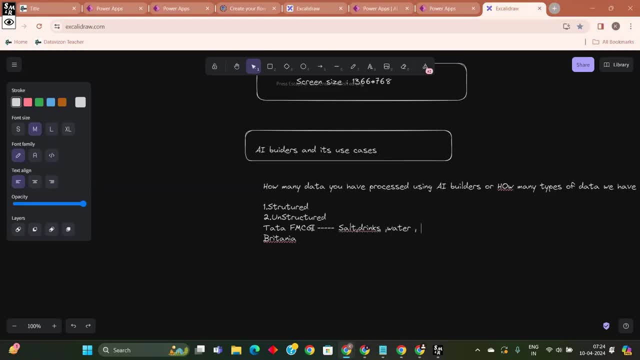 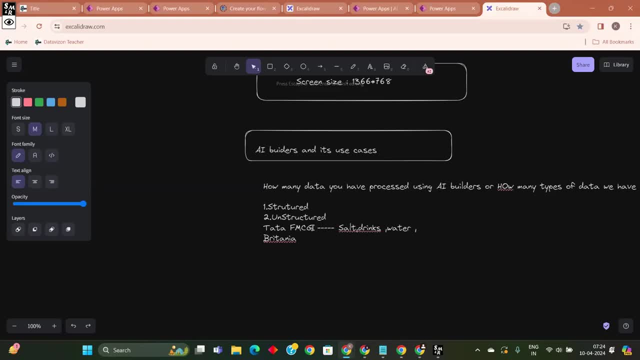 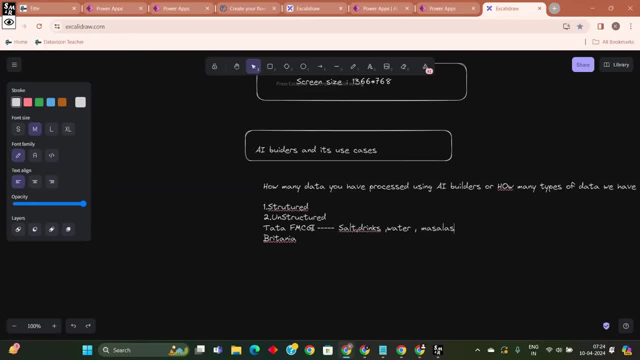 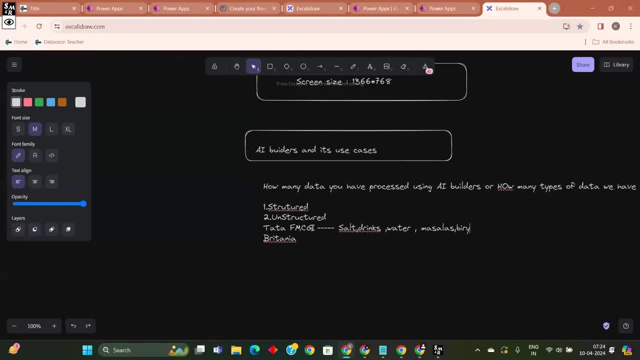 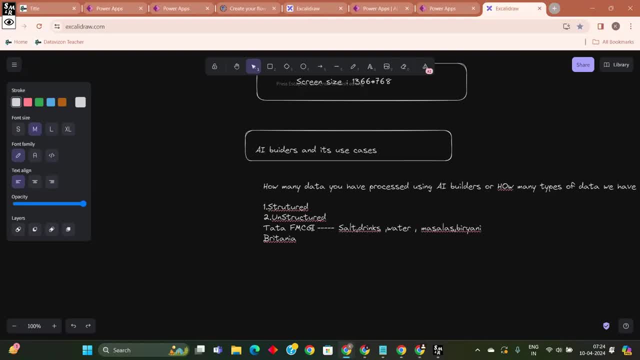 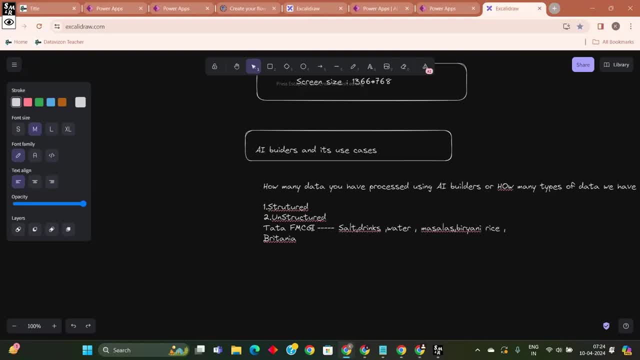 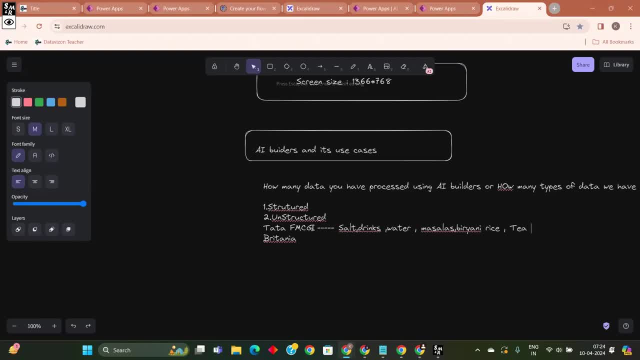 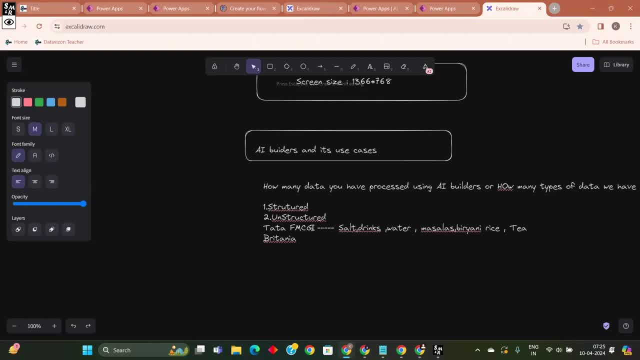 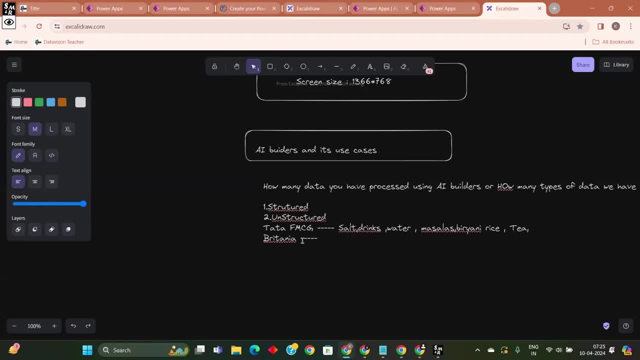 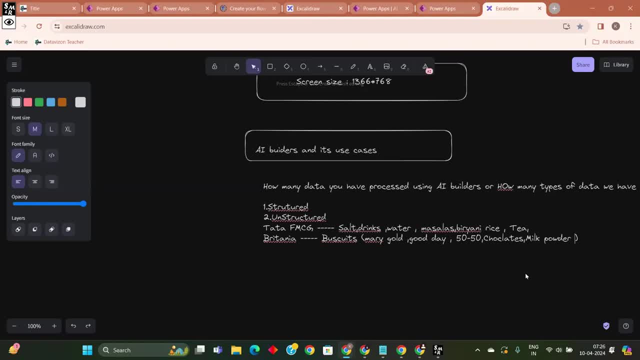 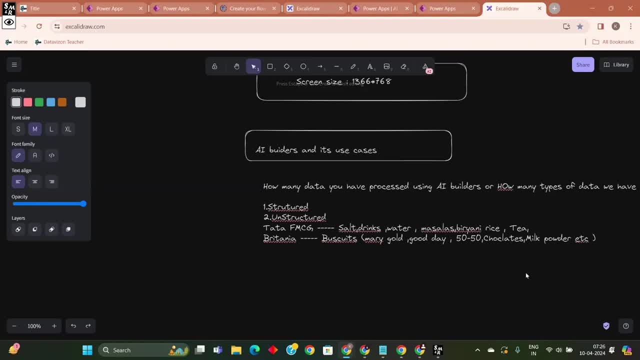 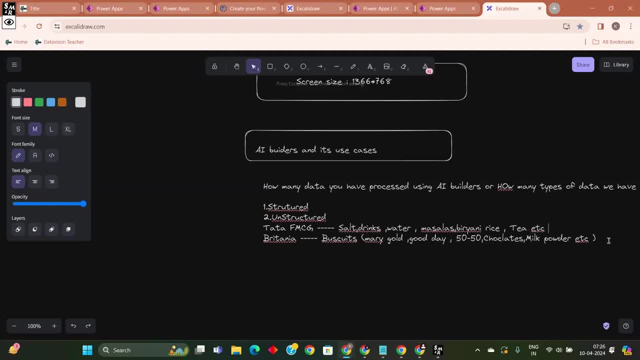 and what does britannia do? and what does britannia do discuss? and when it comes to amul, it is a dairy, it is a dairy product, it's a dairy company. dairy company, what does it do? it sell milk. it sell a curd ghee, paneer, curd lassi and all, exactly all the milk products. 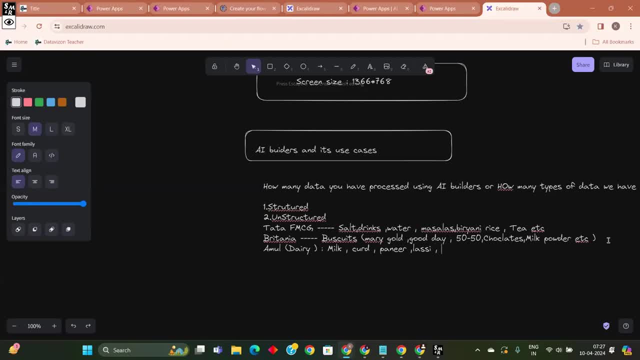 butter, ice cream, ice cream and yeah, etc. butter. i even britannia also sells butter. okay, uh, yes, so, so these are some of the fmcg. fmcg usually fast-moving customer goods. okay, now these companies are having some sales teams. suppose sales teams and how much sales teams they will have for each and every street. there will be more than 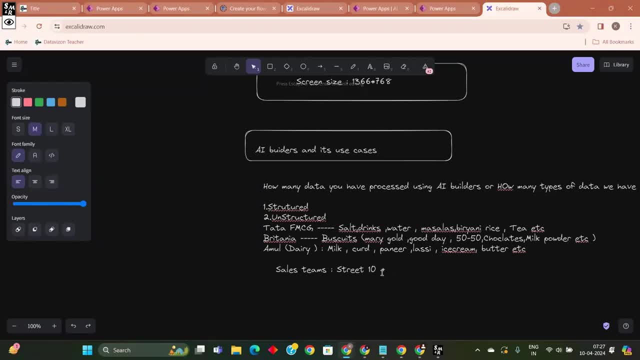 10 people. there will be more than 10 people. okay, 10 plus people. uh, for each street from india, wide, from complete india. okay, think of me like this: as you know, can i make just two or three rooms? okay, in every, from complete country. so, from complete country. they will have nearly 10 sales team, a team of 10. for each street and in a complete car, in a big company like company like india, you can consider that there will be some somewhere around 30 000 plus major streets or areas. you can say 30 000 plus areas and into 10, into 10, how much will be the total? how much will be the total? 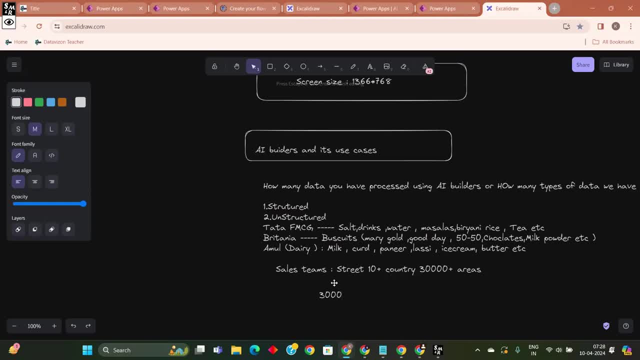 ah, 30 000 into 10. how much. i'm pretty poor in maths. that's the reason i'm asking you the answer. what's the answer? 30 000 into 10? yes, exactly yeah. that is the answer, not three lakh sales people for each and company. 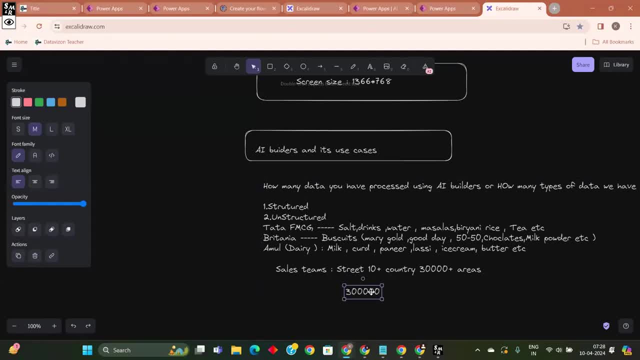 uh, we are assuming, and they will be every day. they will be traveling on their bikes and or else some transport medium. they will use car or vehicle or some trolley and they will be like reaching each and every show, each and every store, to take the orders from various uh shops and supermarkets. 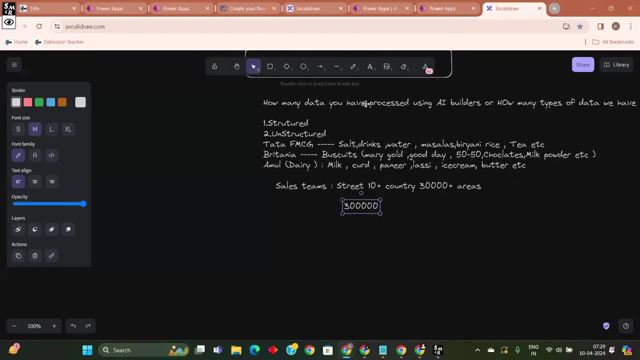 three lakh people and for three lakh people will keep a keep a petrol bill. so this is a use case. they will keep a petrol bill. and this is a small minor activity. if they send a screenshot to their supervisor or manager, he can also process, but the supervisor or 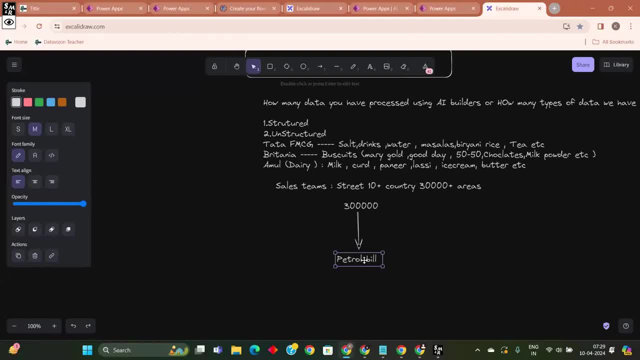 manager is not an accounts team person, okay, so the bill should be reached to the accounting account team. so what? the what we will do is in this scenario, this petrol bill detail should be filled in an application. so this is an application here. this is an application, and all these three lakhs people, daily, daily, daily, daily, they will, they will, they need to. 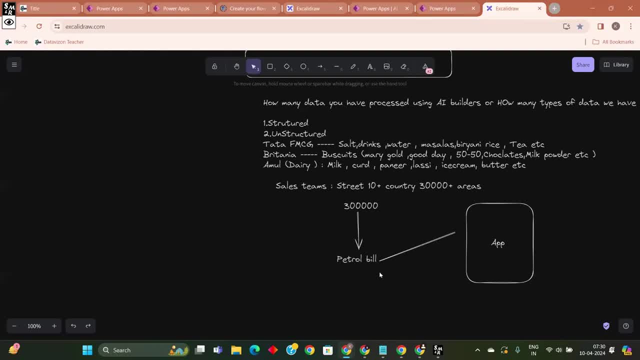 suffer. the submit the petrol bill and calculated and some people, some companies, will give their daily petrol bill, or else some companies will give uh a monthly petrol bill, but the thing is that they should upload their petrol bill daily. daily monthly bills are not accepted because if, if someone uh. keeps a complete monthly bill, he may give a wrong entry or else he may miss some of the dates. that is the reason mostly petrol bill will be calculated daily wise. or else they will keep a petrol bill and here sales team will not have any kind of restriction. they can reach out to anything today. 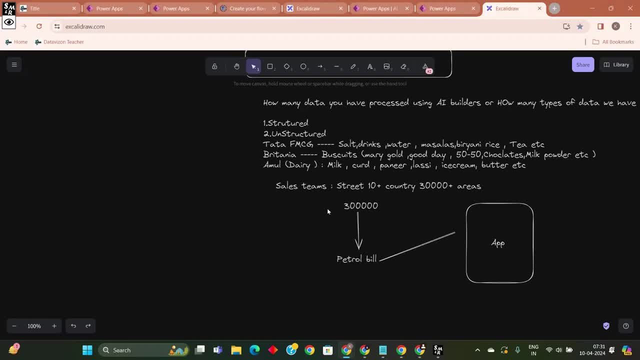 they will reach some, some. they will cover some two kilometers. tomorrow they may cover 20 kilometers. because sales are not happening. they need to get more and more customers. then only production will increase, company's profit will increase. now, this is the main synopsis of sales. sales will never. 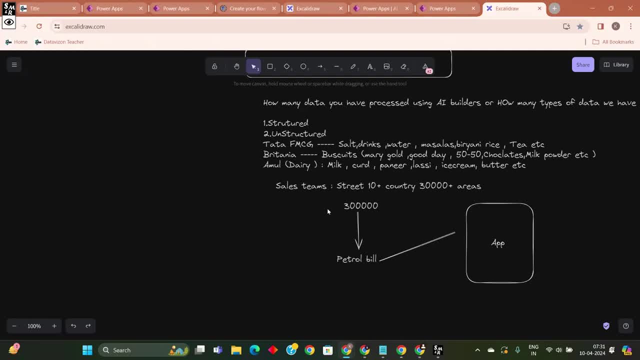 stop, your production will stop your application developer development will stop for certain certain stage if the product is uh ending and product you uh. your company fulfills the product of the software product uh development. but sales is a continuous iteration. it should not stop. if it should not stop, the fuel should be produced. 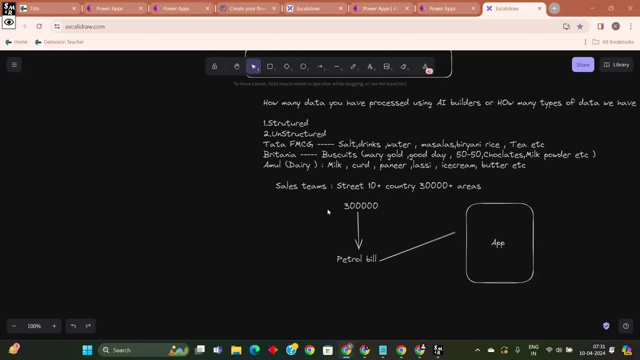 along with the salaries, what the company gives to the sales team. they also should, uh, produce a petrol bill because they are moving around the country or moving around the street or moving around a district for the welfare of the company. so company should take care of the petrol belief. 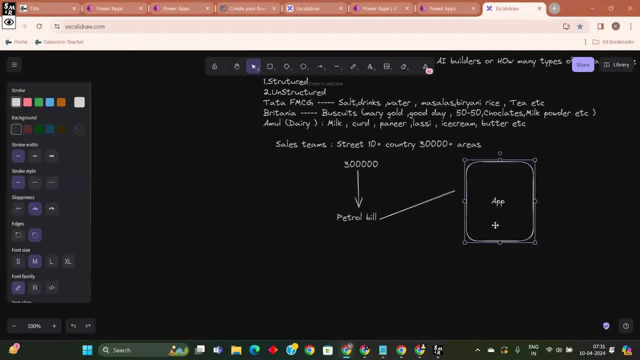 petrol bill is not given no sales company, no sales guy will work okay. so this is the, this is the one thing, and uh, they should upload this petrol bill into the app. if it is a small company company is like, uh, uh. so ksr recently started an fmcg company. ksr recently started ksr fmcg products. 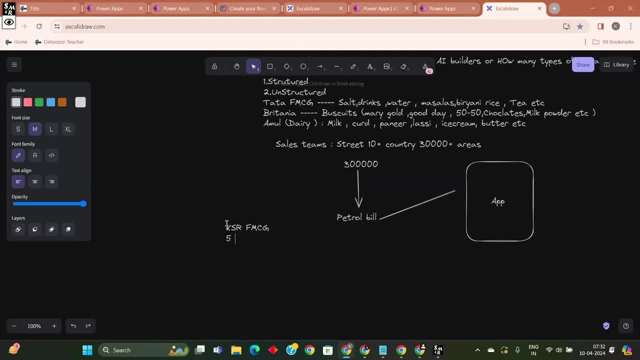 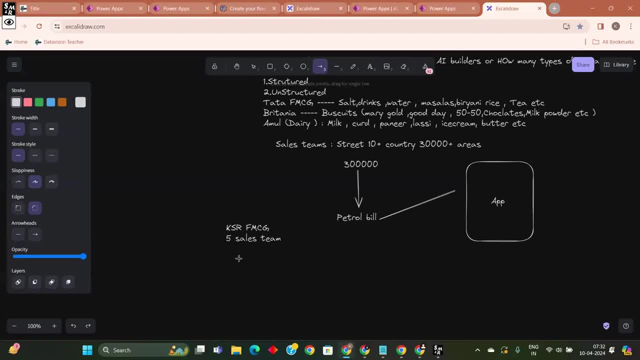 uh, accounts department, uh, accounts department, accounts department. so from here accounts department, so from here accounts department. so from here they will sell to send it to manager and they will sell to send it to manager and they will sell to send it to manager and manager, manager, manager will approve. 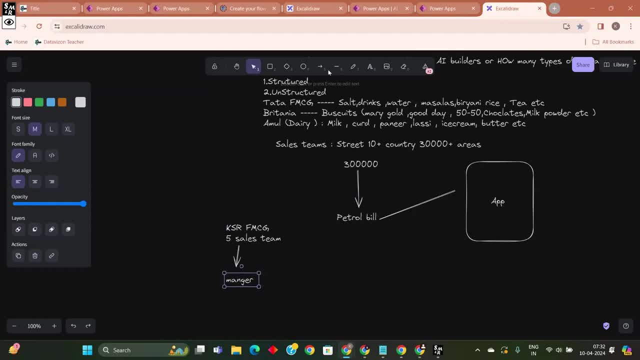 manager and manager will directly send to manager and manager will directly send to manager and manager will directly send to sales team: sorry accounts team, sorry accounts team, sorry accounts team. and here it is a easy process because we- and here it is a easy process because we- and here it is a easy process because we have recently started, we are a small. 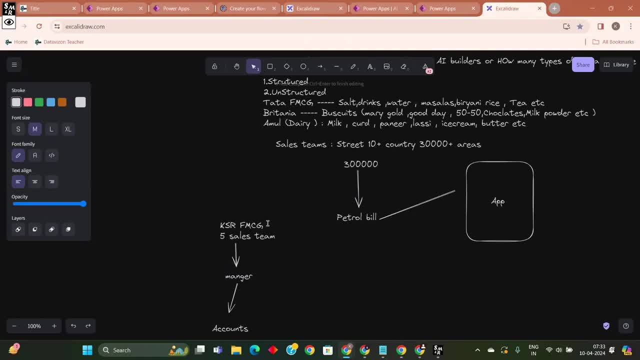 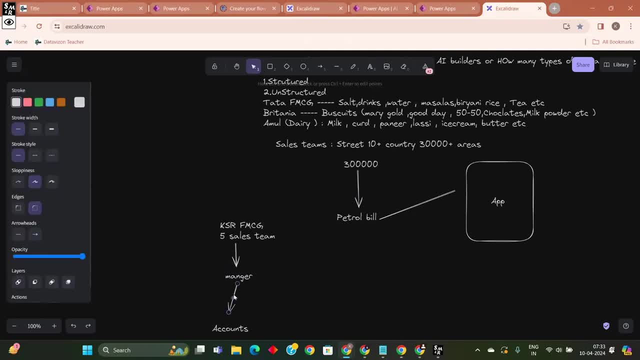 in terms of training. in terms of training, we are one of one amongst the top. we are one of one amongst the top. we are one of one amongst the top and we are the direct microsoft partners. and we are the direct microsoft partners and we are the direct microsoft partners, but one: our, what we call our management. 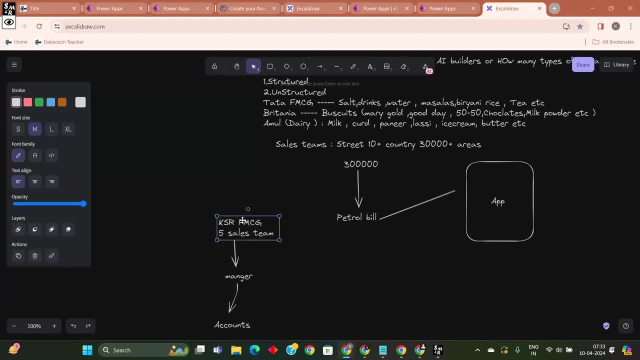 but one our what we call our management, but one our what we call our management- got an idea and they want to go into got an idea. and they want to go into got an idea and they want to go into fmcg products. and here we started with. 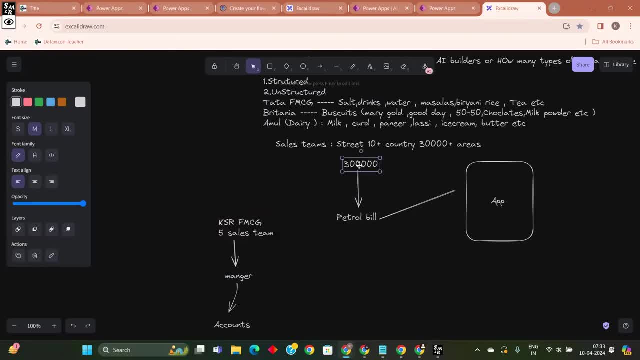 fmcg products. and here we started with fmcg products. and here we started with justify team: here it is possible. but a justify team: here it is possible. but a justify team here it is possible. but a company like amul, a company like company like amul, a company like company like amul, a company like britannia. a company like tata, a company britannia, a company like tata, a company britannia. a company like tata. a company like itc will have nearly 3 lakh sales. like itc will have nearly 3 lakh sales. 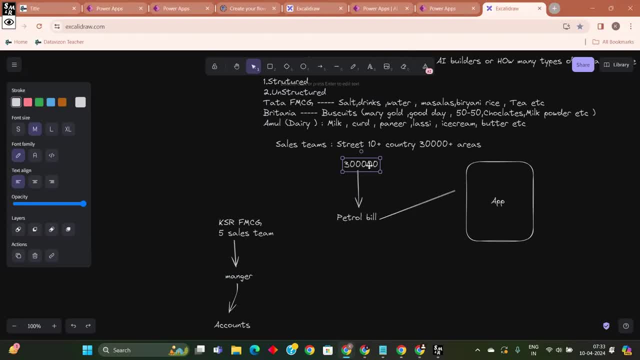 like itc, will have nearly 3 lakh sales people, people, people- they may be contract based or they may they may be contract based or they may. they may be contract based or they may be permanent. but nearly this thing, this be permanent. but nearly this thing, this. 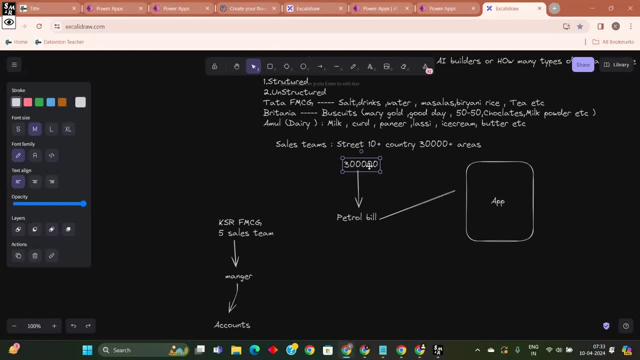 be permanent. but nearly this thing, this, this volume of sales team, is possible. this volume of sales team is possible. this volume of sales team is possible for fmcg and fmcg is such a for fmcg and fmcg is such a for fmcg and fmcg is such a. such a kind of uh market is that. 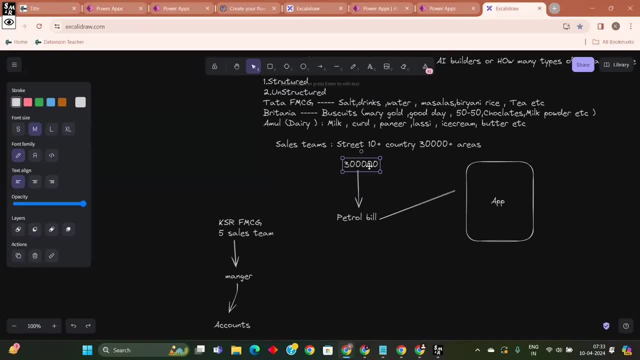 such a kind of uh market? is that such a kind of uh market? is that daily you should show ads. daily you should show ads. daily you should show ads. take a take coca-cola or thumbs up. take a take coca-cola or thumbs up. 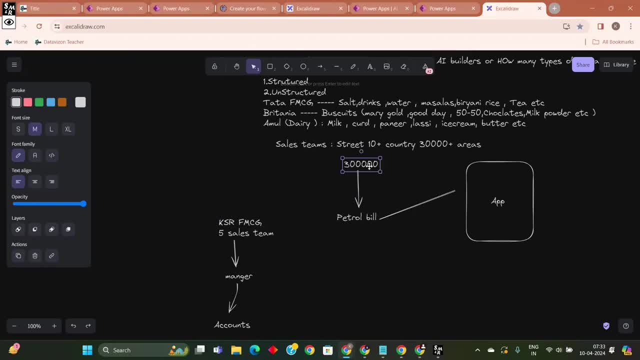 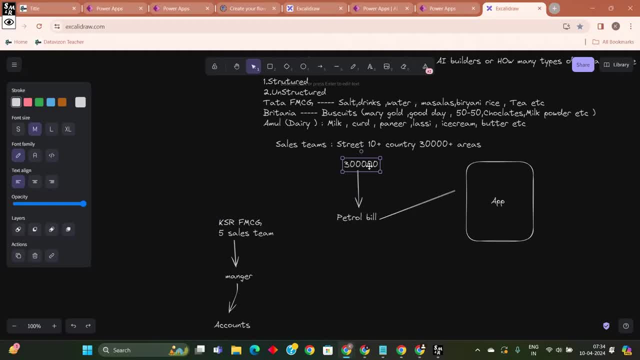 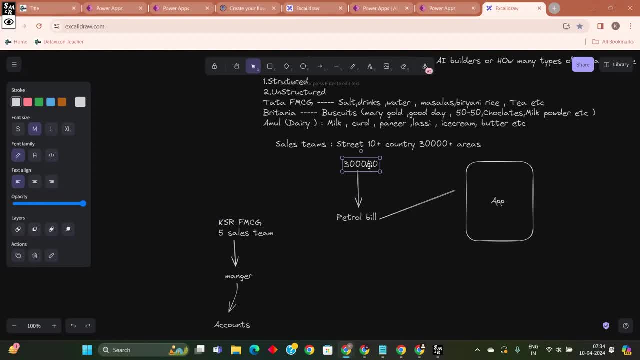 minute, we will get ads, because if they minute we will get ads, because if they, if they won't give ads, we will forget the. if they won't give ads, we will forget the. if they won't give ads, we will forget the product and we will not buy. this is a. 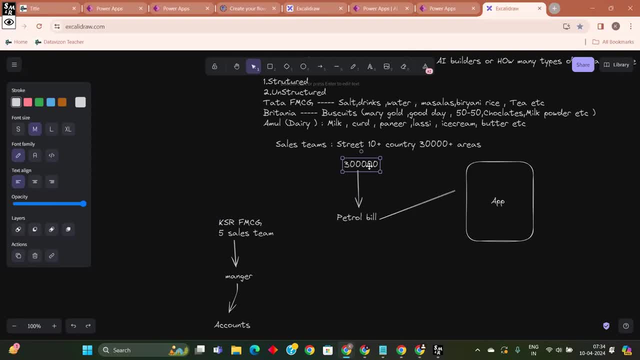 product and we will not buy. this is a product and we will not buy. this is a peer, peer, peer. in the same way sales team with the. in the same way sales team with the. in the same way sales team with the sales team which will move around, uh. 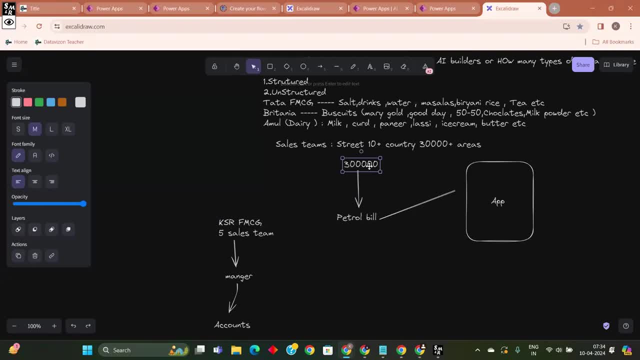 sales team which will move around. uh, sales team which will move around. uh, working, we move around working hours, working. we move around working hours, working. we move around working hours across the across the streets or the across the across the streets or the across the across the streets or the districts, to increase the sales. 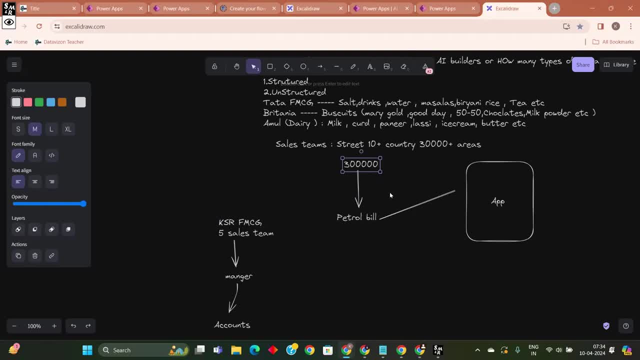 districts to increase the sales districts, to increase the sales. particular vacancies: particular vacancies: particular vacancies: our use case with the air builder is our use case with the air builder is: our use case with the air builder is when a petrol bill is uploaded. when a petrol bill is uploaded. 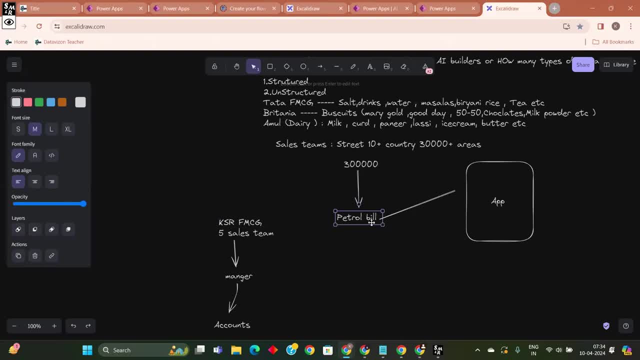 when a petrol bill is uploaded, uh approval should come and the amount uh approval should come, and the amount uh approval should come and the amount should reach out to the. this exact detail should reach out to this exact detail should reach out to this exact detail should reach out to the account stream directly and petrol. 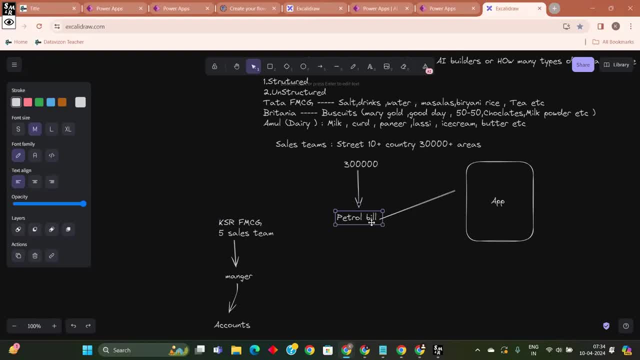 the account stream directly and petrol the account stream directly and petrol. petrol bill should be approved. petrol bill should be approved. petrol bill should be approved. and do you see that when you get a? and do you see that when you get a? and do you see that when you get a petrol bill, in what format the petrol will? 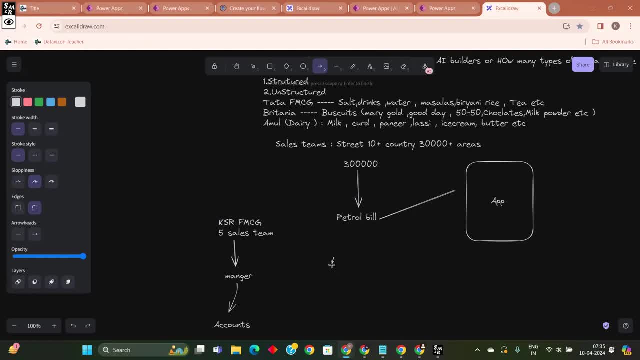 petrol bill. in what format the petrol will petrol bill. in what format the petrol will will be. format of petrol bill: date is there? uh, they are feeds. i am asking you the? uh, they are feeds. i am asking you the? uh, they are feeds. i am asking you the format. 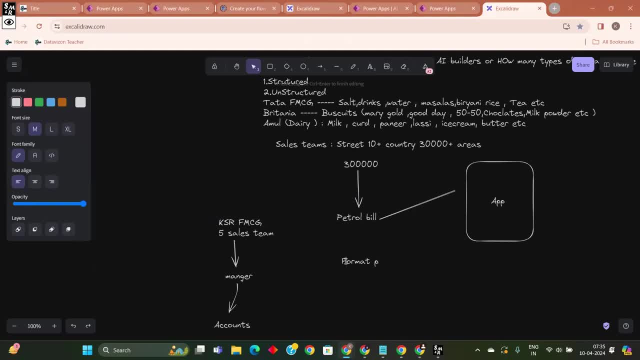 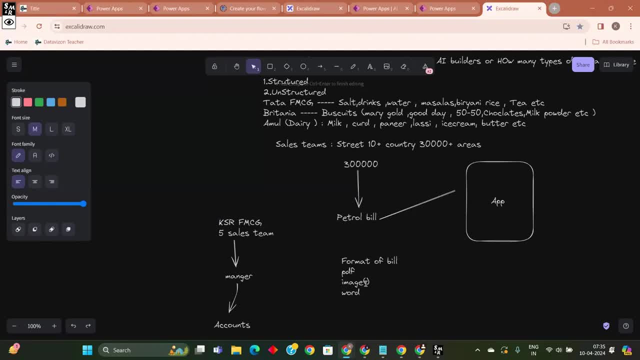 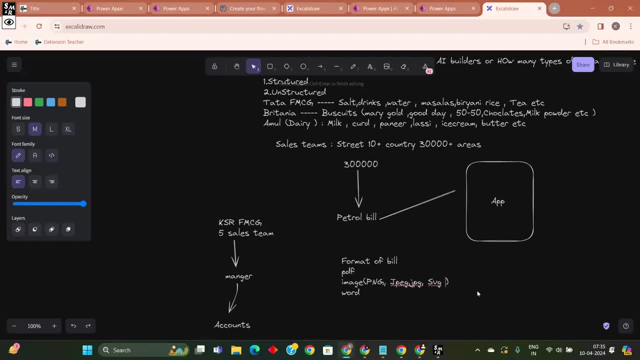 and and svg format. svg format. svg format, etc. etc. etc. ok, these are the formats we have. it may. ok, these are the formats we have. it may. ok, these are the formats we have. it may be in pdf. it may be in image. it may be be in pdf. it may be in image. it may be. 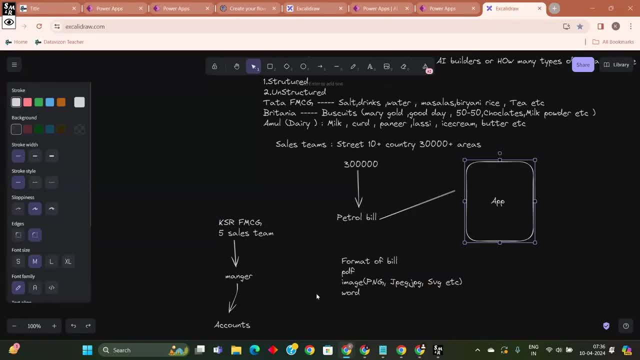 be in pdf, it may be in image, it may be in word. if we just give a update option in word, if we just give a update option in word, if we just give a update option, again it will be a problem for the. again it will be a problem for the. 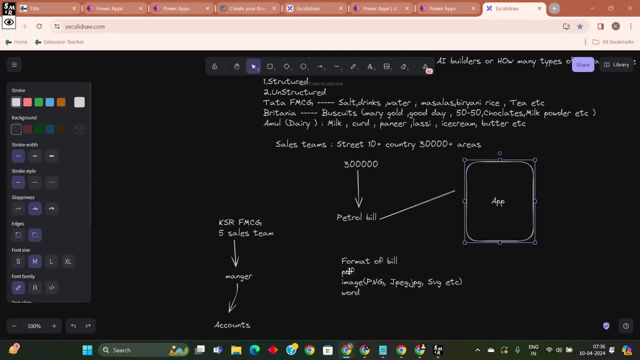 again, it will be a problem for the someone to sort, even for the software, someone to sort even for the software, someone to sort, even for the software also. it is a problem for software to also. it is a problem for software to also. it is a problem for software to sort, because it is not just a five. 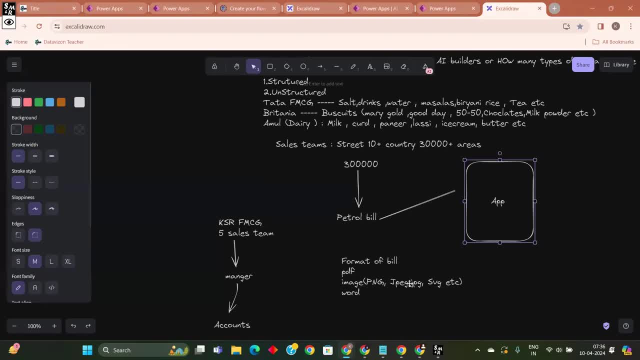 sort, because it is not just a five sort, because it is not just a five number, team number, team number, team: 10s are 20s are 50s will be the maximum. 10s are 20s are 50s will be the maximum. 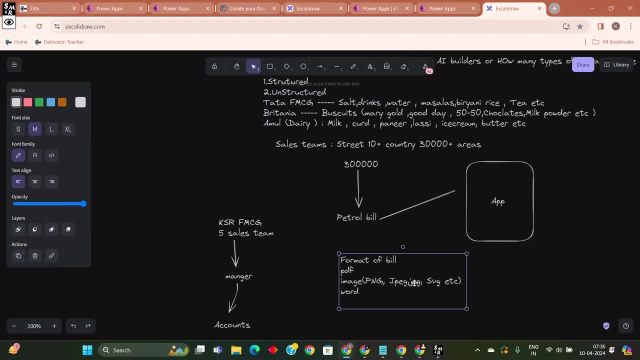 10s are 20s are 50s will be the maximum for a accounts team in a company, in a for a accounts team in a company. in a for a accounts team in a company. in a big company like daylight also the big company like daylight also the. 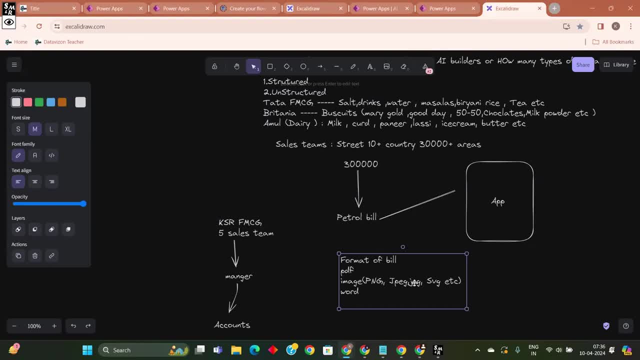 big company like daylight. also, the accounts will be subjected to only 50 accounts will be subjected to only 50 accounts will be subjected to only 50 members. members, members, okay, and 50 members- do you feel that it okay? and 50 members: do you feel that it? 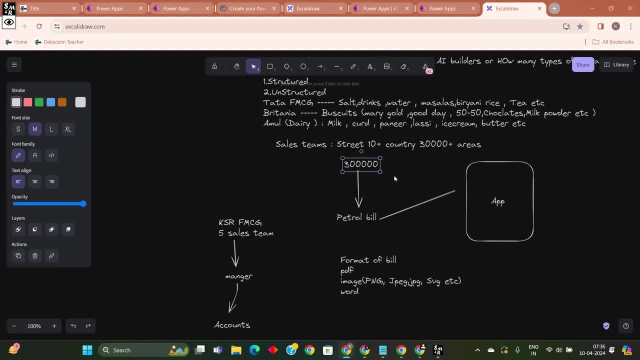 okay, and 50 members. do you feel that it is that much easy to uh evaluate all? is that much easy to uh evaluate all? is that much easy to uh evaluate all the 3000 uh uh petrol bills? is it the 3000 uh uh petrol bills, is it? 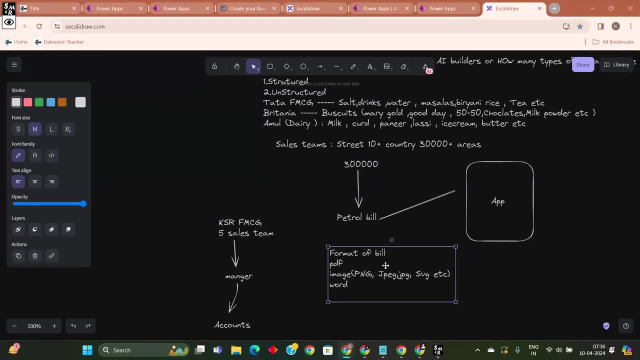 the 3000, uh uh, petrol bills. is it possible in a day? possible in a day? possible in a day? no, not possible. 50, 50, 50 people need to. no, not possible. 50, 50, 50 people need to- no, not possible. 50, 50, 50 people need to take care of just a petrol bill and do. 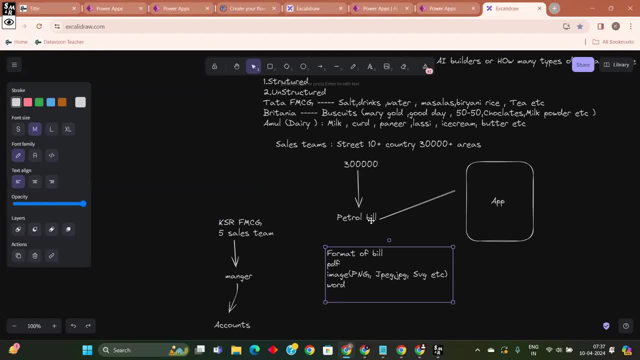 take care of just a petrol bill, and do take care of just a petrol bill. and do you feel that accounts team is having you feel that accounts team is having you feel that accounts team is having only duty of just taking care of the only duty of just taking care of the? 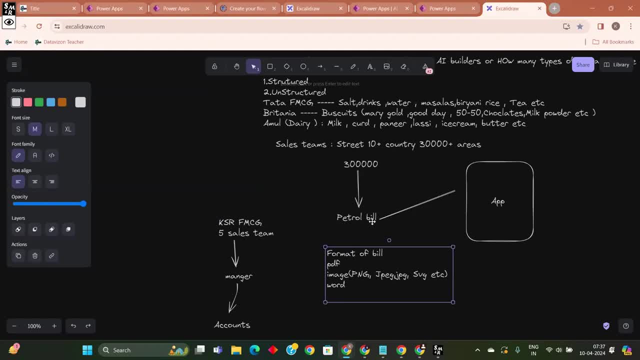 only duty of just taking care of the sales team petrol bill. sales team petrol bill. sales team petrol bill. they need to pay the expenses of the. they need to pay the expenses of the. they need to pay the expenses of the production, production, production. they need to collect the amounts from. 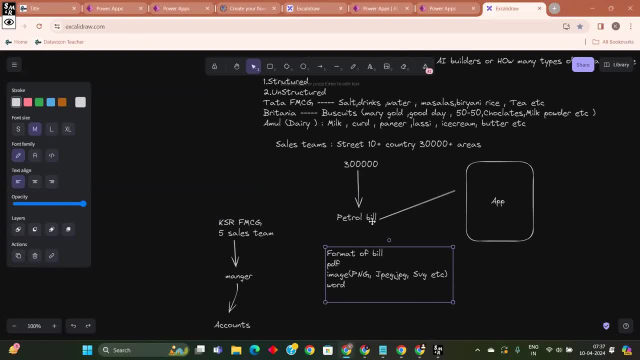 they need to collect the amounts from. they need to collect the amounts from their dealers, their dealers, their dealers. okay, they need to release the salaries of. okay, they need to release the salaries of. okay, they need to release the salaries of remaining employees. remaining employees, remaining employees. they need to pay rents for the lands. 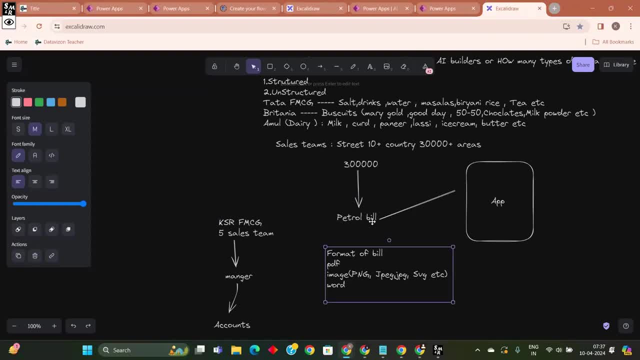 they need to pay rents for the lands. they need to pay rents for the lands which they have taken. they need to pay money for the. they need to pay money for the. they need to pay money for the. uh uh uh. raw material, raw material, raw material. okay, in order. what is the raw material? 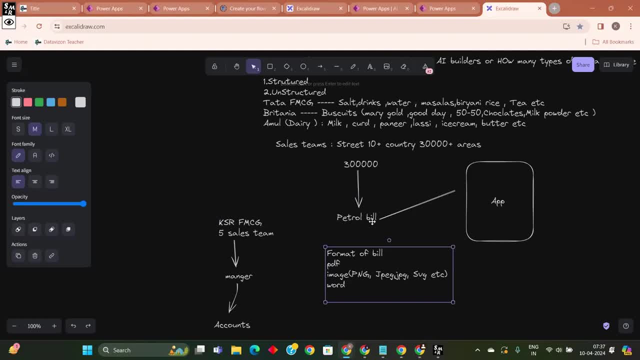 okay, in order. what is the raw material? okay, in order. what is the raw material to make biscuits? biscuits wheat or maida good, wheat or maida good, wheat or maida good, okay, and water for packaging: okay, and water for packaging: okay, and water for packaging. for packaging also. we 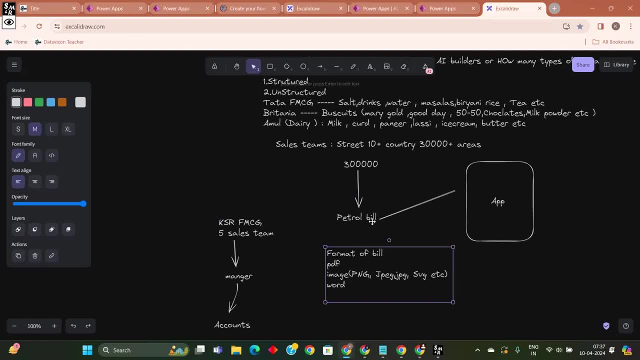 for packaging also. we for packaging also. we should. for packaging also, we should get some raw material correct, get some raw material correct, get some raw material correct. huh, these are all the other activities. huh, these are all the other activities. huh, these are all the other activities. that account stream should pay, that pay. 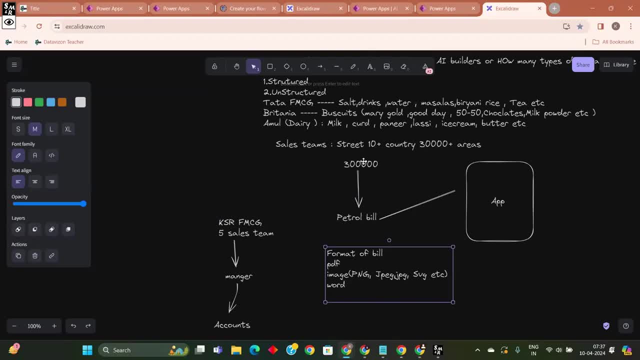 that account stream should pay that pay. that account stream should pay that, pay that pay the bills for. if they keep on that pay the bills for, if they keep on that pay the bills for, if they keep on just just just reading the petrol bill, it will be a 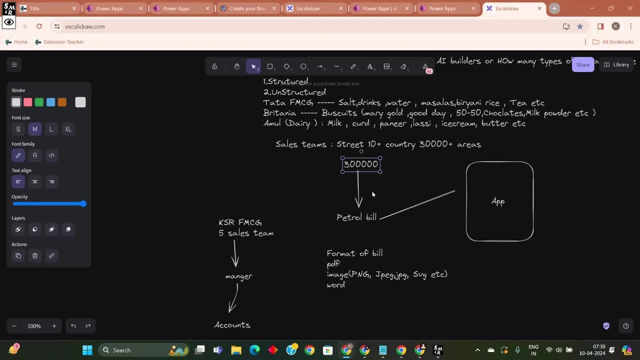 reading the petrol bill. it will be a reading the petrol bill. it will be a waste of time and production. i mean waste of time and production. i mean waste of time and production. i mean productivity of the account stream. will productivity of the account stream will productivity of the account stream will reduce. 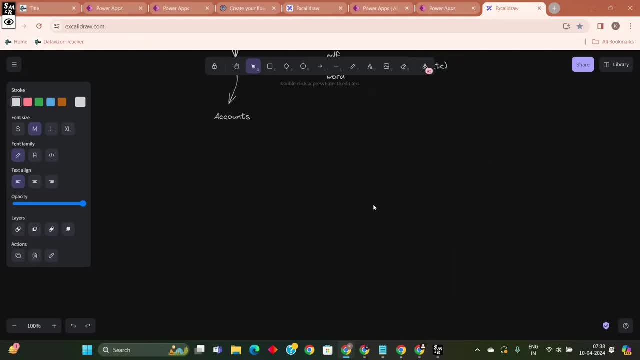 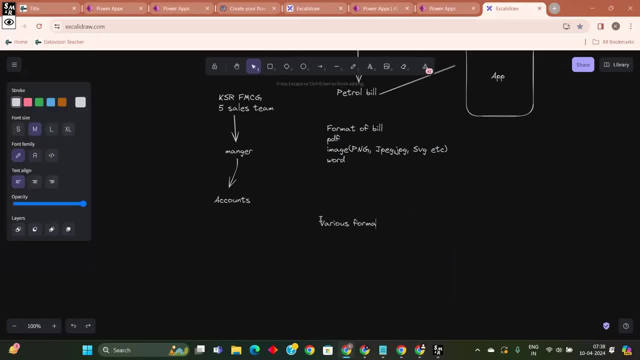 we will get various bills, various formats. we will get various bills, various formats of the bills, of the bills, of the bills, various, various, various formats of the bill. okay, various formats of formats of the bill. okay, various formats of formats of the bill. okay, various formats of the bill. 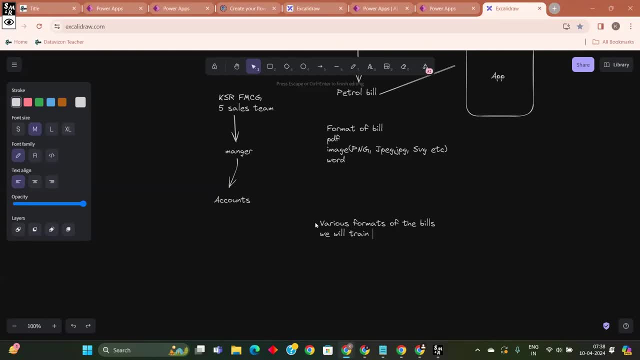 the bill, the bill, and we will, and we will, and we will train the ai model. we will train the ai, train the ai model. we will train the ai, train the ai model. we will train the ai model, model, model, so that it captures the fields. no, the no. 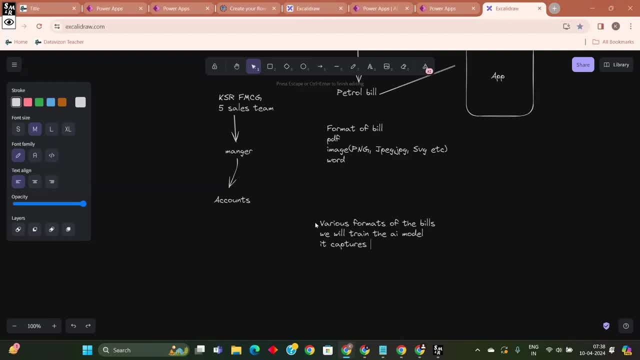 so that it captures the fields? no the no. so that it captures the fields. no the no. same in the fields, same in the fields, same in the fields. someone started saying date, etc, etc. it. someone started saying date, etc, etc. it. someone started saying date, etc, etc. it captures the. 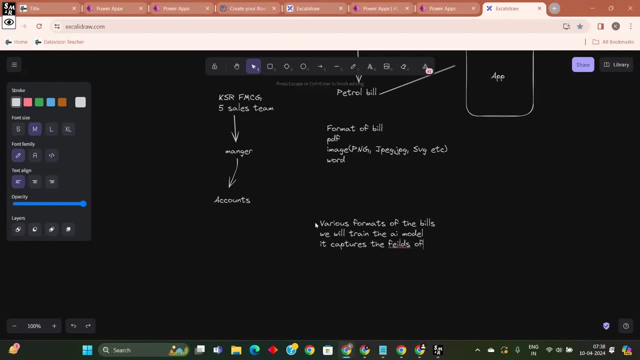 captures the captures the. it captures the fields. it captures the. it captures the fields. it captures the. it captures the fields. it captures the fields of fields, of fields, of the uh, the uh, the uh bill. no semi, what can be the fields? what can? no semi, what can be the fields? what can? 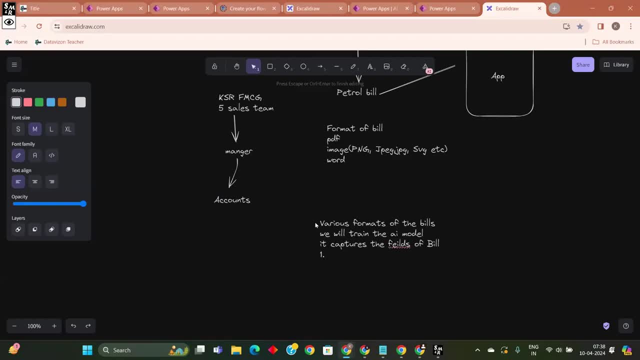 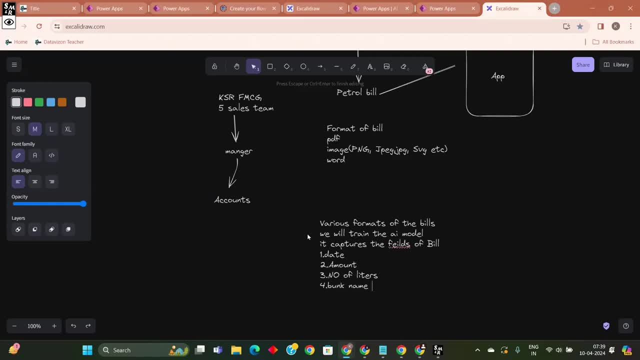 i mean the company name in the sense a, i mean the company name in the sense a: petrol bunk name, petrol bunk name, petrol bunk name, bunk name, correct, correct, correct, and we can also take that state also, and we can also take that state also, and we can also take that state also: location. 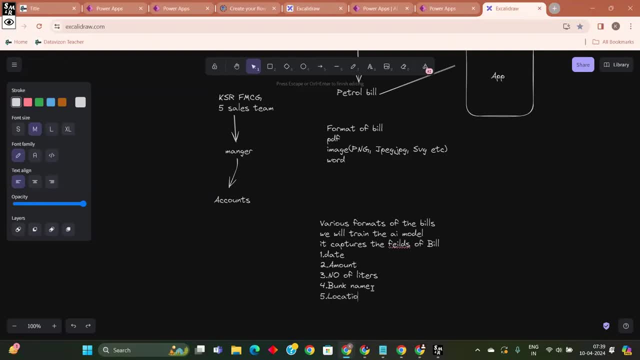 location, location, exactly location, because our sales team are across, because our sales team are across, because our sales team are across india. so they also need to get a location india. so they also need to get a location because in some question, in some, because in some question, in some, 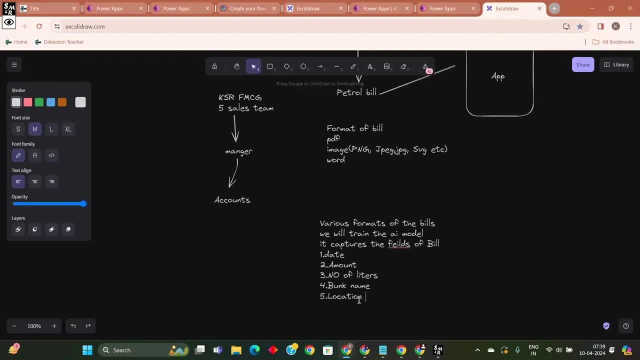 because in some question, in some, in some locations the petrol cost will be 100. in some locations the petrol cost will be 100. in some locations the petrol cost will be 100 in some code. in some locations it will. in some code: in some locations it will. 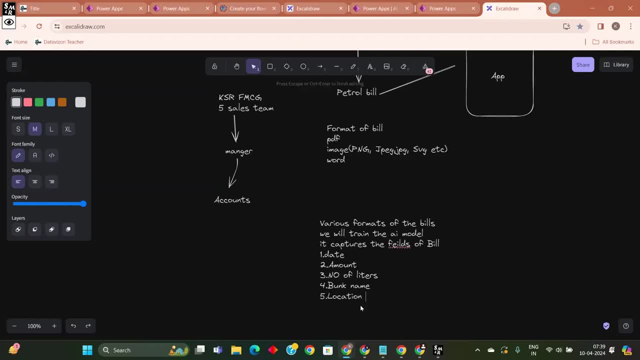 in some code, in some locations it will be 115 120.. be 115 120.. be 115 120.. so they also need to get the location to. so they also need to get the location to. so they also need to get the location to verify whether they are keeping a. 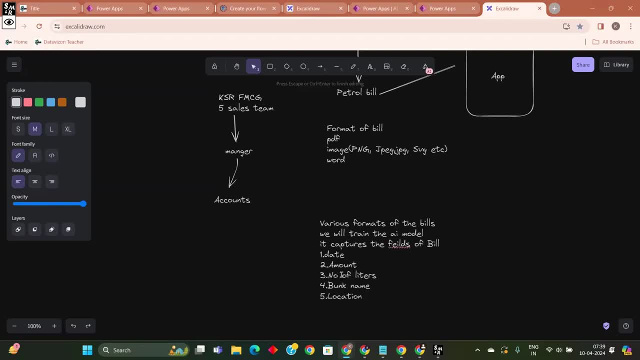 verify whether they are keeping a, verify whether they are keeping a correct bill or not, correct bill or not correct bill or not. okay, these are few fields which we can. okay, these are few fields which we can. okay, these are few fields which we can. and a name, of name of the person also. 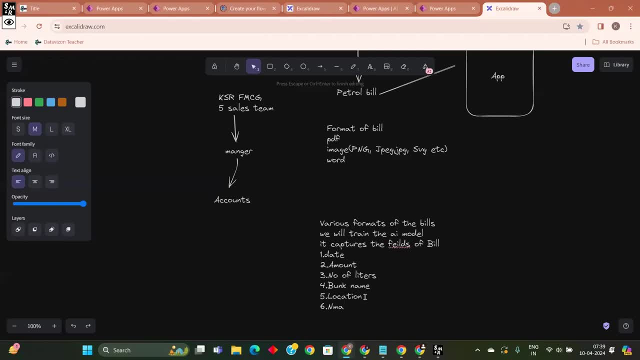 and a name of name of the person also and a name of name of the person also. this is very important. this is very important. this is very important. person name, employee, id, id name and id, person name, employee, id, id name and id person name, employee, id, id name and id name and id name and id also. 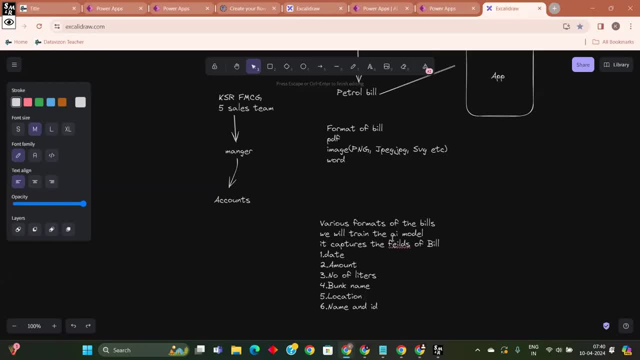 name and id also name and id also okay. so these are the things which are okay. so these are the things which are okay. so these are the things which are mandatory. it should be in the mandatory. it should be in the mandatory. it should be in the uh format of the bill. 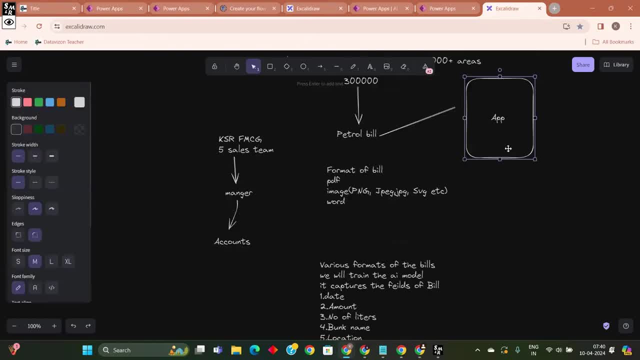 and here we have an option also before, and here we have an option also before. and here we have an option also before: uh ai builder, also we have an option. uh, uh ai builder, also we have an option. uh, uh ai builder, also we have an option. uh, it will, what we, what take, what we can do. 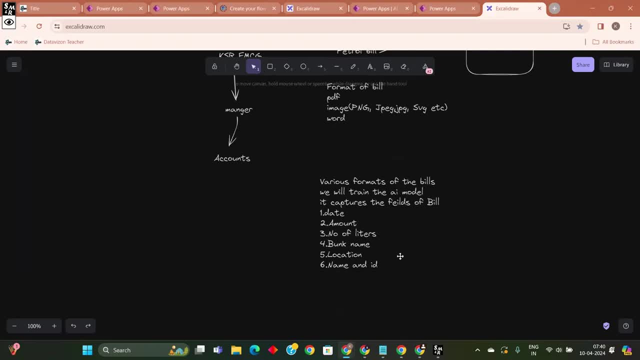 it will what we what take, what we can do. it will what we what take. what we can do is uh, is uh, is uh, we will upload the data. i mean like manually enter the data. and i mean like manually enter the data. and i mean like manually enter the data and we will upload the pdf. i mean like uh. 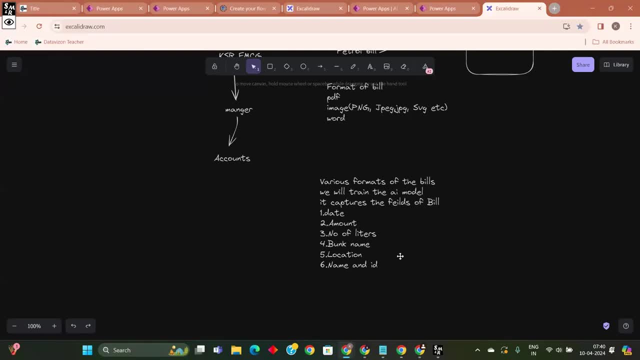 we will upload the pdf. i mean like uh. we will upload the pdf. i mean like uh, bill bill bill image as a proof. this is bill bill bill bill image as a proof. this is bill bill bill bill image as a proof. this is also one option, is there? 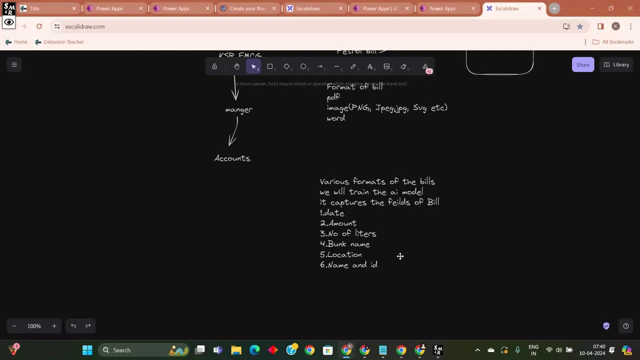 also one option is there also one option is there again here. the problem is that again here. the problem is that again here. the problem is that if you do it manually, if you do it manually, if you do it manually again, account stream should cross check again, account stream should cross check. 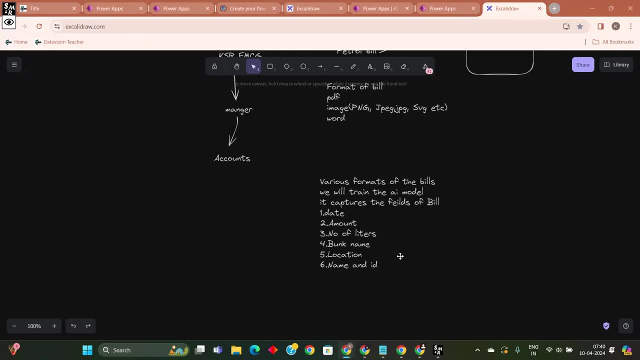 again, account stream should cross check the image, the image, the image and the fields which you have entered and the fields which you have entered and the fields which you have entered. suppose the bill is, suppose the bill is, suppose the bill is costing 1025, costing 1025. 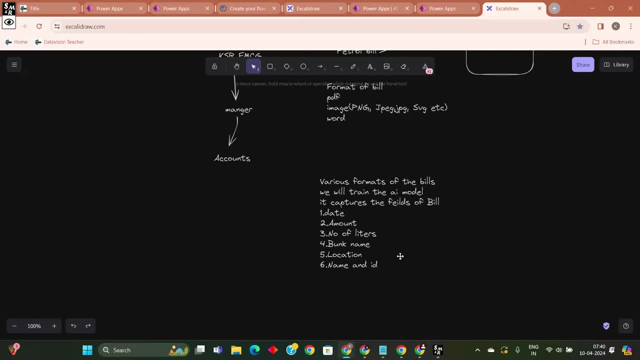 costing 1025 and accounts team want to process. they and accounts team want to process. they and accounts team want to process. they want a proof, want a proof, want a proof. what will happen if they want to prove? what will happen? if they want to prove what will happen, if they want to prove again, they will cross verify the bill. 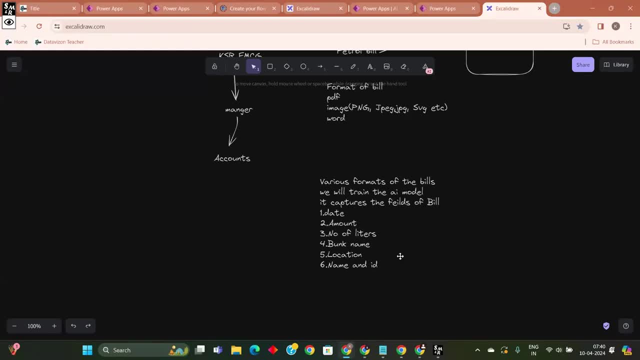 again. they will cross verify the bill again. they will cross verify the bill and they will cross verify the input. and they will cross verify the input and they will cross verify the input fields which you have entered, fields which you have entered, fields which you have entered: 1025 is in the input field and the bill. 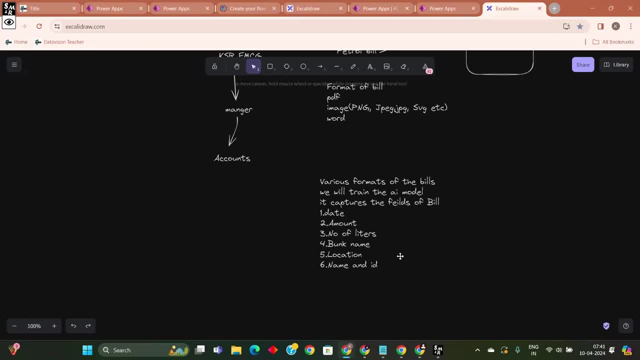 1025 is in the input field and the bill 1025 is in the input field and the bill is showing 1015, is showing 1015, is showing 1015 again. it will be a problem again. it will again. it will be a problem again, it will. 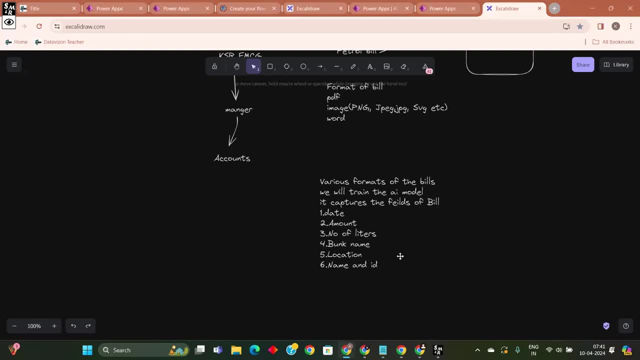 again it will be a problem. again. it will come for uh what we call uh. come for uh what we call uh. come for uh what we call uh- rework. it will be a rework again. they rework. it will be a rework again. they rework. it will be a rework again. they will say that uh mismatch in your bill. 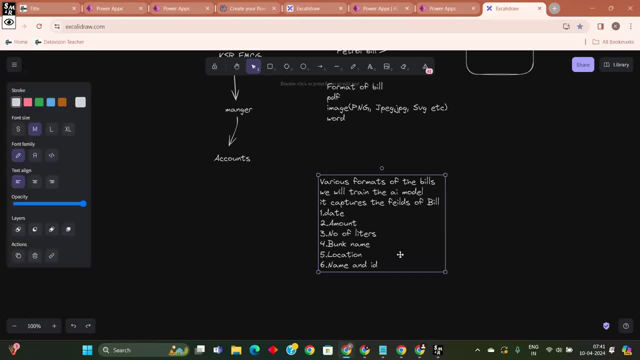 will say that, uh, mismatch in your bill, will say that, uh, mismatch in your bill, please correct returns. and again it will, please correct returns. and again it will please correct returns. and again it will be a time waste. so, what day? what we will do is we will. 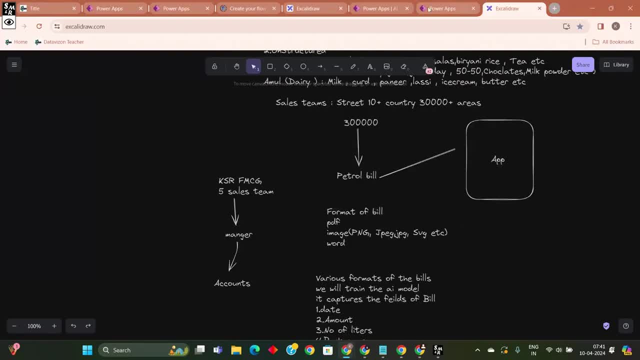 so, what day? what we will do is: we will. so, what day? what we will do is we will train, train, train. uh, we will train the ai model. so this, uh, we will train the ai model. so this, uh, we will train the ai model. so this is a model. 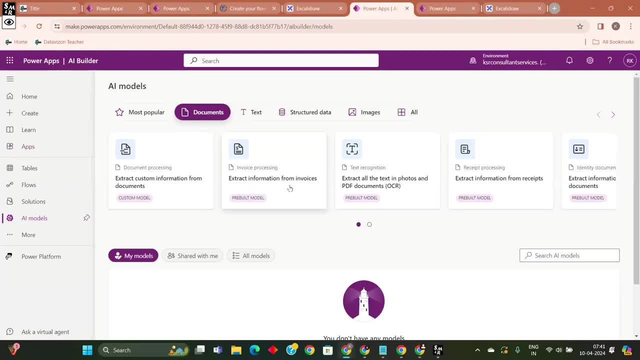 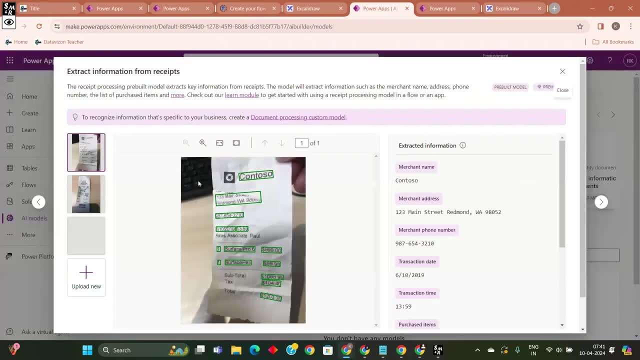 so in uh here. extract information from in uh here. extract information from uh here. extract information from invoices we can take. extract custom invoices we can take. extract custom invoices we can take. extract custom information from documents. information from documents. information from documents. extract information from receipt: extract information from receipt. 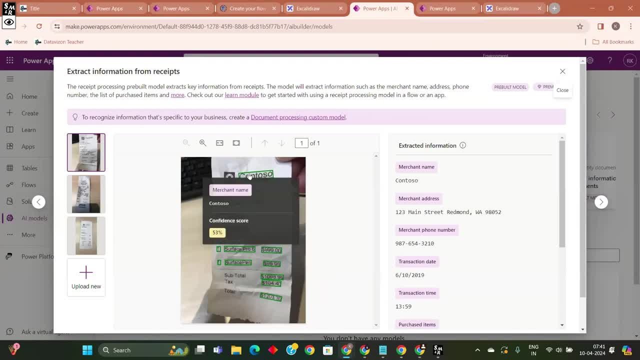 extract information from receipt. so okay, our receipt is in this manner. so okay, our receipt is in this manner. so okay, our receipt is in this manner. so in a bunk, so in a bunk. so in a bunk, we will. we can get a bill directly if we we will. we can get a bill directly if we. 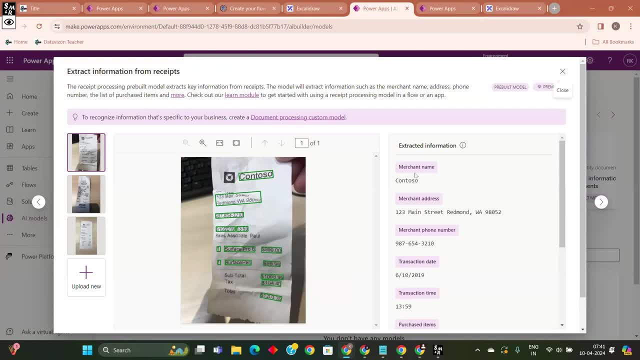 we will. we can get a bill directly if we ask. or else he will directly print the ask, or else he will directly print the ask, or else he will directly print the receipt and view. so a receipt is receipt and view. so a receipt is receipt and view. so a receipt is something which looks like this and an. 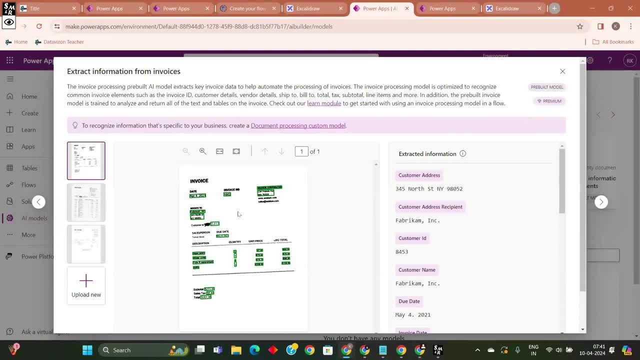 something which looks like this and an something which looks like this and an invoice is something which we which look invoice is something which we which look invoice is something which we which look like this, so probably for a petrol, uh. like this, so probably for a petrol, uh. 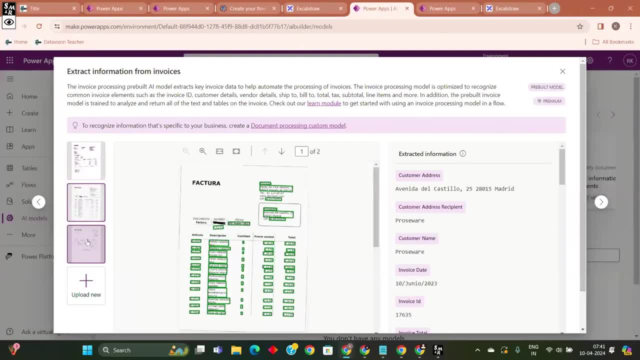 like this. so probably for a petrol- uh, petrol- scenario, we will not get a invoice petrol scenario. we will not get a invoice petrol scenario. we will not get a invoice something like this, okay, something like this, okay, something like this, okay, we'll most probably get a. we'll most probably get a. 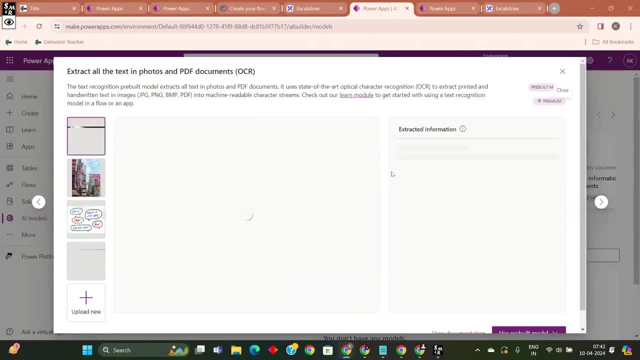 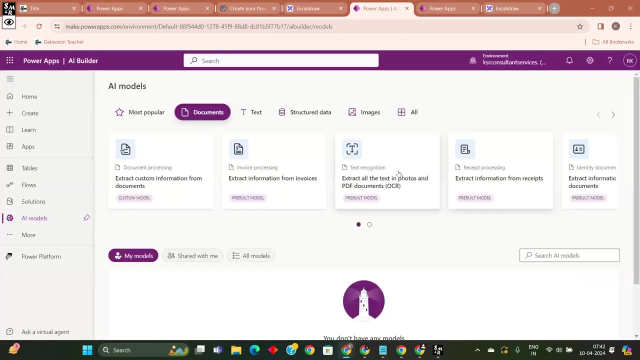 we'll most probably get a invoice in this. uh, we'll probably get a receipt like this, receipt like this, receipt like this: what we will do is uh in a manual. when what we will do is uh in a manual. when what we will do is uh in a manual. when we are developing this ai model, we will 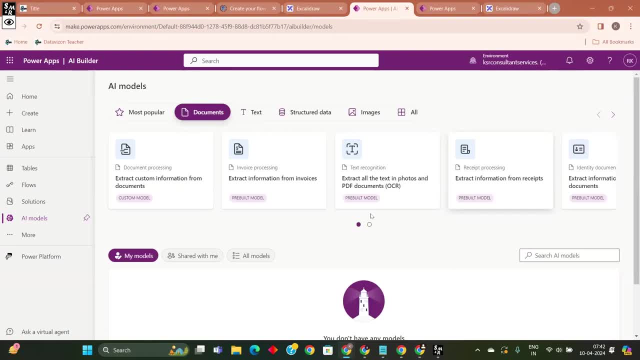 we are developing this ai model. we will. we are developing this ai model. we will collect all the, collect all the collect all the from across the india, what the sales are from across the india, what the sales are from across the india, what the sales are doing, sales people are doing. we will. 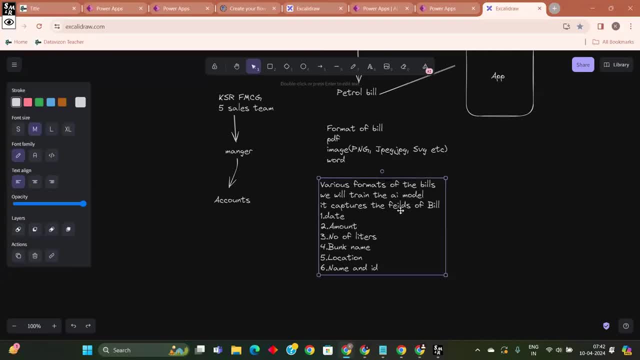 doing sales people are doing. we will doing. sales people are doing. we will gather all these formats from various. gather all these formats from various. gather all these formats from various states, various states of various states, various states of various states, various states of various buildings, various states of various. 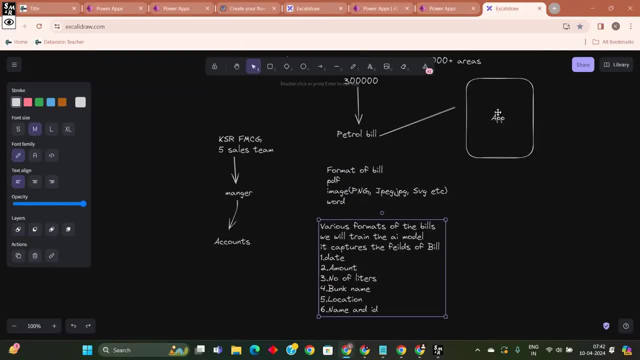 buildings, various states of various buildings, various states of various invoice formats. we will gather all the invoice formats. we will gather all the invoice formats. we will gather all the things and we will train an ai model things and we will train an ai model things and we will train an ai model. so all these formats, what we will do is 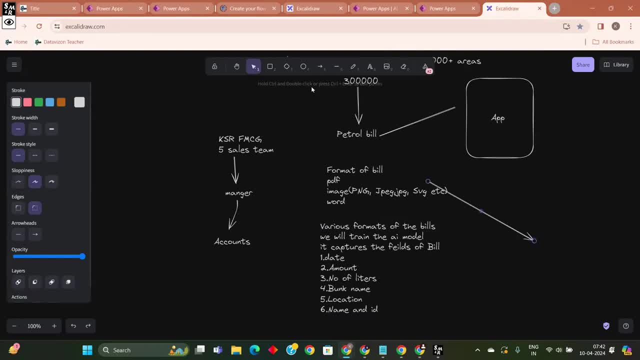 so, all these formats. what we will do is: so, all these formats. what we will do is: for all these formats, what we will do is: for all these formats, what we will do is: we will train a ai model, we will train. we will train a ai model, we will train. 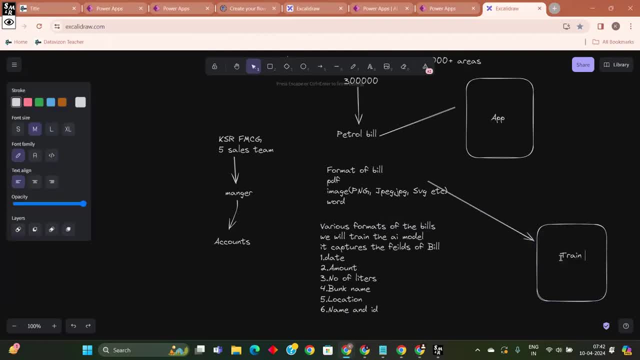 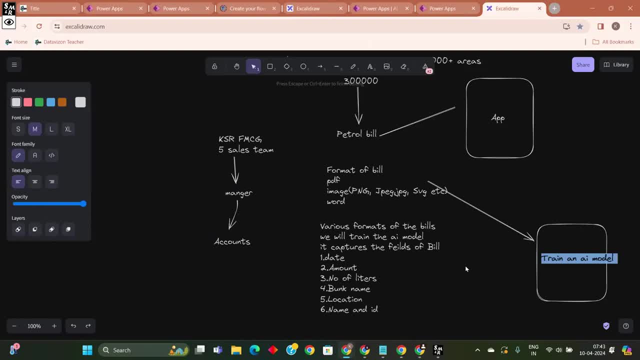 once a model is trained or not, we will train it in such a way that. so, if we will train it in such a way that, so, if we will train it in such a way that, so, if you are training a cricket player, if you, you are training a cricket player, if you. 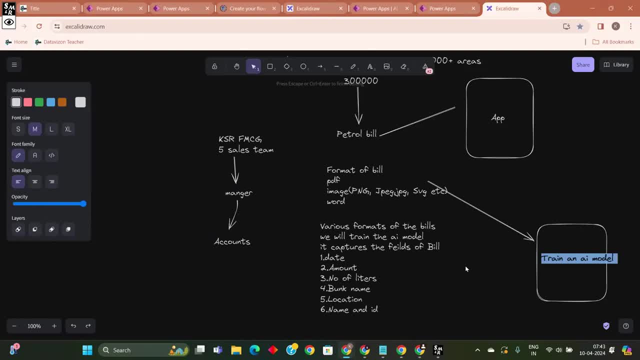 you are training a cricket player. if you are training an all-rounder like hardik, are training an all-rounder like hardik. are training an all-rounder like hardik pandya, so his coach will train him in pandya, so his coach will train him in. 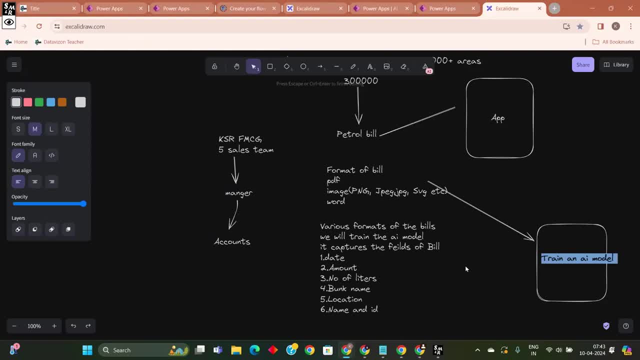 pandya. so his coach will train him in both balling feeling and as well as both balling feeling and as well as both balling feeling and as well as batting. in the same way we will train our batting, in the same way we will train our. 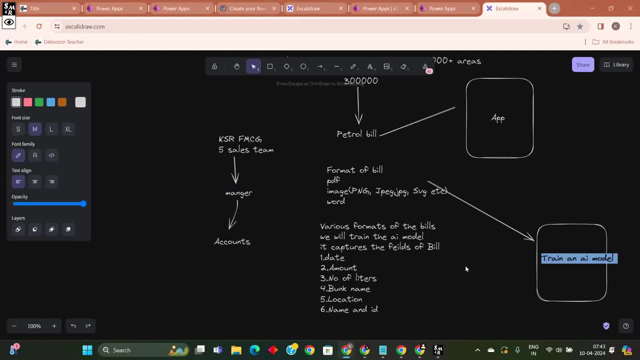 batting. in the same way, we will train our ai model in both structured data with ai model. in both structured data with ai model. in both structured data with unstructured data. no, i will give you the unstructured data. no, i will give you the unstructured data. no, i will give you the concept of structured and unstructured. 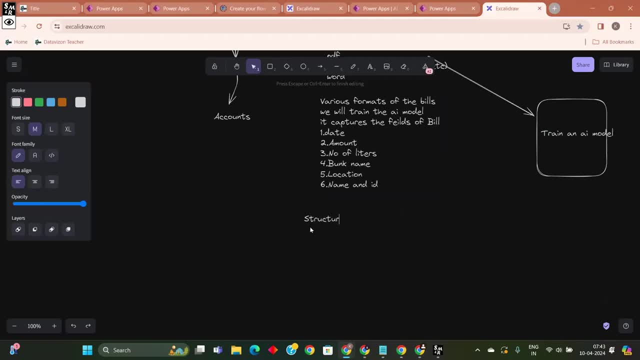 concept of structured and unstructured concept of structured and unstructured data structure. so i will take a same bill as structure. so i will take a same bill as structure. so i will take a same bill as an example. if the bill is always from a. an example if the bill is always from a. 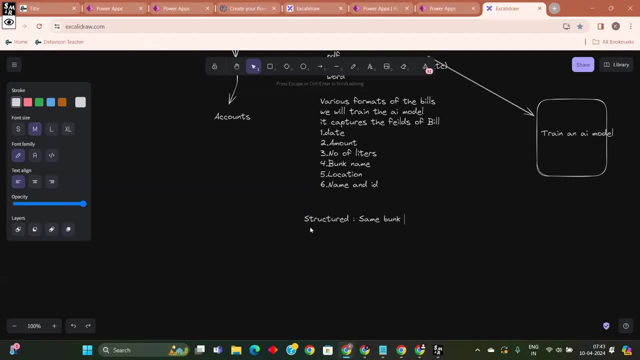 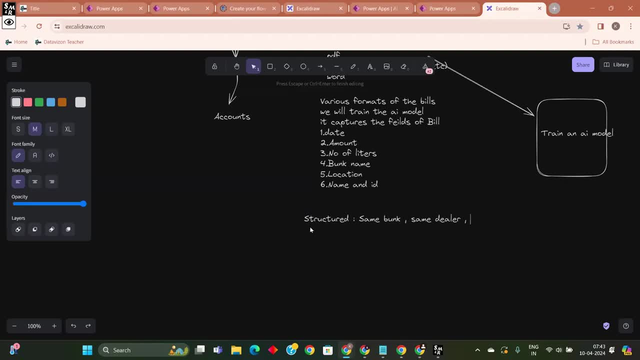 ah means if hp means hp bunk, only if. ah means if hp means hp bunk, only if boris petroleum means boris petroleum. boris petroleum means boris petroleum. boris petroleum means boris petroleum. only indian oil means indian island. this. only indian oil means indian island, this. 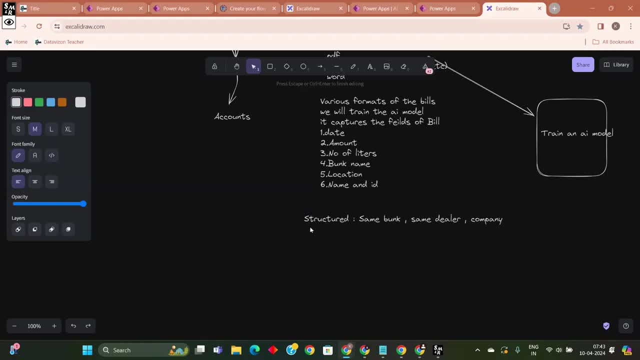 only indian oil means indian island. this is uh when comes to the company, and same bunk means and same bunk means, and same bunk means highly impossible, highly impossible, highly impossible. we said that our sales team is. we said that our sales team is. we said that our sales team is accountable. 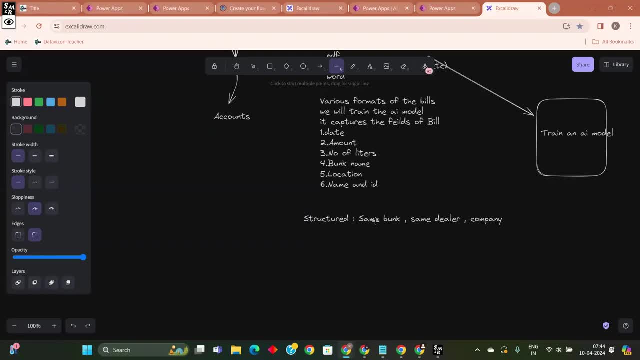 accountable, accountable across india. and same bunk is highly across india. and same bunk is highly across india. and same bunk is highly impossible, impossible, impossible. same bunk is highly impossible correct. same bunk is highly impossible correct. same bunk is highly impossible correct, yes or no? yes or no, yes or no: same dealer possible. 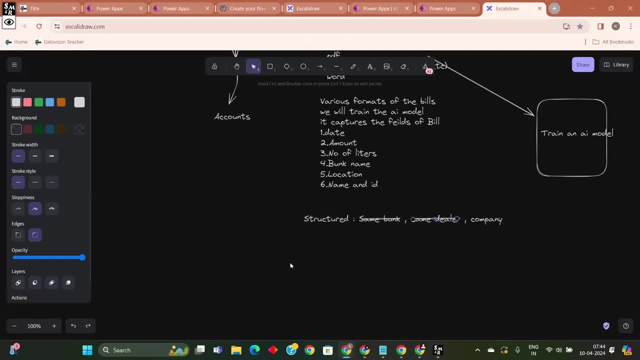 possible or not same dealer. so in possible or not same dealer. so in possible or not same dealer. so in hyderabad the dealer called uh tillu filling store is there in tillu filling store. is there in tillu filling store is there in hyderabad. can we find the same tillu? 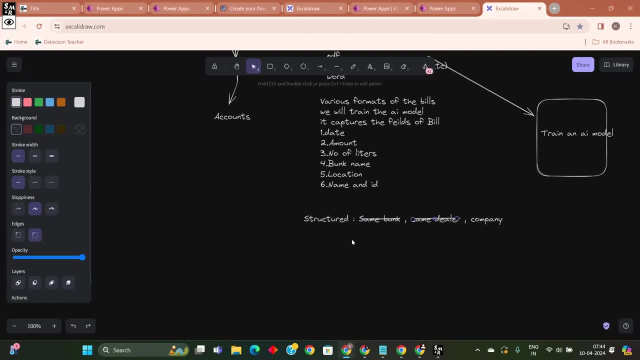 hyderabad. can we find the same tillu hyderabad? can we find the same tillu filling store in pune? filling store in pune. filling store in pune. is that is there a possibility? is that is there a possibility? is that is there a possibility? possibility is there. 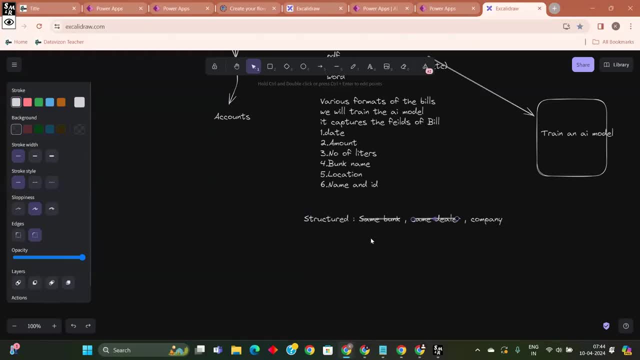 very, very minor possibility. so very, very minor possibility. so very, very minor possibility. so and company and company and company, company, is there a possibility? is there a company? is there a possibility? is there a company? is there a possibility? is there a possibility that all possibility, that all? 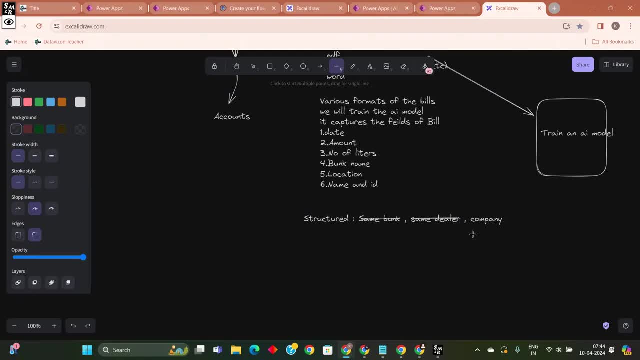 possibility that all because sales team, because sales team, because sales team will do the, will do the, will do the, we'll do the sales. we'll do the sales in cities, we'll do the sales in. we'll do the sales in cities, we'll do the sales in. 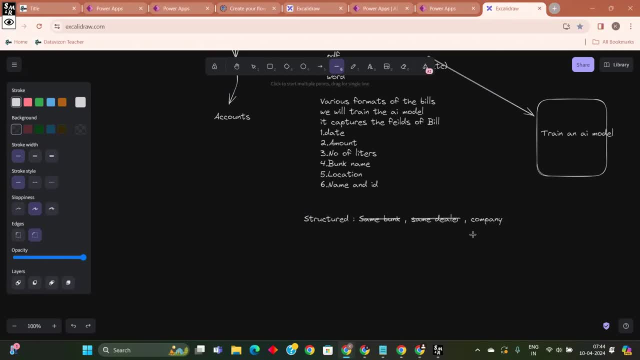 we'll do the sales in villages. we'll do the sales in towns and we'll do villages. we'll do the sales in towns and we'll do villages. we'll do the sales in towns and we'll do the same in a remote areas also. the same in a remote areas also. 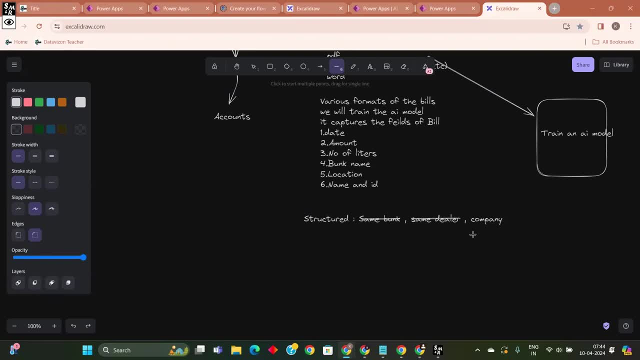 the same in a remote areas also, because if you go to kashi, because if you go to kashi, because if you go to kashi, products correct in those remote areas, products correct in those remote areas, products correct in those remote areas, we cannot expect the same company. no, if 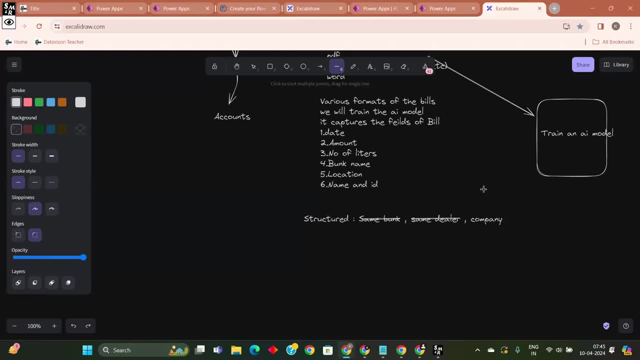 we cannot expect the same company: no. if we cannot expect the same company: no. if some if britannia orders their employees, some if britannia orders their employees, some if britannia orders their employees to fill it from only hb bank: no. to fill it from only hb bank- no. 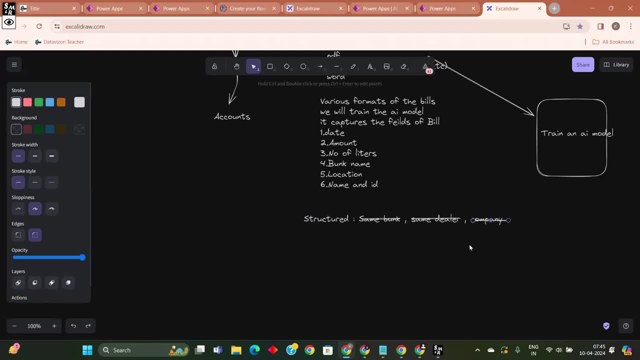 to fill it from only hb bank. no, it is highly impossible that we will find. it is highly impossible that we will find. it is highly impossible that we will find an hb bank in himachal pradesh. uh, an hb bank in himachal pradesh, uh. 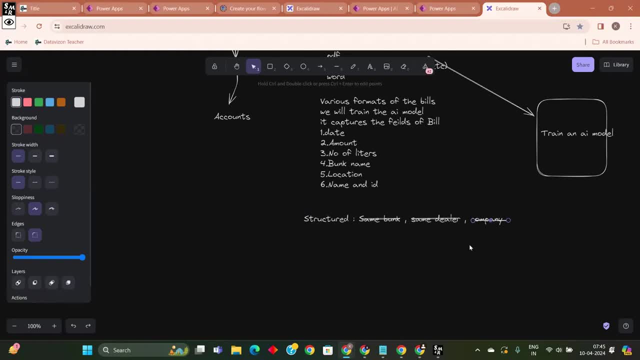 an hb bank in himachal pradesh? uh uh, hilly roads, highly impossible. so, uh, hilly roads highly impossible. so uh, hilly roads, highly impossible. so these three things are cannot be. these three things are cannot be, these three things are cannot be. fees to ksr: uh, ksr, private limited, our. 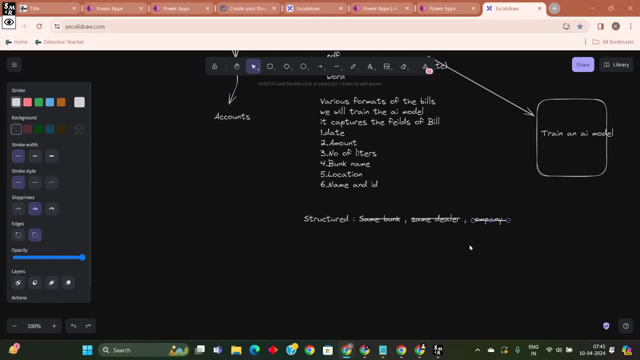 fees to ksr: uh. ksr private limited. our fees to ksr uh. ksr private limited. our company, company, company, hundred person. i can sure that you will hundred person, i can sure that you will hundred person, i can sure that you will all get the same invoices. 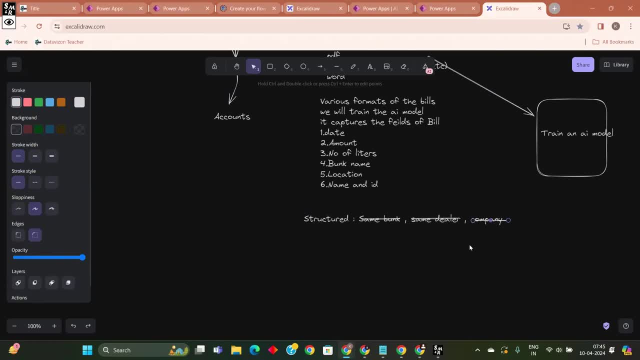 all get the same invoices. all get the same invoices. same invoices. where deadfield is there, same invoices where deadfield is there. same invoices. where deadfield is there, they're only dead will be deadfield. they're only dead will be deadfield. they're only dead will be deadfield. deadfield will be there. 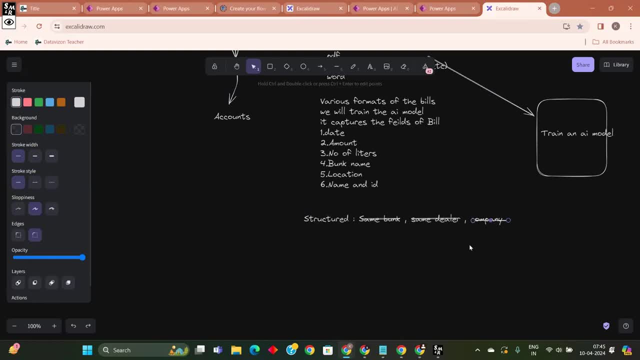 deadfield will be there. deadfield will be there where total billing is there. there only where total billing is there. there only where total billing is there. there only you will get total billing where taxes. you will get total billing where taxes. you will get total billing where taxes are there. there only will find taxes. now. 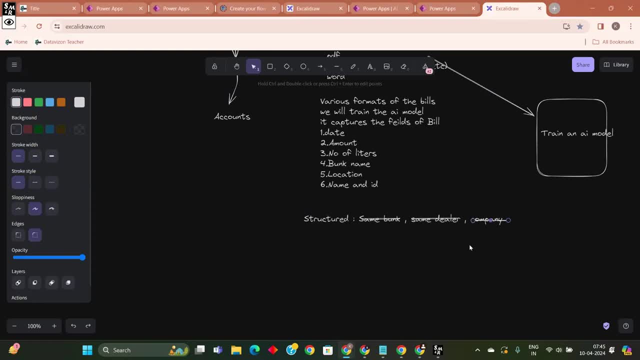 are there? there only will find taxes now. are there? there only will find taxes. now. this is called structured data. this is called structured data. this is called structured data. and you all belong to your same and you all belong to your same and you all belong to your same. you all belong to your say, you are you. 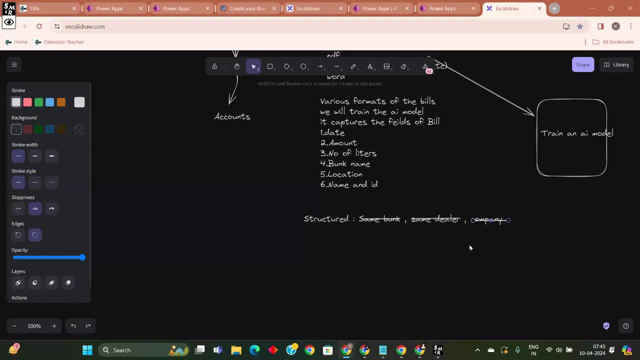 you all belong to your say you are you. you all belong to your say you are. you are all getting your training from the. are all getting your training from the are all getting your training from the same company called ksr private limited. same company called ksr private limited. 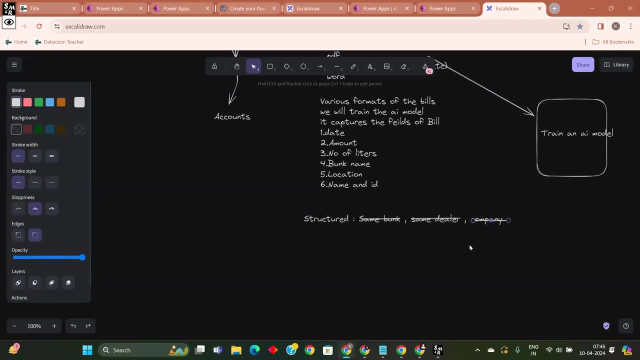 same company called ksr, private limited cancer data division privacy. limited cancer data division privacy. limited cancer data division privacy. limited because you are all in noises will be because you are all in noises will be because you are all in noises will be same. this can i can assure. but 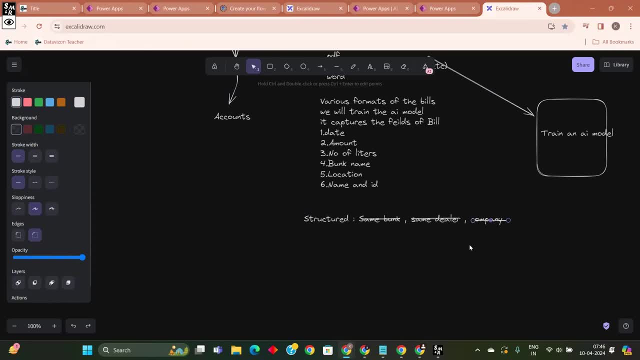 same- this can i can assure. but same this can i can assure. but for a company like vast company, like for a company like vast company, like for a company like vast company like tata britannia and tata britannia and tata britannia and idc, it is highly impossible to get a. 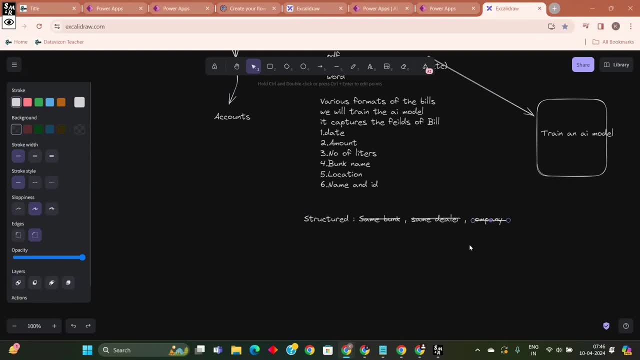 idc. it is highly impossible to get a idc. it is highly impossible to get a structured data now. let's take an example of dominoes. now let's take an example of dominoes. now let's take an example of dominoes. let's take enough dominoes. what dominoes? 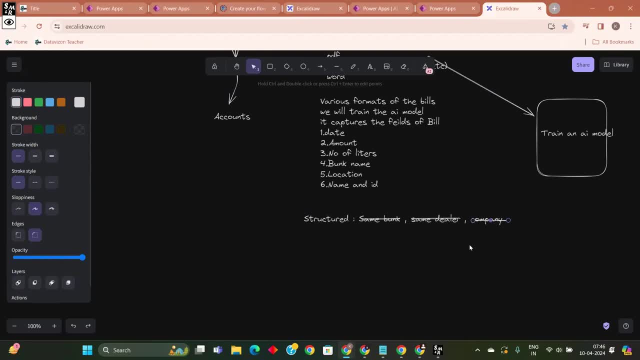 let's take enough dominoes. what dominoes? let's take enough dominoes. what dominoes will do, will do. will do anyone make pizza? make pizza, make pizza? no, they'll just make all the cells. no, they'll just make all the cells. 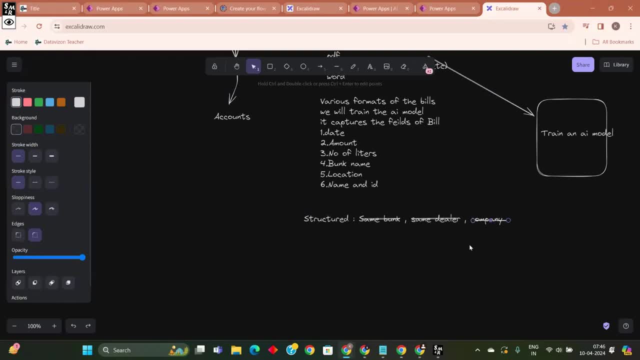 no, they'll just make all the cells pizzas and red pizzas and red pizzas and red. they will make and even sell also. okay, so here uh, so here uh, so here uh, each, see suppose if you are selling something, see suppose if you are selling something, see suppose if you are selling something in delhi. there will be some additional. 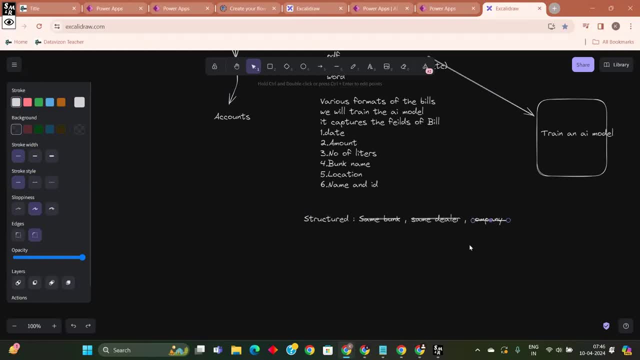 in delhi, there will be some additional. in delhi, there will be some additional taxes, like something called green tax taxes, like something called green tax taxes, like something called green tax. the same green tax is not applicable in the same green tax is not applicable in the same green tax is not applicable in himachal pradesh or hyderabad. 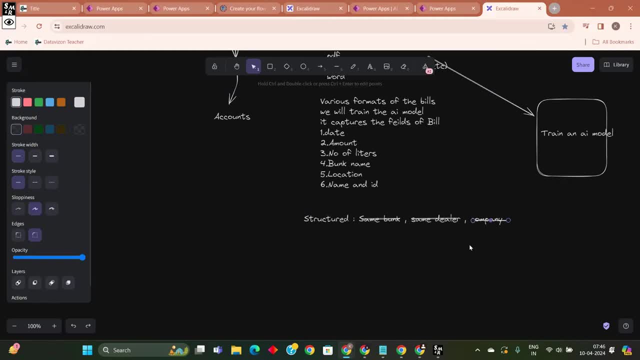 himachal pradesh or hyderabad. himachal pradesh or hyderabad. so based on the state, the taxes will so based on the state. the taxes will so based on the state, the taxes will vary. the central tax will be same but vary. the central tax will be same, but. 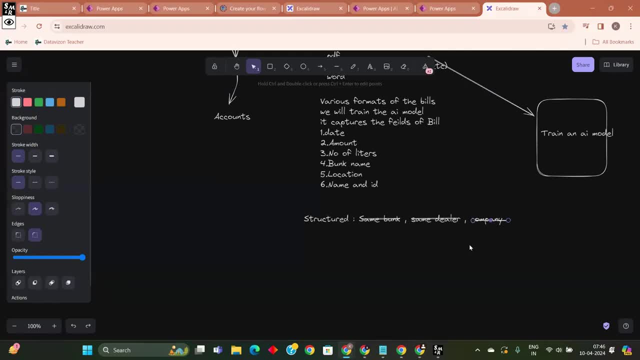 vary. the central tax will be same, but based on the state. there will be based on the state. there will be based on the state. there will be something called some additional taxes, something called some additional taxes, something called some additional taxes. there will be some, there will be some. 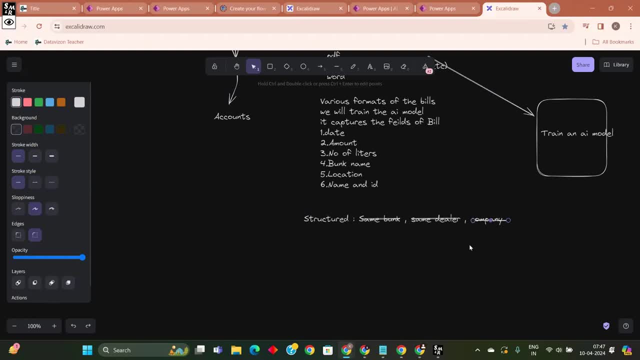 there will be some clean, clean tax. clean, clean tax, clean, clean tax. bmc: we have bmc. we have bmc. we have for bmc. the taxes are high for bmc. the taxes are high for bmc. the taxes are high because it is it need to accommodate bmc. 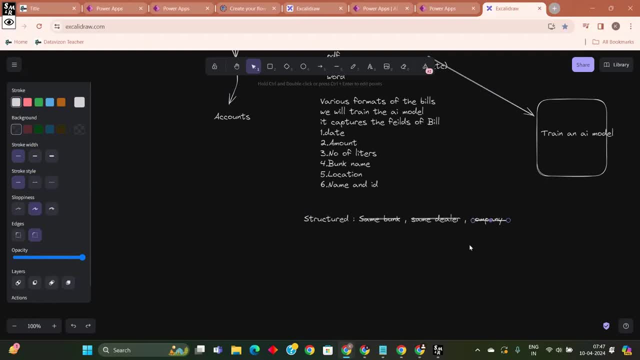 because it is it need to accommodate bmc. because it is it need to accommodate bmc means bangalore, means bangalore, means bangalore, bangalore municipal corporation, bangalore municipal corporation, bangalore municipal corporation. the taxes are high compared to other. the taxes are high compared to other. the taxes are high compared to other other states, other states, other states. because? because, because it need to accommodate more people. it, it need to accommodate more people. it it need to accommodate more people. it need to get more water from other other, need to get more water from other other. 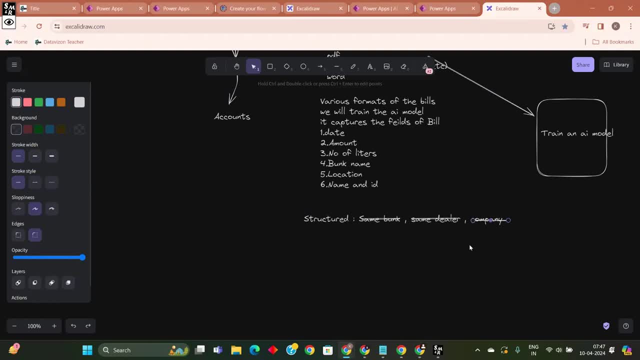 need to get more water from other other areas. so the cost for municipality will areas, so the cost for municipality will areas, so the cost for municipality will be higher, be higher, be higher. keeping all these, all this in uh, keeping all these, all this in uh, keeping all these, all this in uh picture they will design the taxes also. 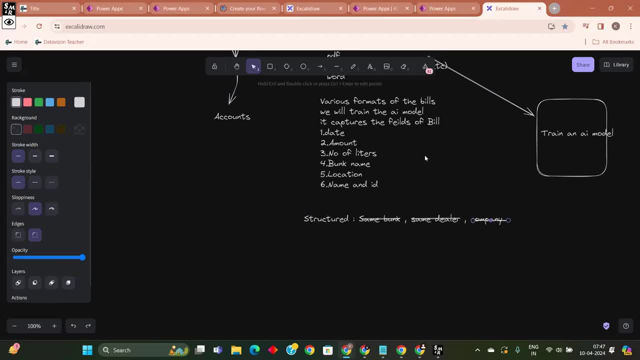 picture they will design the taxes also. picture they will design the taxes also in this way, in this way, in this way, for, even though it is a dominoes, it is for, even though it is a dominoes, it is for, even though it is a dominoes, it is all it is selling. uh, it is from, it is. 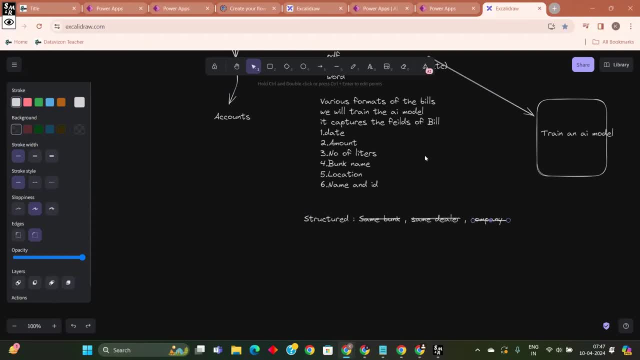 all it is selling, uh, it is from. it is all it is selling, uh, it is from. it is the same franchise franchise chain and the same franchise franchise chain and the same franchise franchise chain. and it is a, it is a, it is a. it is selling the same goods in all its uh. 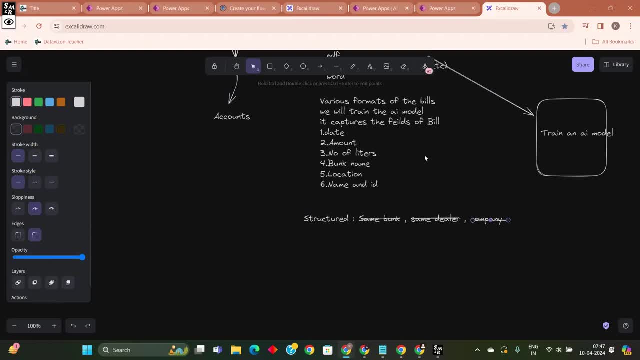 it is selling the same goods in all its uh. it is selling the same goods in all its uh, all its stores, all its stores, all its stores, even though their invoice format is same. even though their invoice format is same, even though their invoice format is same, but the invoice fields will be different. 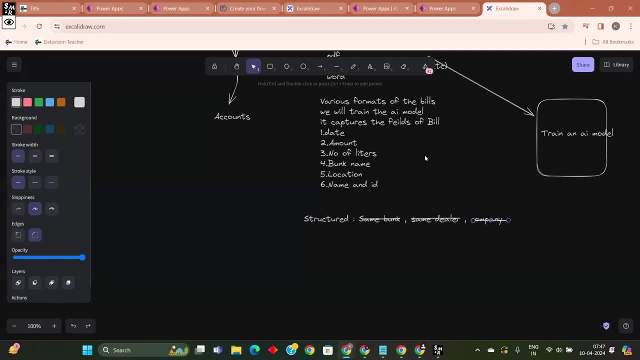 but the invoice fields will be different. but the invoice fields will be different. can you make? can you consider it as a? can you make? can you consider it as a? can you make? can you consider it as a structured data? structured data- structured data- yes or no no? 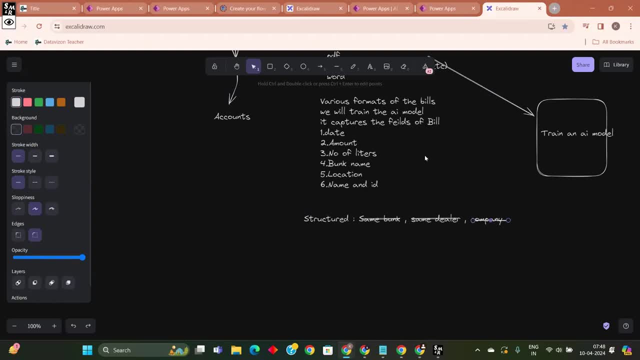 no, no, exactly, no, exactly, no, exactly, no, no. let's see, okay, uh, okay, uh, okay, uh. so so people are thinking that they want so. so people are thinking that they want so. so people are thinking that they want to implement some, uh, to implement some uh, to implement some, uh, some law based on that, every state will 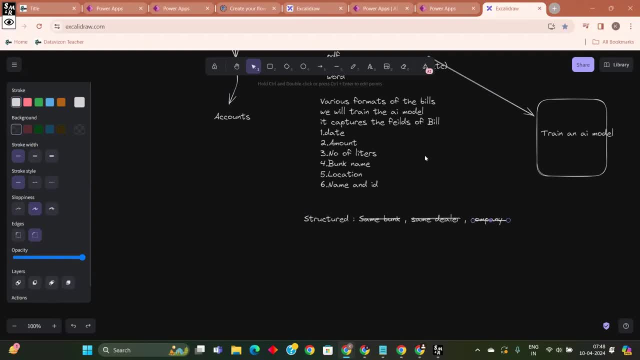 some law based on that. every state will. some law based on that: every state will have same taxes. every, every state will have same taxes. every, every state will have same taxes. every, every state will have same policies, etc, etc. have same policies, etc, etc. have same policies, etc. etc. uh, the bjp government is planning, if that, 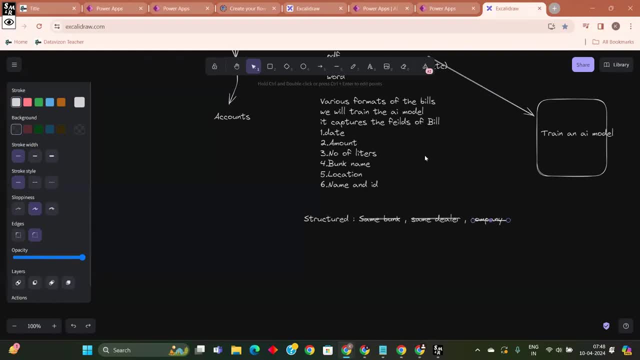 uh, the bjp government is planning. if that, uh, the bjp government is planning. if that also comes into picture. also comes into picture. also comes into picture. no, let's calculate it from. so, domino's, no, let's calculate it from. so, domino's, no, let's calculate it from. so domino's is having a store in india, and domino's. 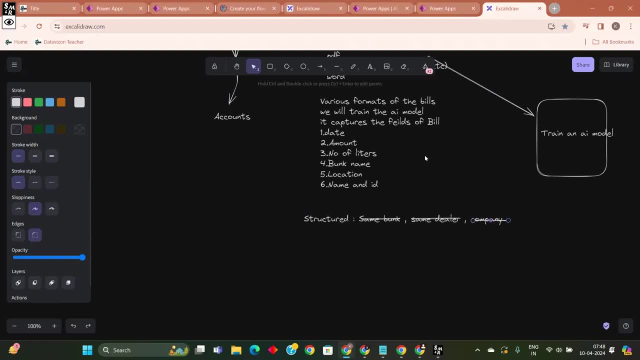 is having a store in india and domino's is having a store in india and domino's is having a store in canada. is having a store in canada. is having a store in canada? no way, both these, no way. both these, no way, both these. the canada taxes on the canada prices. 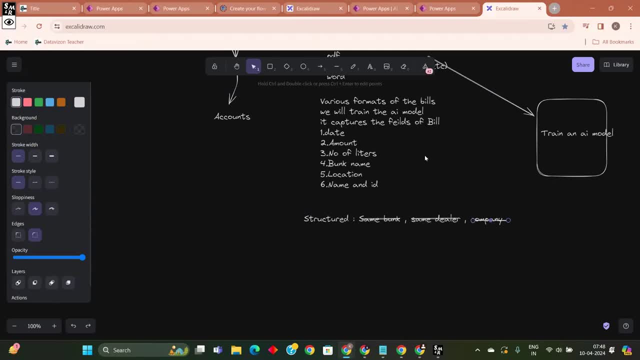 the canada taxes on the canada prices. the canada taxes on the canada prices will be different and the indian taxes will be different and the indian taxes will be different, and the indian taxes and indian prices will be different and indian prices will be different and indian prices will be different. no, they want to submit all these uh. 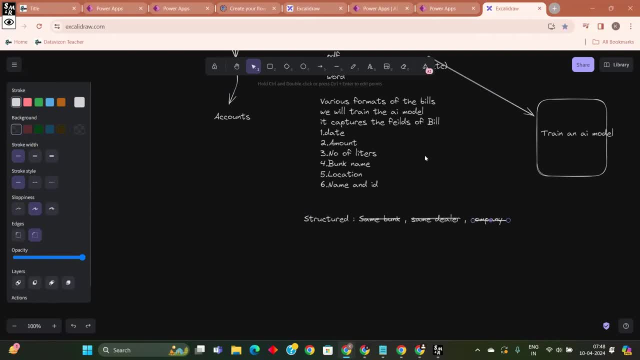 no, they want to submit all these. uh, no, they want to submit all these. uh, what we call a submit all the profits, what we call a submit all the profits, what we call a submit all the profits, are the all the invoices to the central. are the all the invoices to the central? 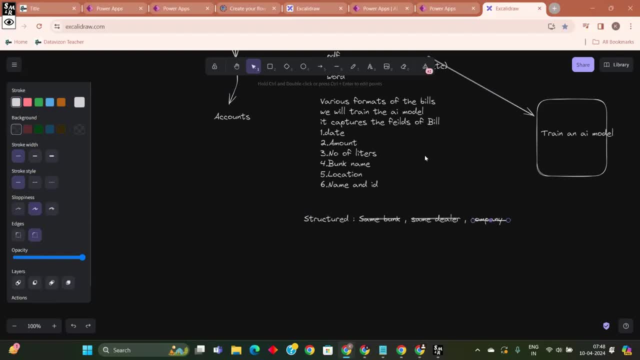 are the all the invoices to the central team, which is in us team, which is in us team, which is in us. there we will get a crash there. we will get a crash there. we will get a crash based on the countries also. based on the countries also. 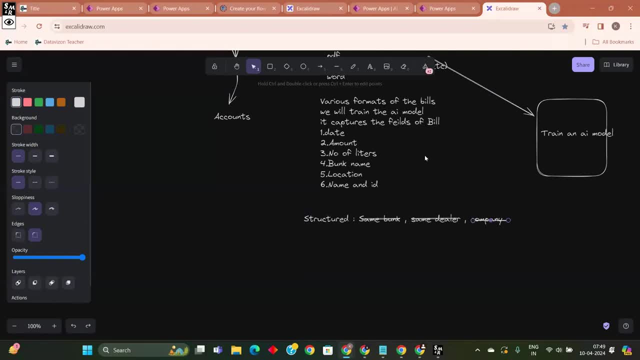 based on the countries. also, if you want to do, do if you want to. if you want to do, do if you want to. if you want to do, do if you want to make. if you want to make an app or make what we. if you want to make an app or make what we. 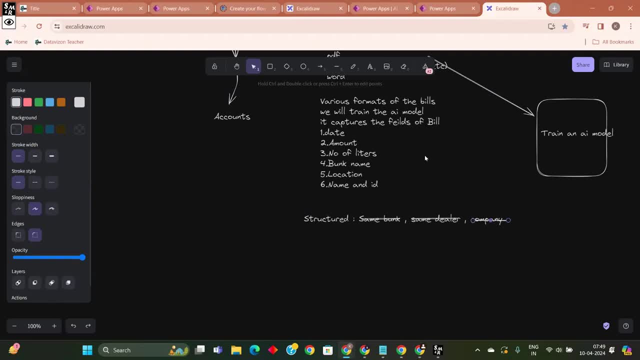 if you want to make an app or make what we call some train a model. uh, structured data is highly impossible. structured data is highly impossible, so structural data is highly impossible. so so this is called unstructured data or unstructured invoices. an unstructured invoice, unstructured data, means format of docs are not same. 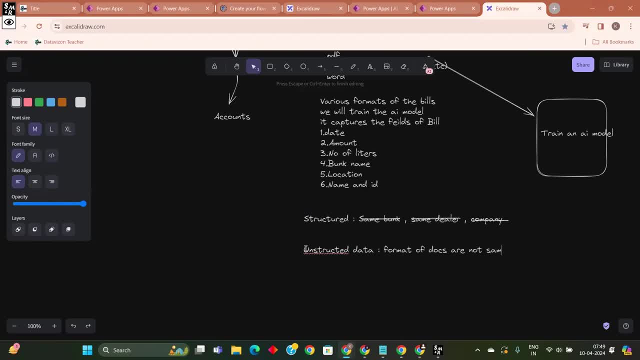 not same here. when it comes to structured data, all the formats and all the fields will be same. okay, so this is a difference between structured data and unstructured data, based on your requirement, most probably in the things which i have worked on now we get unstructured data only, but if you are- uh, if in some use cases, internally suppose, 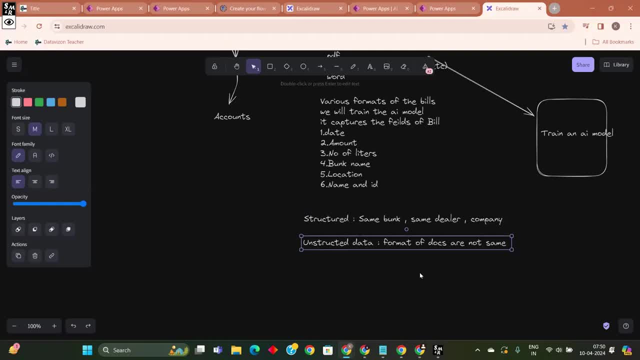 if you want to do and create an ai model for our invoice invoices, our students invoices in ksr, then we will definitely go for structured data. structured data in order to read the information. it will take less time, but it when it comes to unstructured data, your training. 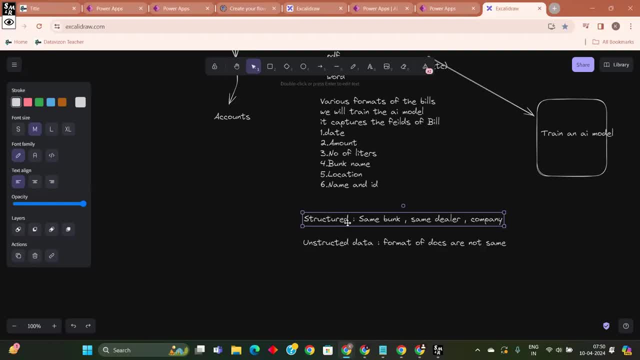 model should also be in a very high. you should train the model in a very high manner. you should also code them accordingly. okay, you need to link the feeds properly here in structured data. it will be a structure data. it will be a structure data. it will be a structure data. 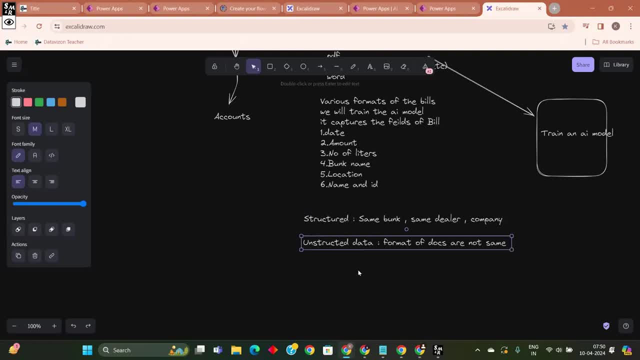 smooth run. when it comes to unstructured data, you need to keep in mind each and every problem which you can face. you need to get all invoices across the world. okay, so dominoes will collect. get the invoices of uh, various stores, various states of various countries, then create a model. 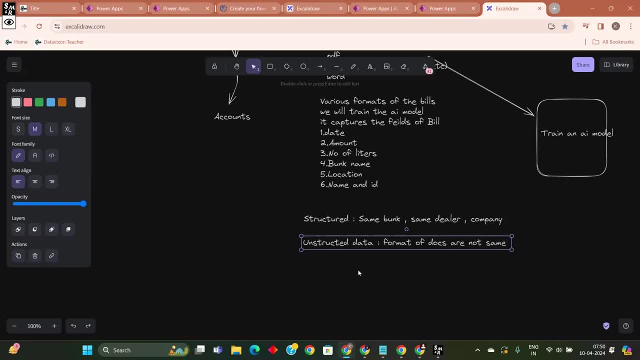 now, this is the difference between structured matter. just remember one thing in ai model: when compared to other tools with the ai model is like a cakewalk, but the thing is that it is a very bit costly tool and you need to know how to use that, which i will teach. main questions in ai builder, which 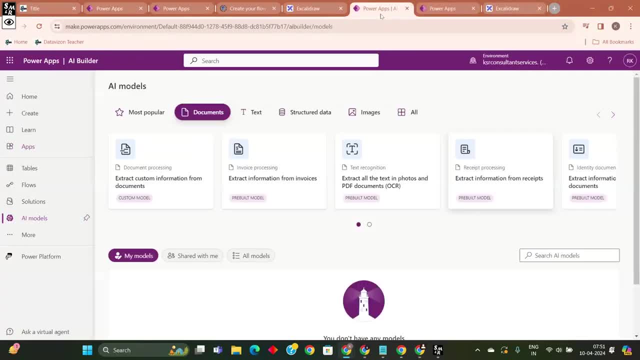 you will get is types of types of ai builders. so, types of ai builders. so firstly you should say: firstly, you should say when someone asks you know, uh, just big, extract custom information from documents, extract information from invoice, extract the text in photos and uh, this is the production model. i will discuss it about this production model no only, and customer feedback. 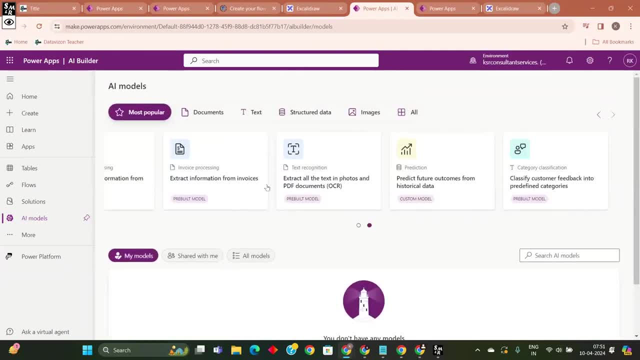 okay, any questions still here? when i started working with ai models, there were only just four models. there were only just four models. but here we have under documents, i have six under text. i have some so many eight under structure that i have one images, i have three. 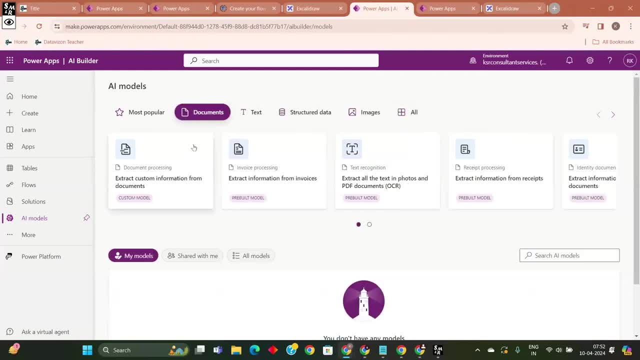 all images when i started working with ai models. i have only document, i have image, i have ocr and i have, uh, this one prediction model. only four models we have. no, they have simplified and simplified for ease of use. they are separately made: a air model for invoice processing, document processing, recipe processing. 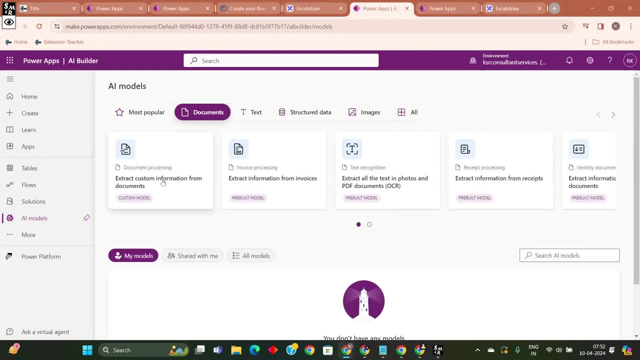 etc. i will give clearly give you information when i directly go to topic and when we are doing hands on. i will give you more information on document processing, invoice processing, recent processing, etc. but for today you understand that if someone asks you questions, how many types of air builders? 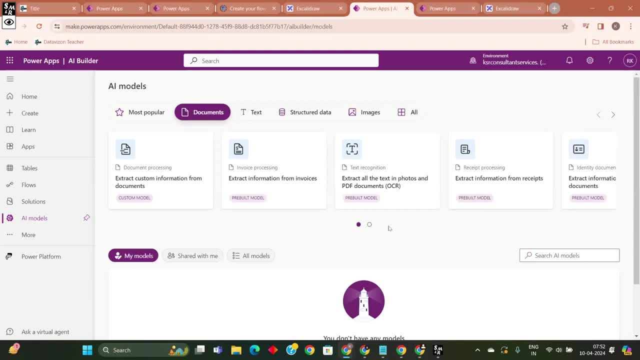 are there in ai models, where models are there in ai builders? you can give these answers, which you can see: document processing, invoice processing, photo processing, recipe processing, uh, id card processing, etc. okay, now let's go. this is one, one use case of ai model. now let's go to. 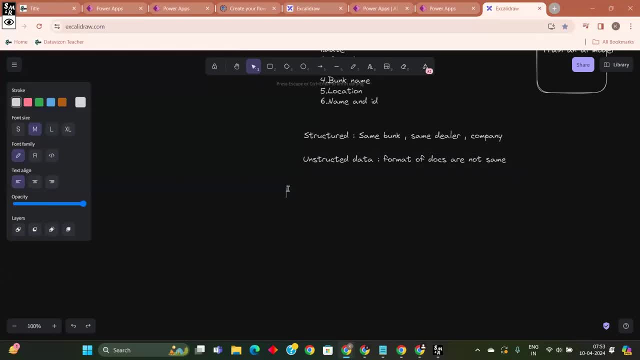 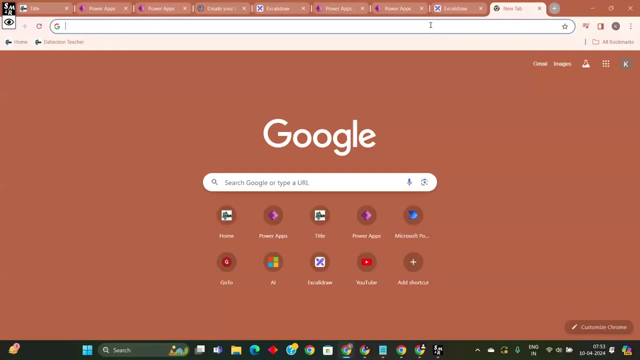 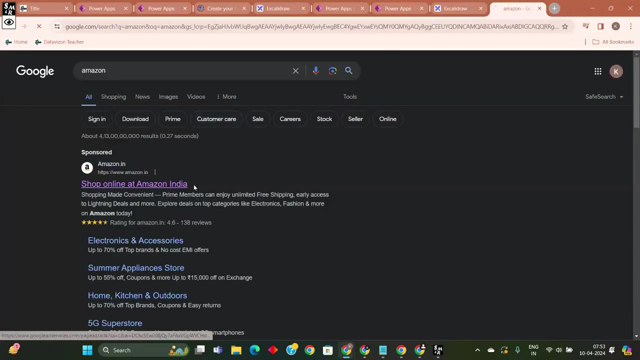 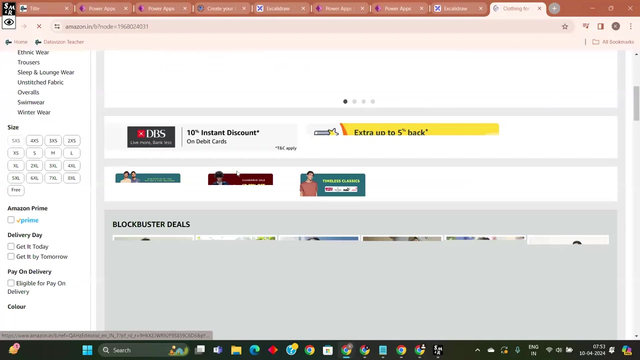 let's go to feedback or analysis, future analysis, prediction model. prediction model. okay, it is very simple to understand when you want to purchase some mobile phone or some product from amazon, which things you will focus. any online model price, apart from that color, color, i agree again. brand. 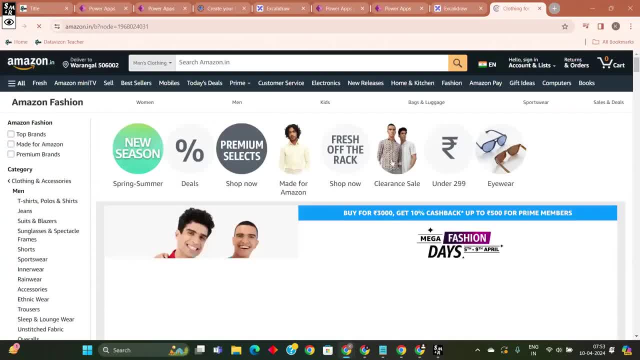 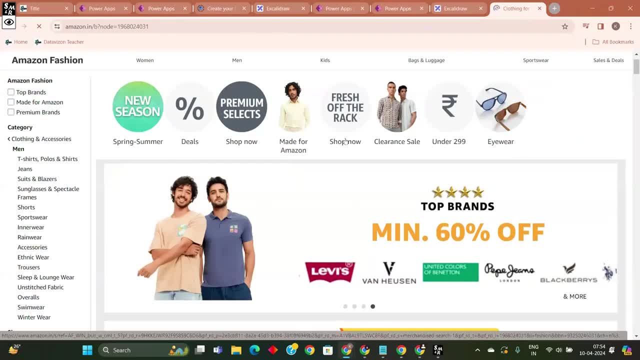 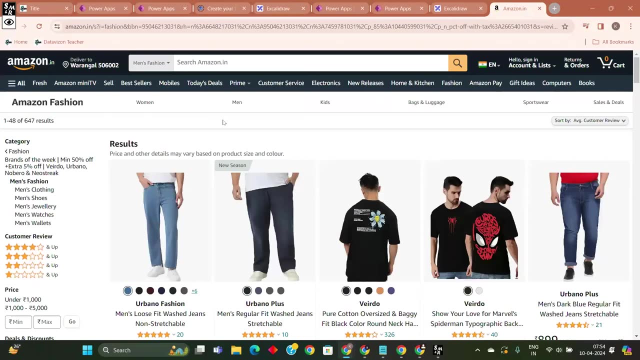 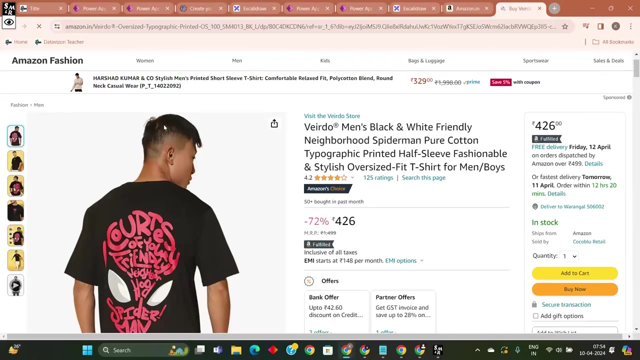 superb, hi size, now all the features which you are saying now from the user perspective of you. no, let's say me. i am the owner, you are only the owner. please put yourself in the owner. okay, okay, please put yourself in the owner. what you will observe, what you will take care. 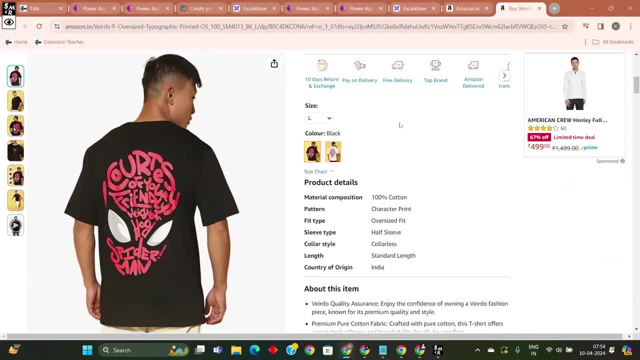 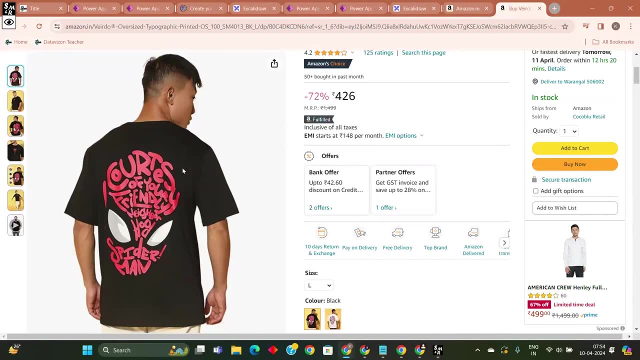 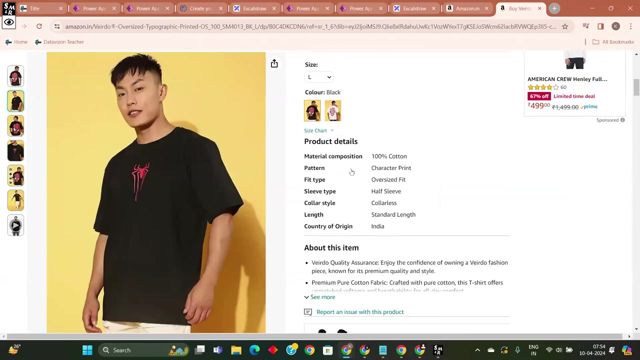 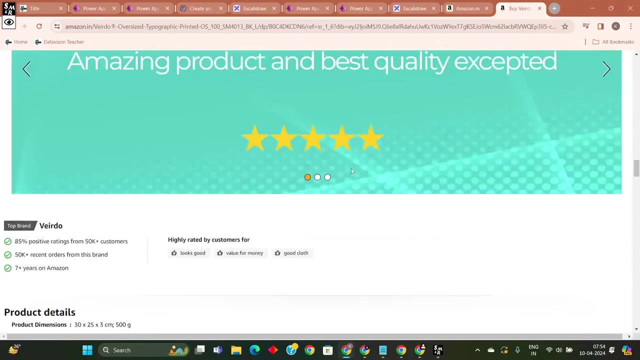 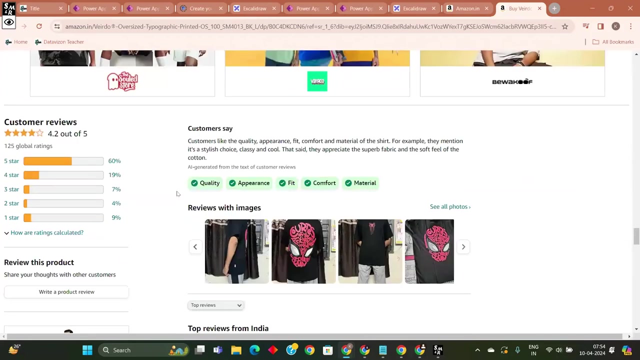 device, not amazon. owner. product owner- much quality and much quality and much quality and lot of on the feedback and rating. as a owner, you will understand whether to reach the customer and give me a new product. so if there will be a lot of customers saying that i received a damaged product, i received a old product, i 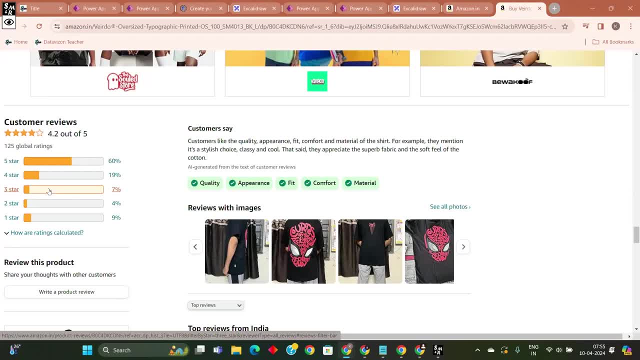 received a user product, especially when it comes to all things, even mobile phones also, there will be like. there will be like some customers saying that there is your user mobile, there is your user t-shirt, there is your user kurta, there is your user salary- sorry, etc. etc. a lot of things will. 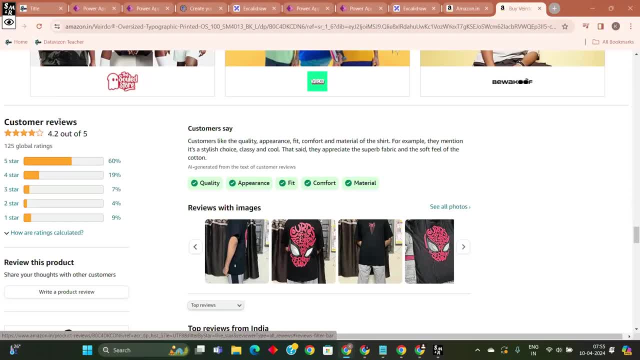 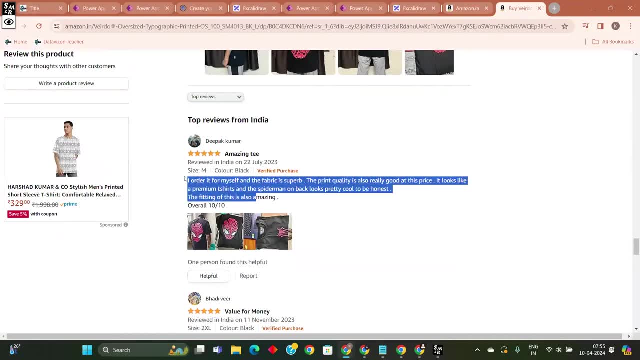 happen now as a business owner, when i go to customer reviews and feedback, then i will come to understand what is happening exactly what is happening exactly now. what we will do is we will take all the comments. we will take the all the comments. so let's see this user's comment deepak. 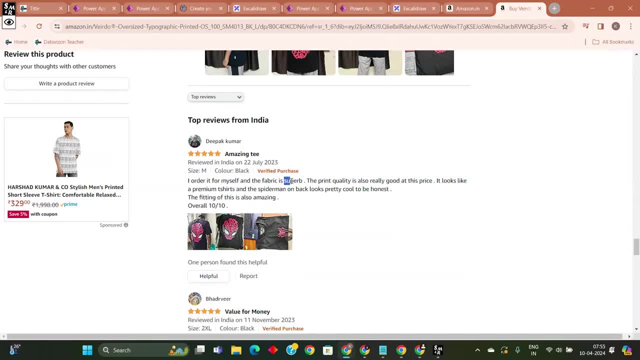 kumar is what deepak kumar is saying inside amazon. he is saying: super, i will mark this word. print quality: i will mark this word. really good, i will mark this word. at this price, pretty call, pretty cool, to be honest. okay, and t-shirt, because here the product is t-shirt. i will mark these words and make that. 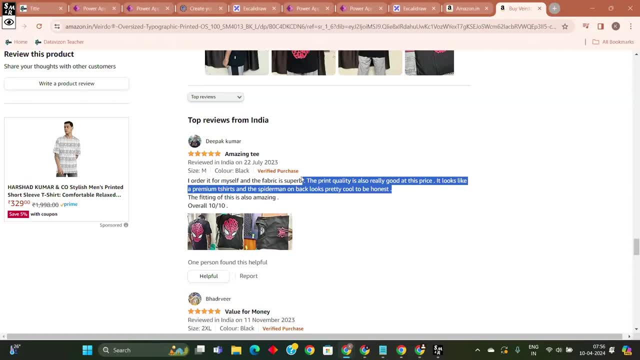 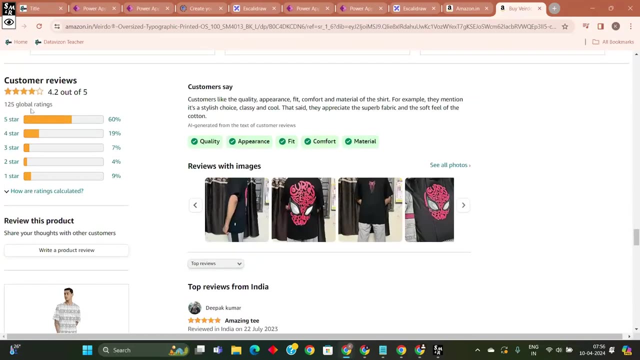 whenever i result, i receive these type of words in any kind of comment. any kind of comment make it as positive production, make it as a positive person. because, as a owner, i cannot come and read daily, uh, nearly 125 ratings, because i'm not only selling this product, this bio code, this is bao nursing company. 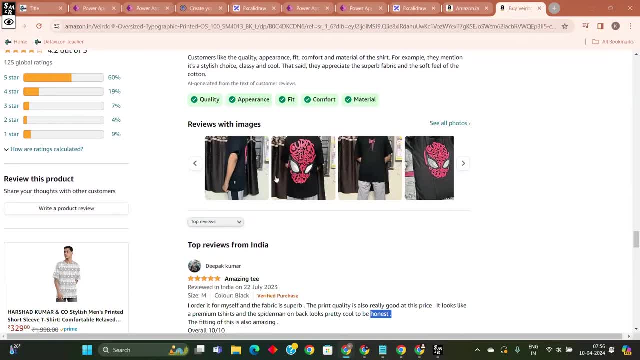 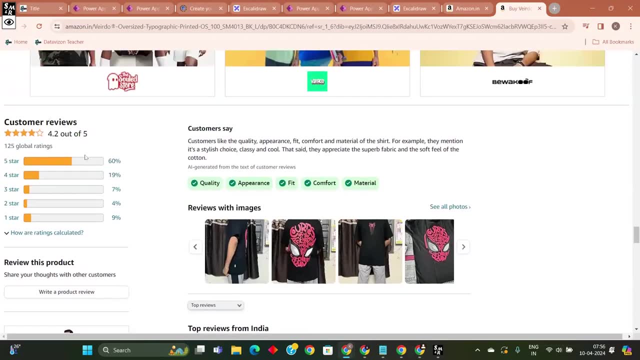 okay, he's not only selling only one T-shirt. he will sell nearly 100 to 200 T-shirts, and for each and every 100 T-shirts. if you want to come and read the ratings, it's highly impossible, so they will use a model which will give them prediction. 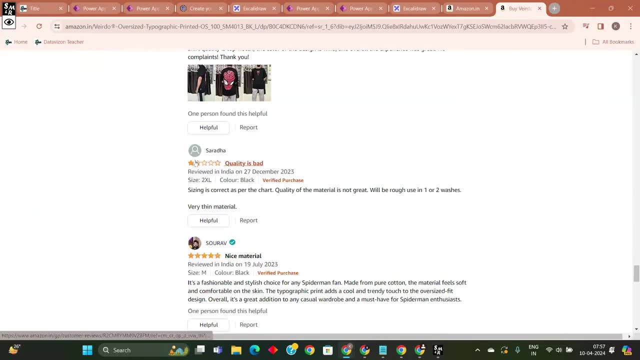 section on feedback. no, here you see, let's go for a negative. connect sizing is correct as per the chart. quality of the material quality. already we have marketed the quality there, that part that guy is saying the quality is good but quality of the material is not great. 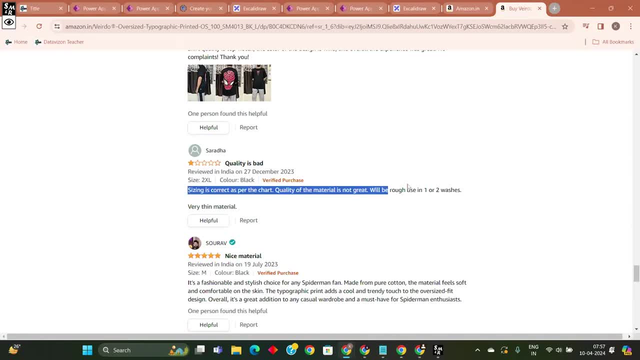 i will use this keyword- will be rough using one to two watches rough and mark this. so i will train the model that if any feedback, if it comes, and if any feedback is containing these kind of terms, treat it as a negative now at the end user. by the day i will have 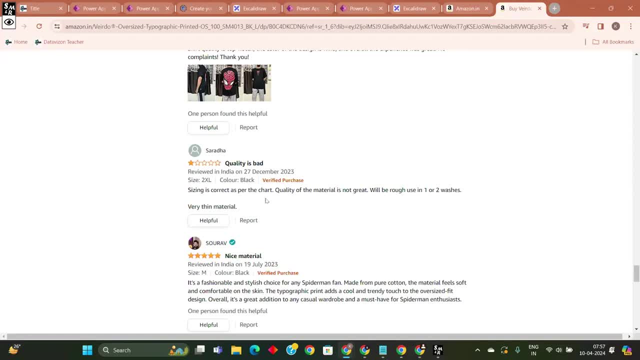 only two columns. the ai model is only filtering all these feedbacks and it will be giving me only two columns to the owner. main order: positive and negative. positive 35, negative: 25. so you will come to understand and it will go to production and it will go to design team and it will ask for the changes. no for the same, for one. 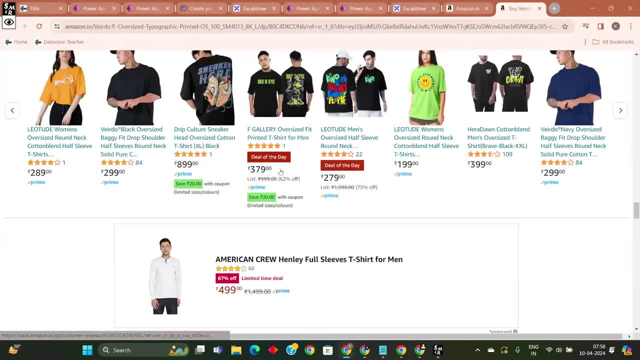 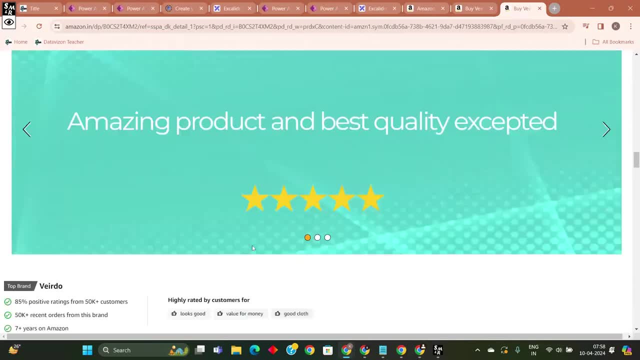 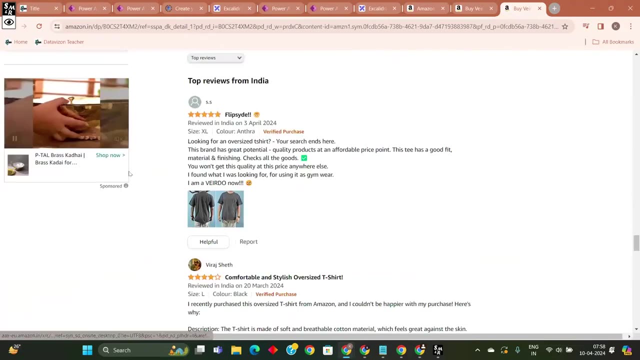 more t-shirt for one more t-shirt, for one more t-shirt. if you use it, you will reverse the process. you will be wondering by your product price. help this product and we. we have also created an ai model for this and it is having 3.9 rating. 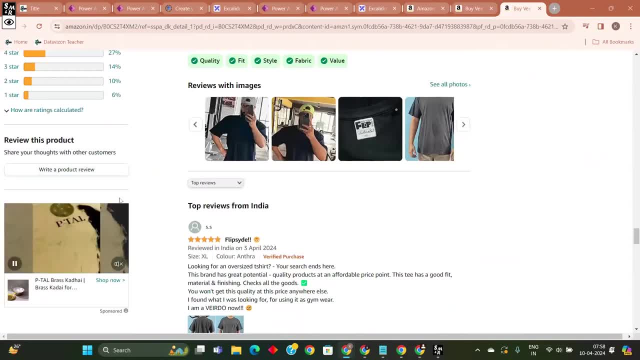 okay, so we will take it. and here the positive are 35 and negative are five. he will not even take care of the product. also, where the negative cases are high, as a product owner, i will come into the picture and look it with legend to my design team, looking to my whatever it is. 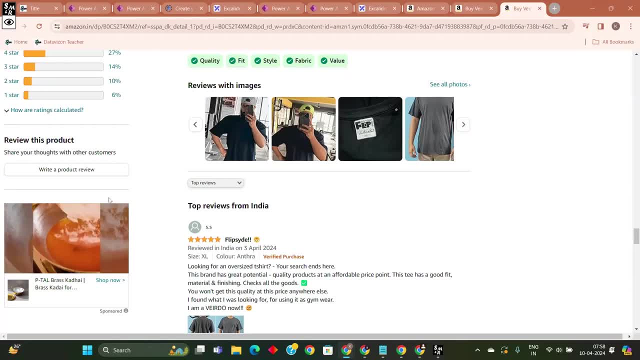 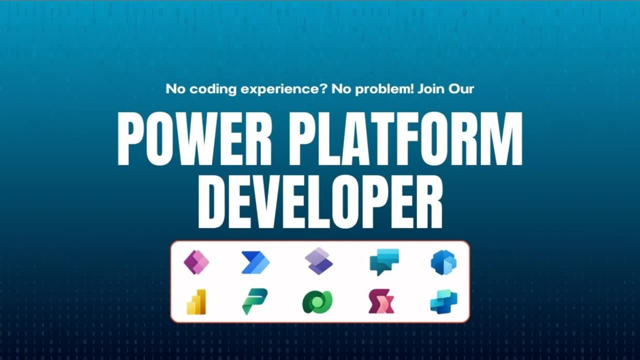 production team. so this is a production model. any questions still here? these kind of developments which we have, which we will do, uh, in ai model. so this is the thing which i have didn't cover in our first five sessions. that is the reason i have covered it today. so people who joined new 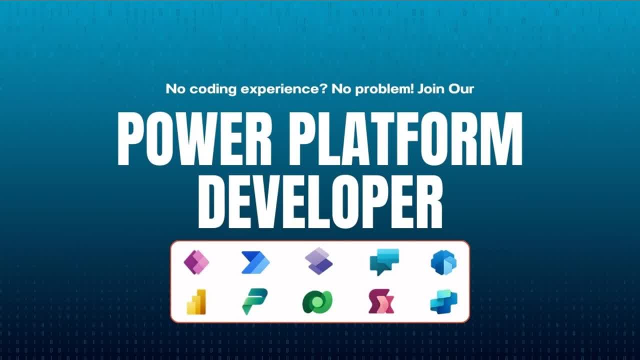 i request you to go through. uh, i would like to stop the session here. people who attended today: they can clarify the questions, along with the people, uh, who are attending daily. uh, i will take the questions from the people who are attending regularly. if you have any questions, you can ask. 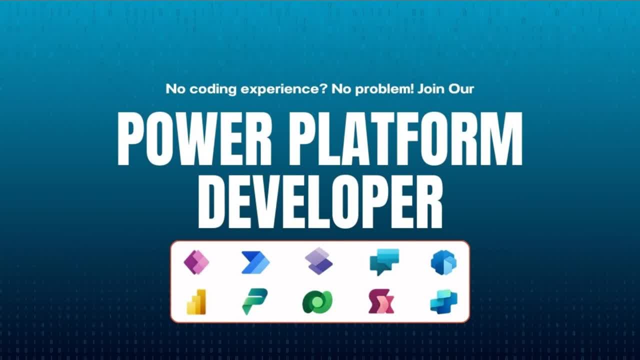 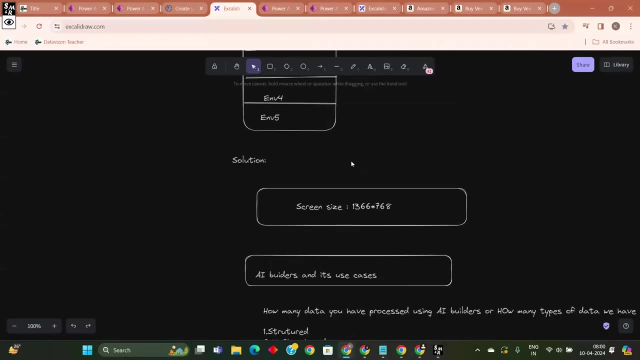 i would like to stop the session here from our regular class. yes, yesterday you told that on environment and solution, that you will tell about manage and unmanaged portion, about this, good ranjini, thanks very much. so here we have managed solution and unmanaged solution. okay, 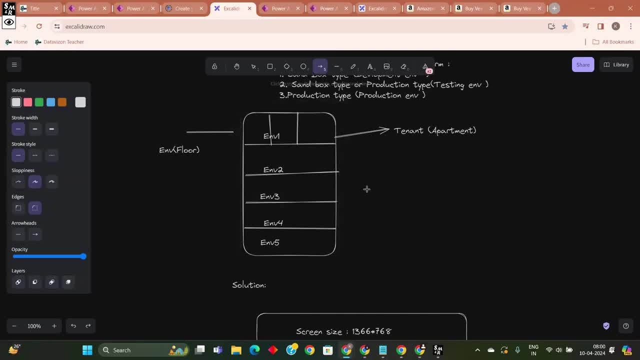 so solutions are of two types and very, very important. uh, interview question. solutions are our two types. one is managed solution- unmanaged comes first, unmanaged, unmanaged. and another thing is managed. you understood how to import and export correct. you understood how to import and export correct. 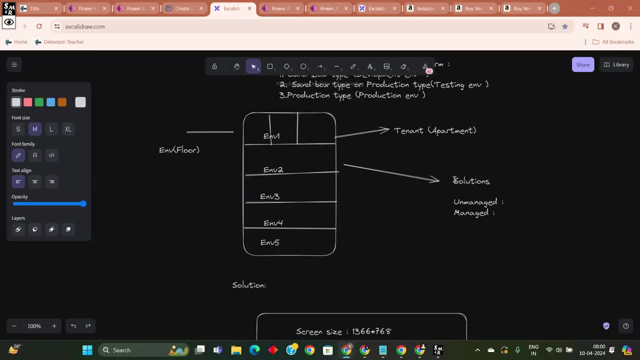 you understood how to import and export correct. you can export and import solutions correct. you can export and import solutions correct. you can export and import solutions correct, yes or no? yes, exactly, but when. to do it as. yes or no? yes, exactly, but when to do it as. 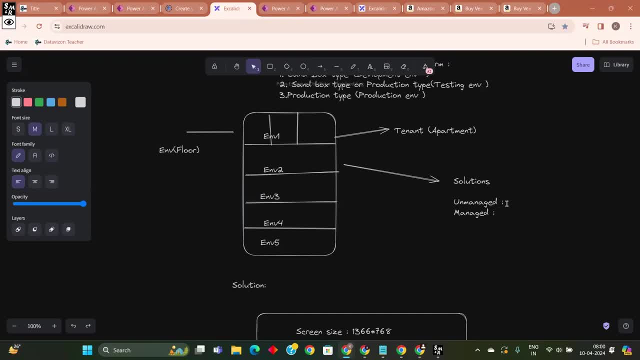 yes or no? yes, exactly, but when. to do it as unmanaged and when to do it as managed- i unmanaged. and when to do it as managed, i unmanaged. and when to do it as managed, i will give a clarity. so when you are will give a clarity. so when you are. 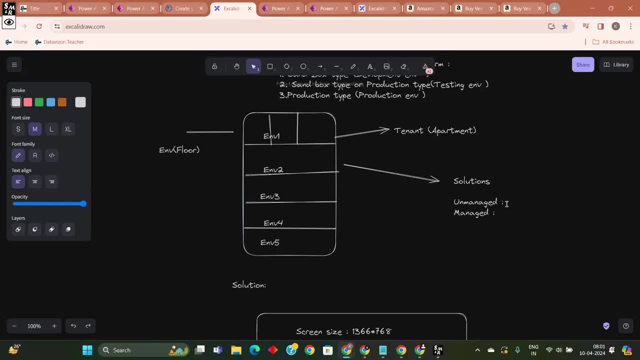 will give a clarity. so, when you are creating a new solution for development, creating a new solution for development, creating a new solution for development purpose for development purpose, purpose for development purpose, purpose for development purpose, are doing changes, are doing changes? are doing changes or enhances or enhances? 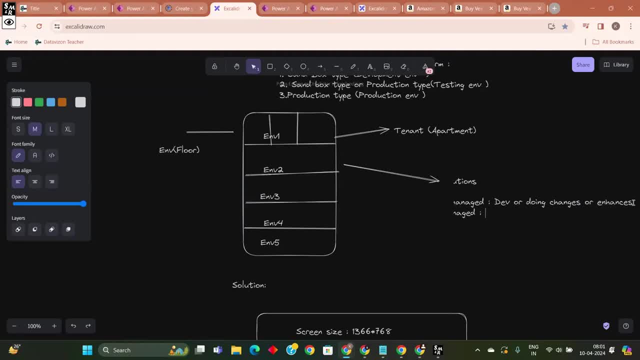 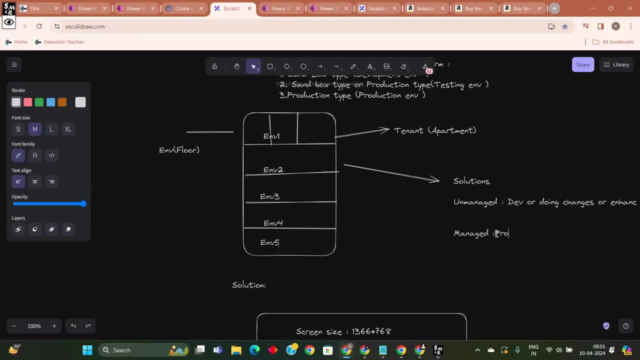 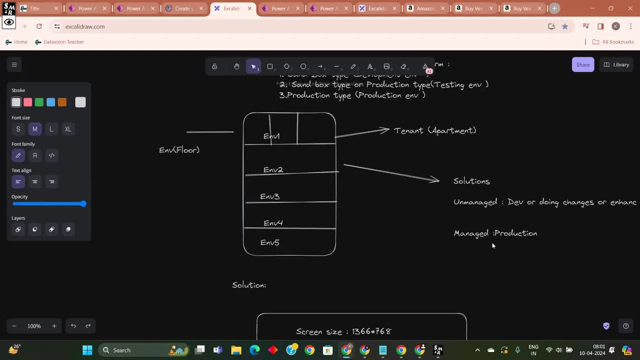 then give it to production, because the then give it to production, because the production version is always live. this production version is always live. this production version is always live. this is the one which is used by various users, is the one which is used by various users, is the one which is used by various users, but when it, when it comes to developer. 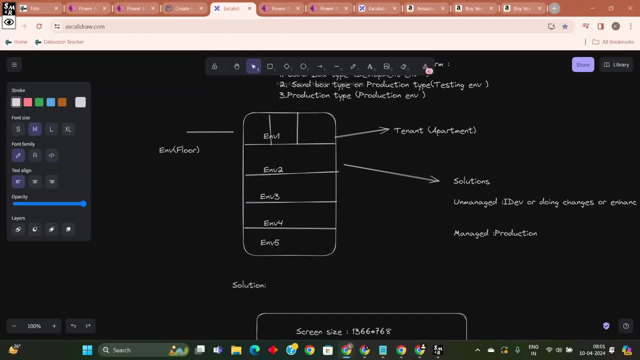 but when it, when it comes to developer, but when it, when it comes to developer environment, no, it will be used. or environment, no, it will be used. or environment, no, it will be used or developed by only developers, only developers, correct, but in when it. only developers, correct, but in when it. 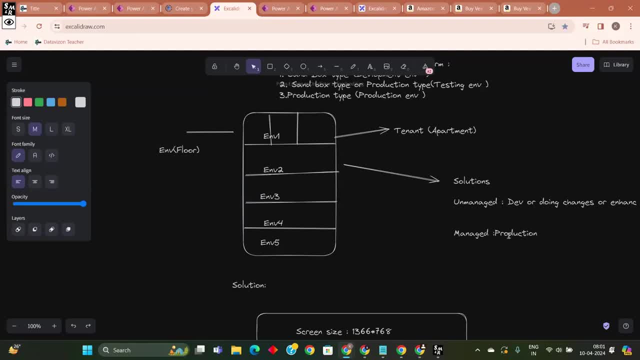 only developers, correct, but in when it comes to production, all the various users comes to production, all the various users comes to production, all the various users. so, if they are so, if they are so, if they are, uh, if, uh, if we have released that app, uh, if, uh, if we have released that app. 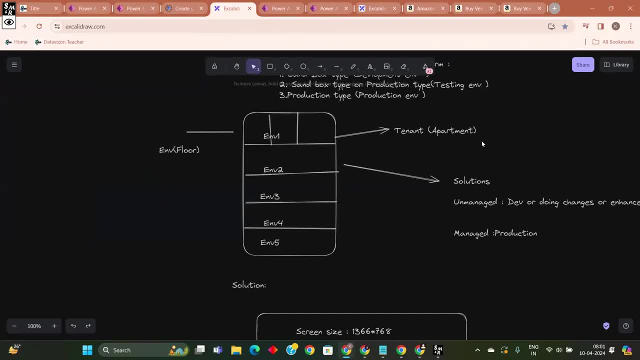 uh, if, uh, if, we have released that app to all the sales team, to all the sales team, to all the sales team of this, all the sales team. okay, all the of this. all the sales team. okay, all the of this. all the sales team. okay, all the sales team. how many sales team we are? 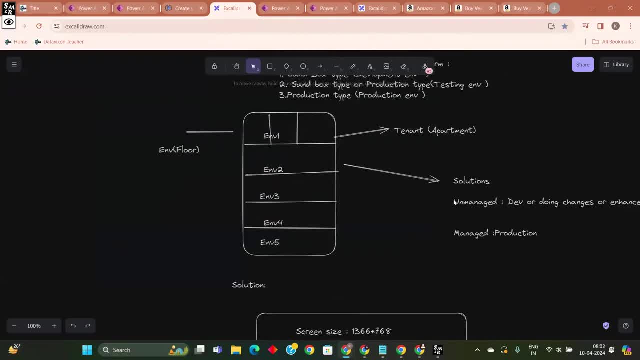 sales team, how many sales team we are sales team, how many sales team we are having for this use case? three lakh. having for this use case three lakh. having for this use case three lakh people. so if you go and change people, so if you go and change, 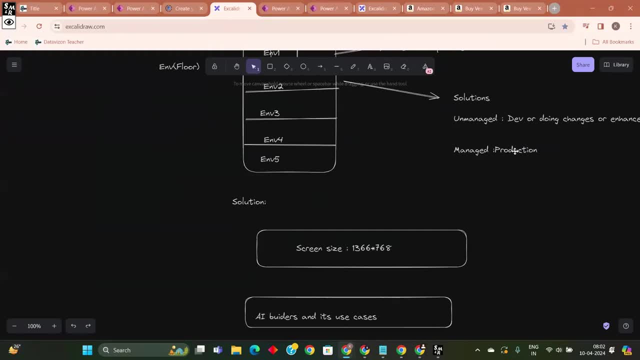 people. so if you go and change something, some solution in the something, some solution in the something, some solution in the production, what will happen? you know production. what will happen, you know production. what will happen, you know it will affect all those three lakhs. it will affect all those three lakhs. 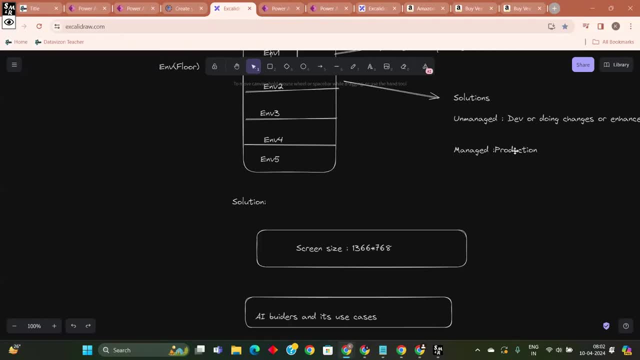 it will affect all those three lakhs people, people, people, so, so, so, to protect our two, uh, i mean like uh to protect our two. uh, i mean like uh to protect our two. uh, i mean like uh, to create a, to create a, to create a discipline, to create a discipline for. 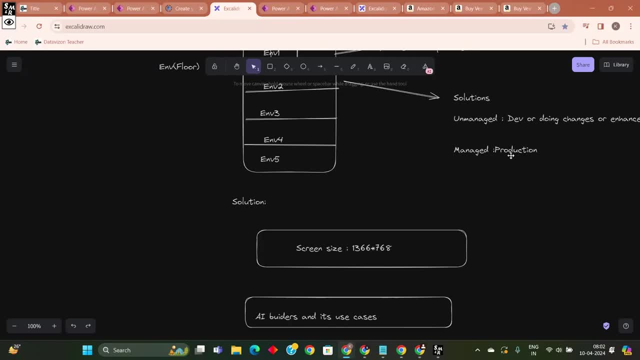 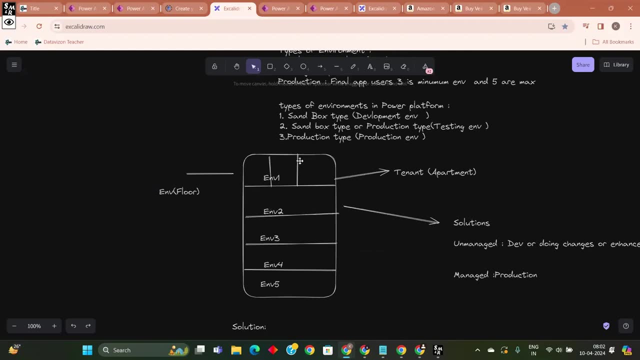 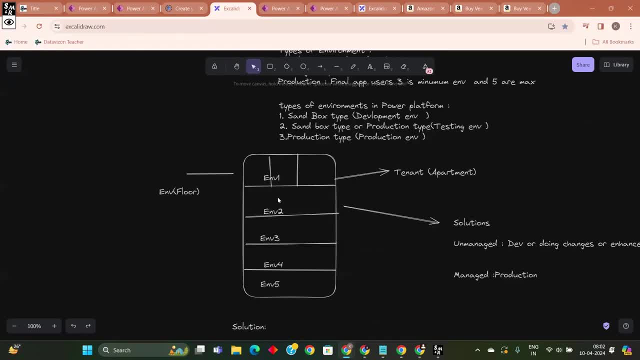 and production and production, okay so, okay so, okay. so, as we said: wow, i mean you are better. as we said: wow, i mean you are better. as we said: wow, i mean you are better: clarify: you have a better clarification. clarify: you have a better clarification. clarify: you have a better clarification and understanding of developer. 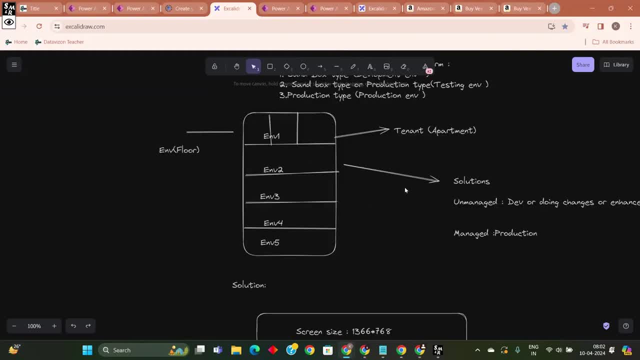 and understanding of developer and understanding of developer. environment testing environment and environment. testing environment and environment. testing environment and production environment and what type also production environment and what type also production environment and what type also. we will, we will use. you got a clarity. we will, we will use. you got a clarity. 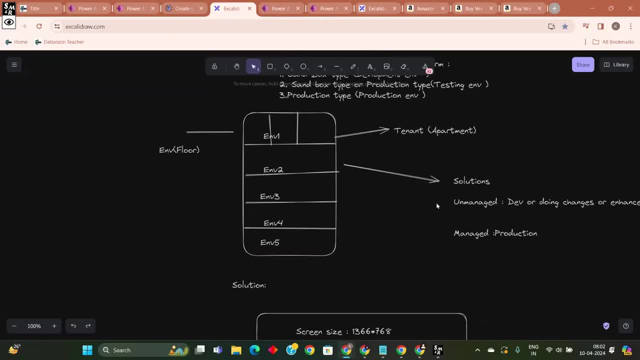 we will. we will use you got a clarity and newcomers, please go to yesterday's and newcomers, please go to yesterday's and newcomers, please go to yesterday's video. get it from my edge video. get it from my edge video. get it from my edge. ah, so here we have, manager solution. 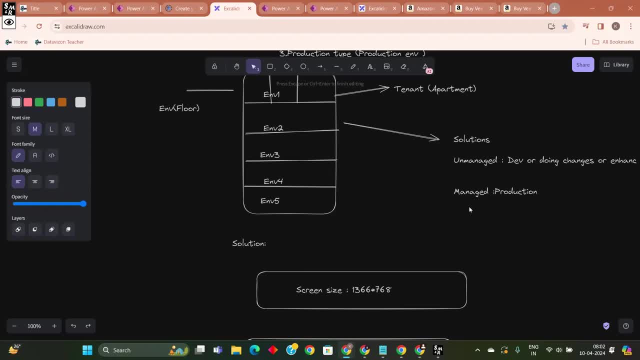 ah, so here we have manager solution. ah, so here we have manager solution. manage, the solution is nothing, but you manage the solution is nothing, but you manage, the solution is nothing, but you cannot do any changes. you cannot do any, cannot do any changes, you cannot do any. 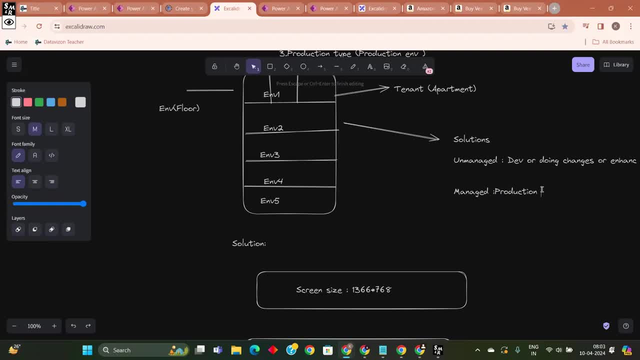 cannot do any changes, you cannot do any changes. changes, changes. if you do changes also, if you do changes also, if you do changes also, changes will appear in, changes will appear in, changes will appear in, changes will appear as, appear as appear as layers, layers, layers. so a layer is formed, a layer is formed. 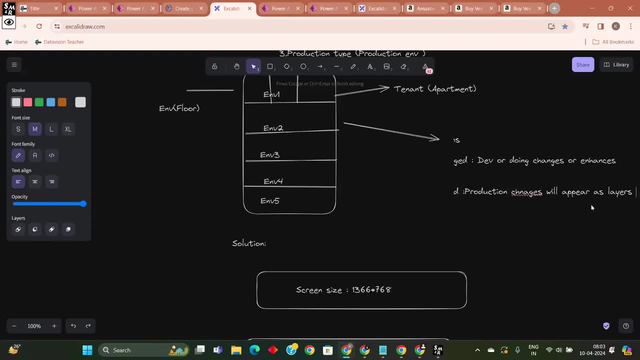 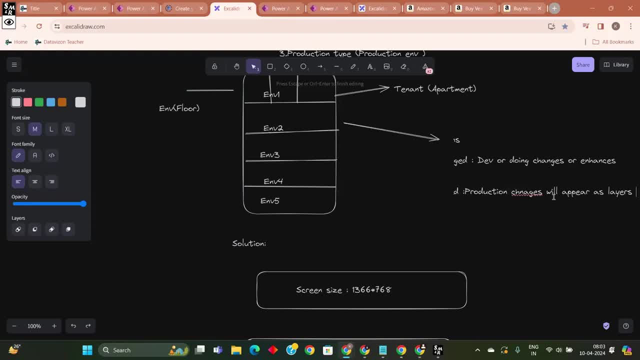 will not go live. the changes which you will not go live. the changes which you do will not go live. production changes do will not go live. the changes which you do will not go live. the changes which you will appear as layers will appear as layers will appear as layers. production will appear as layers. okay, 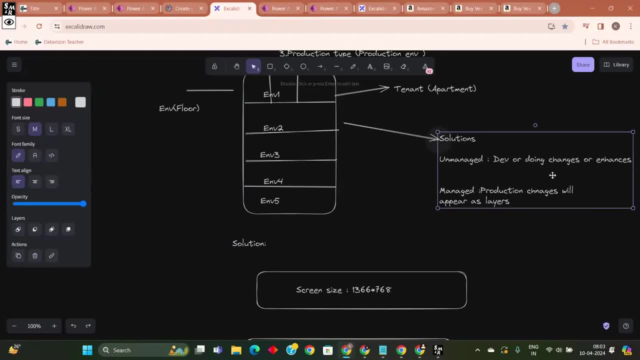 production will appear as layers. okay, production will appear as layers. okay, now these are the synopsis about now. these are the synopsis about now. these are the synopsis about solutions and solutions and solutions and uh solutions and uh solutions and uh solutions and manage the solution and manage solution. 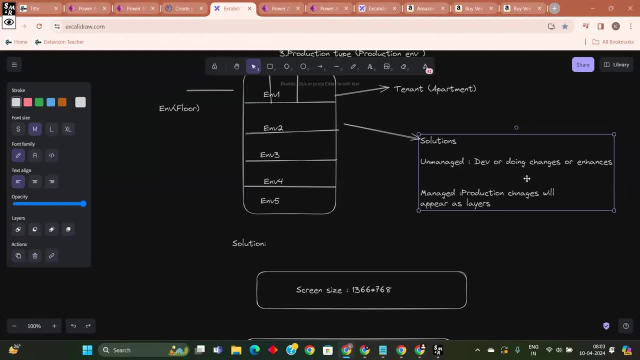 manage the solution and manage solution. manage the solution and manage solution. and we will learn more on and we will learn more on and we will learn more on in our upcoming classes. we will learn in our upcoming classes. we will learn in our upcoming classes. we will learn more. okay. 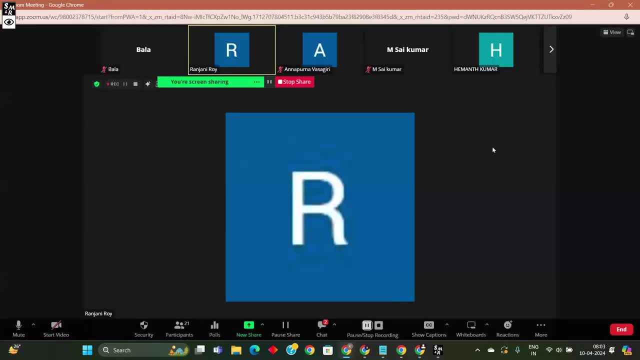 if it will not go live, then what is the? if it will not go live, then what is the? if it will not go live, then what is the use of, use of, use of? what is the use of changes? ah yes. what is the use of changes? ah yes. 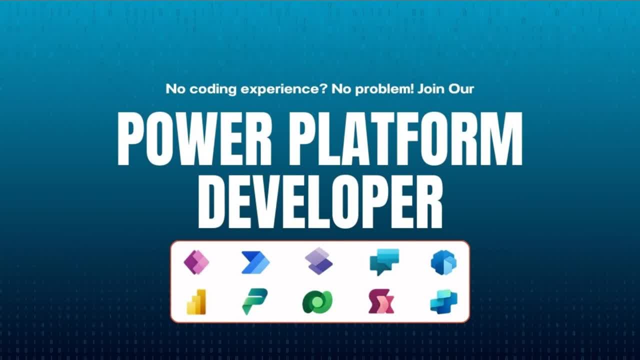 what is the use of changes? ah yes, very good question, very good question, very good question. what you will do is you will come back. what you will do is you will come back. what you will do is you will come back to your developer environment, to your developer environment. 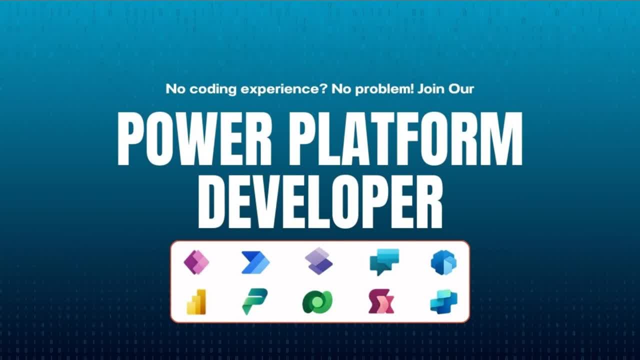 to your developer environment. whatever the changes are asked, you will. whatever the changes are asked, you will. whatever the changes are asked, you will do it in the developer environment, do it in the developer environment. do it in the developer environment. again, the process repeats the deployment. again, the process repeats the deployment. 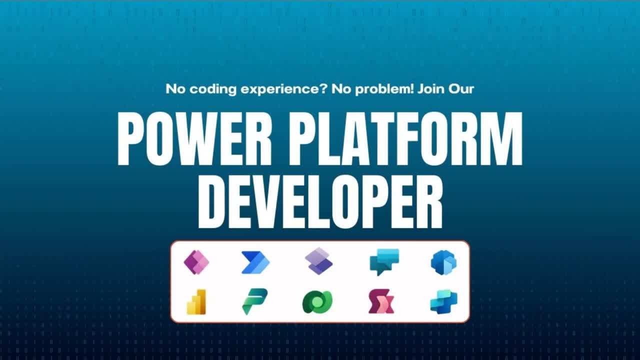 again, the process repeats the deployment. we call it deployment again, you push it. we call it deployment again, you push it. we call it deployment again, you push it: testing. someone will do the testing, they testing. someone will do the testing, they testing. someone will do the testing, they will certify. 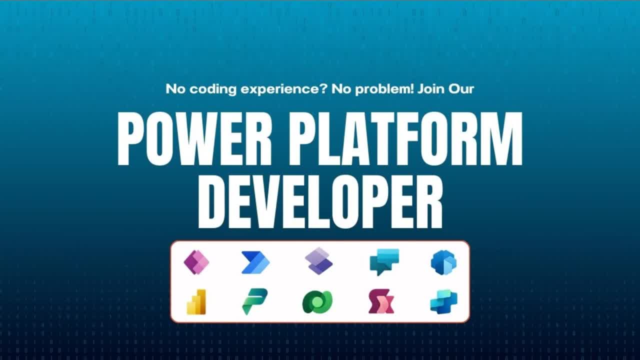 will certify. will certify, then you will send this test version to then. you will send this test version to then you will send this test version to production. very good question. production, very good question. production. very good question. correct, correct, correct production. you should not touch anything. production, you should not touch anything. 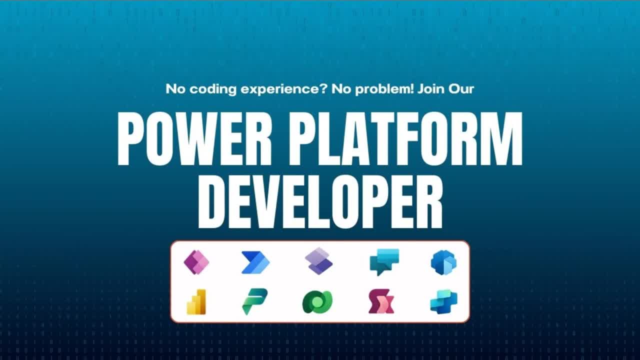 production. you should not touch anything. production is made for user. production is made for user. production is made for user. if you want to, if you want to, if you want to do what- add some new features- you will do what. add some new features. you will do what. add some new features. you will come to your developer. you will take 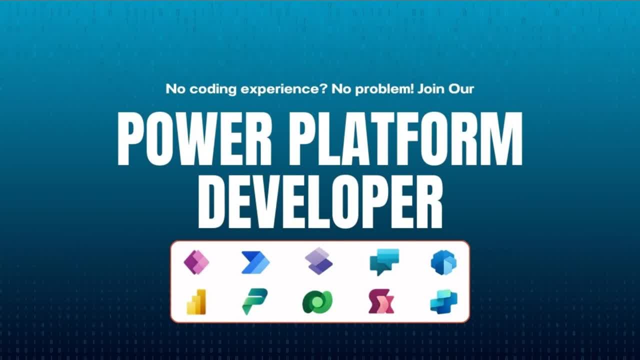 come to your developer, you will take. come to your developer, you will take your old solution. you will do the changes- your old solution. you will do the changes- your old solution. you will do the changes, then do the testing, then do the. then do the testing, then do the. 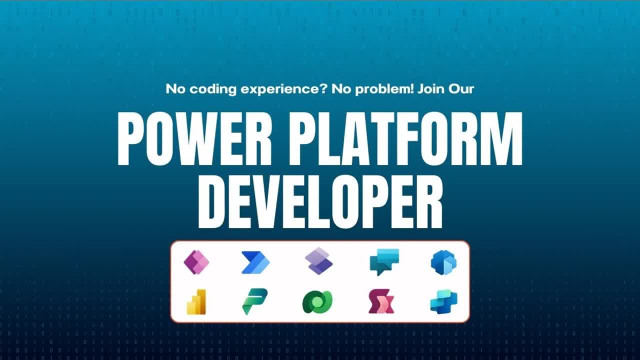 then do the testing, then do the production deployment, production deployment, production deployment. we will learn it more in pipelines. so from tomorrow we will be like starting. so from tomorrow we will be like starting. so from tomorrow we will be like starting our administration part, whatever the, our administration part, whatever the. 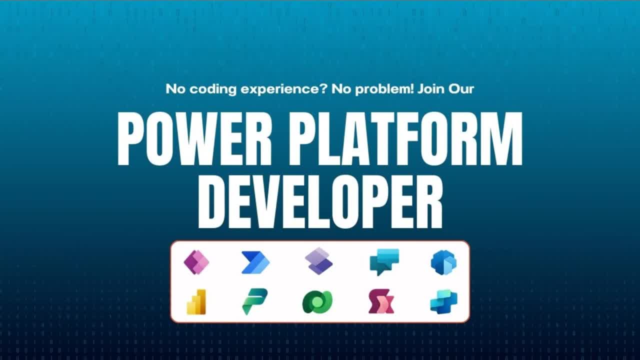 our administration part. whatever the things which happened, you know they are things which happened. you know they are things which happened. you know they are just just just baby steps. tomorrow, everyone attend baby steps. tomorrow, everyone attend baby steps. tomorrow, everyone attend from your laptop, from your laptop, from your laptop, we will be starting our 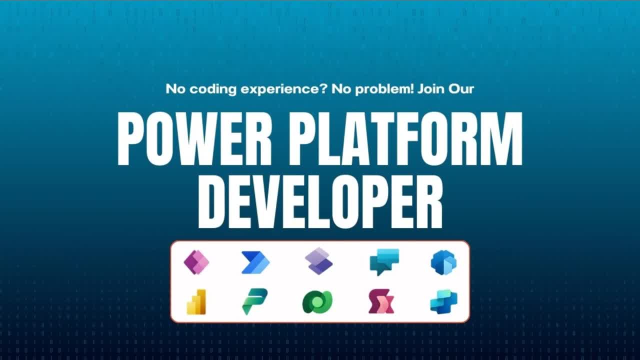 we will be starting our. we will be starting our administration. we will be starting our administration part by creating everything tenant from part. by creating everything tenant from part, by creating everything tenant from scratch okay, scratch, okay, scratch, okay. but better you get the, but better you get the. 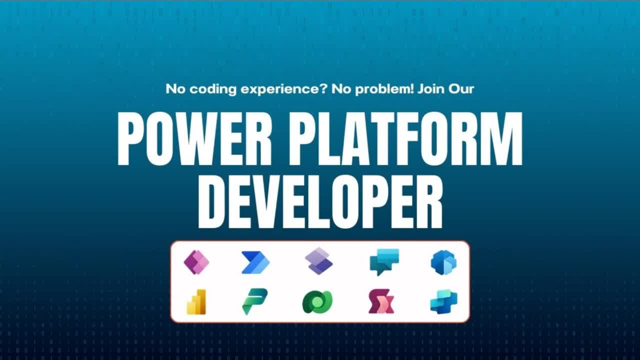 but better you get the access of our tenant ksr. access of our tenant ksr. access of our tenant ksr id. you get because that is a valid id. you get because that is a valid id. you get because that is a valid environment. it will stay with you for. 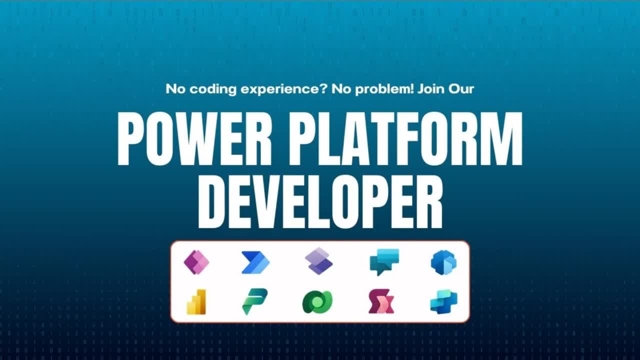 environment. it will stay with you for environment. it will stay with you for lifelong until you get jobs. lifelong until you get jobs. lifelong until you get jobs. we are not going to remove your access. we are not going to remove your access. we are not going to remove your access, okay. 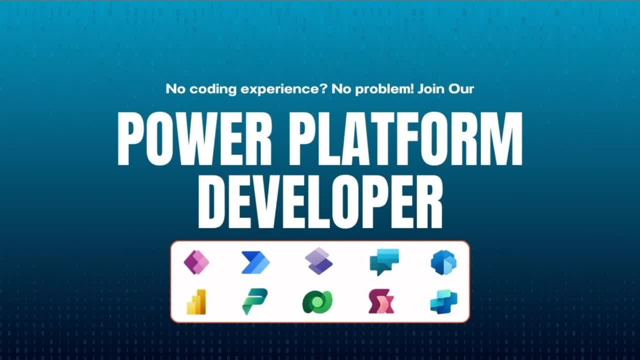 semi-structured is not there. semi-structured is not there. semi-structured is not there. vignesh, can you vignesh? can you vignesh? can you brief your question? more the same is done. brief your question: more the same is done. brief your question: more the same is done by rpa tools also, right. 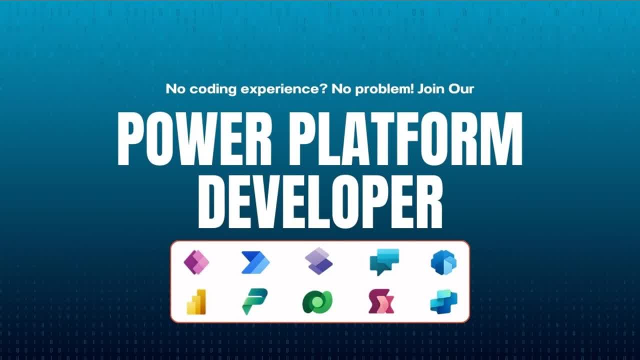 by rpa tools also right. by rpa tools also right. no, no, no that thing. we call it as web. no, no, no that thing. we call it as web. no, no, no that thing. we call it as web scrapping. scrapping, scrapping, production is different and web. 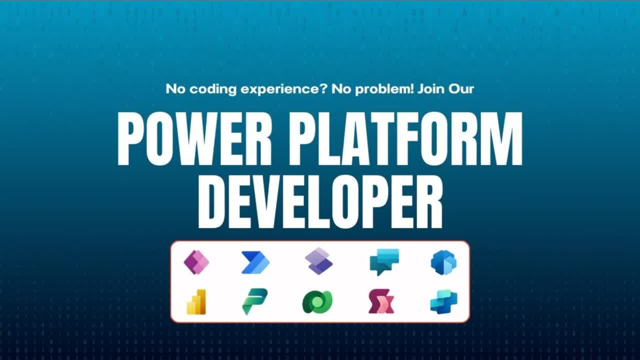 production is different and web production is different and web scrapping is different. the rpa tool, which scrapping is different. the rpa tool, which scrapping is different. the rpa tool which you have said: no, that will be. you have said no, that will be. 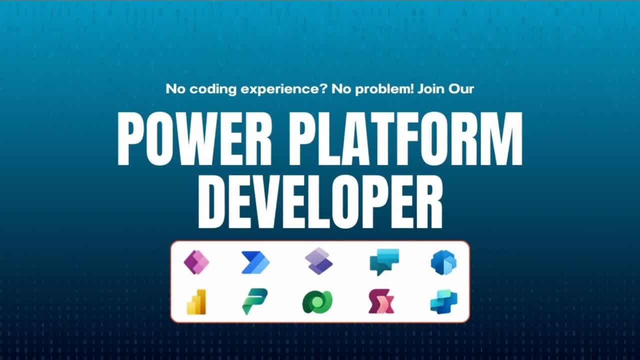 you have said no, that will be: uh uh web scrapping. we won't do uh uh web scrapping. we won't do uh uh web scrapping. we won't do production with uh web scrapping, production with uh web scrapping, rpa tool. uh, whatever, we develop bot. no. 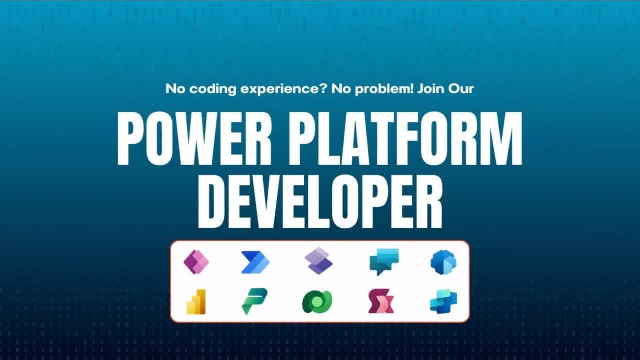 rpa tool: uh, whatever we develop bot, no. rpa tool: uh, whatever we develop bot, no, that is not a updated part. that is not a updated part. that is not a updated part. it is a programmed in such a way that it is a programmed in such a way that 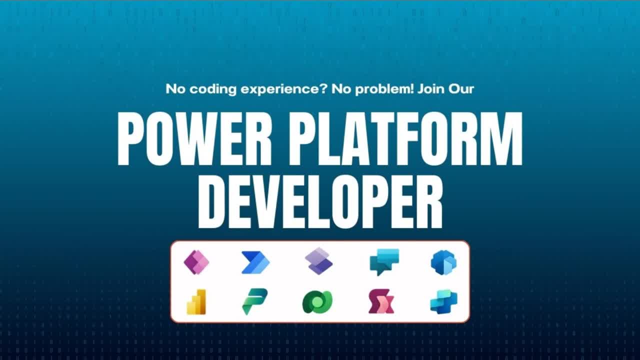 it is a programmed in such a way that, okay, you follow these steps to get this. okay, you follow these steps to get this. okay, you follow these steps to get this data. that's it data. that's it data. that's it. live prediction is not possible with the. 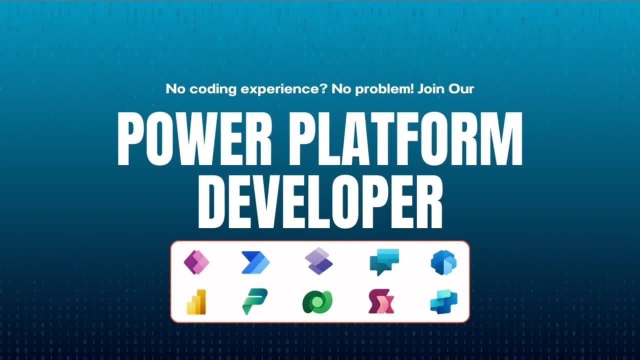 live prediction is not possible with the live prediction is not possible with the rpa. duration of the course is more than duration of the course is more than duration of the course is more than three. three months, so nearly three and a three. three months, so nearly three and a. 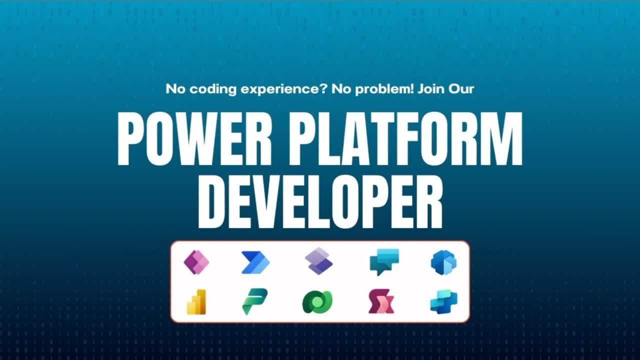 three, three months, so nearly three and a half months you can consider, and if half months, you can consider, and if half months you can consider. and if uns in unforeseen condition, if there are uns in unforeseen condition, if there are uns in unforeseen condition if there are some holidays and or else if i have some. 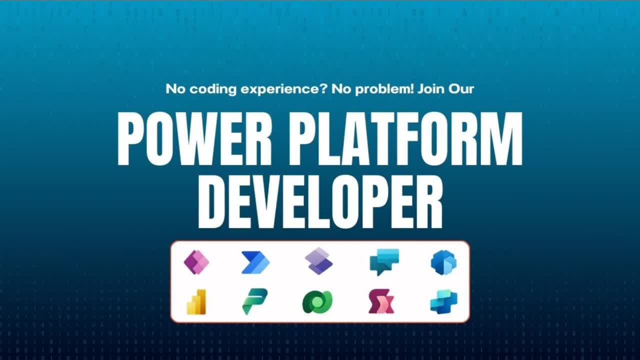 some holidays, and or else, if i have some some holidays and or else if i have some project, project, project, or else, or else, or else some, some, some. you know keeping unforeseen conditions in. you know keeping unforeseen conditions in. you know keeping unforeseen conditions in uh, few in view. 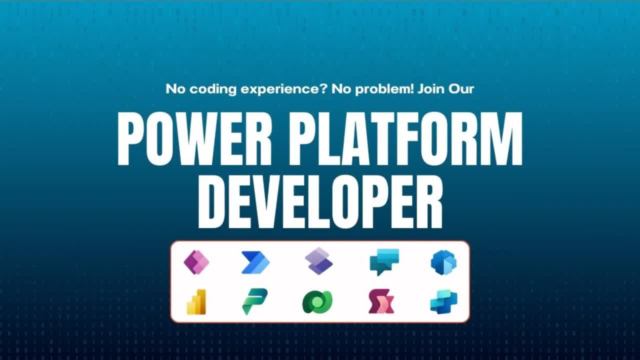 uh, few in view, uh, few in view. you can read it as four months, but more. you can read it as four months, but more. you can read it as four months, but more than three months. yeah, for every tool, we will create a new. yeah, for every tool, we will create a new. 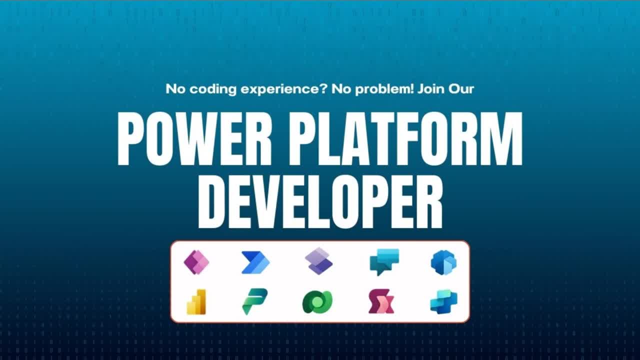 yeah, for every tool, we will create a new project from my side. i will explain you project from my side. i will explain you project from my side. i will explain you one project along with the basics and one project along with the basics, and one project along with the basics and fundamentals. and i will give you one. 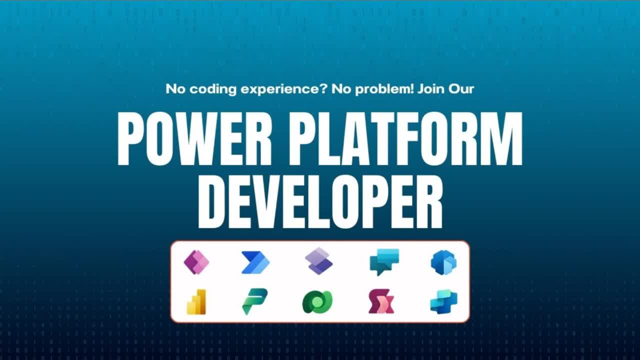 fundamentals and i will give you one fundamentals and i will give you one more project which you need to do, more project which you need to do, more project which you need to do parallelly. yes, master projects will be covered. so once, uh, in every tool i will cover. 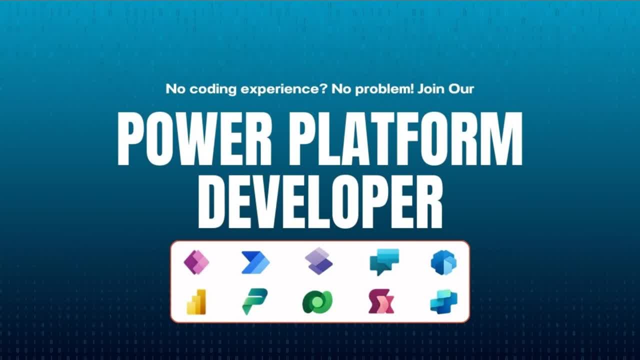 so once uh in every tool, i will cover. so once uh in every tool, i will cover some basics and, based on the basics, we some basics. and based on the basics- we some basics. and based on the basics, we will start, will start, will start developing the projects, no issues. 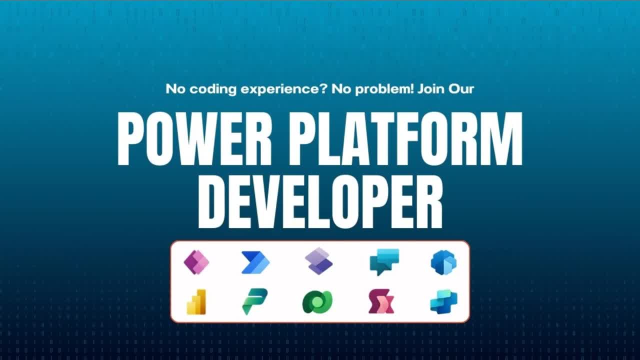 developing the projects, no issues. developing the projects, no issues. an interview, an interview, an interview: preparation, preparation, preparation. everything will be covered, everything will be covered, everything will be covered. thank you, okay, uh, for uh two weeks. or thank you okay, uh, for uh two weeks. or thank you okay, uh, for uh two weeks. or 15 days, uh, in a, in a month, i will take. 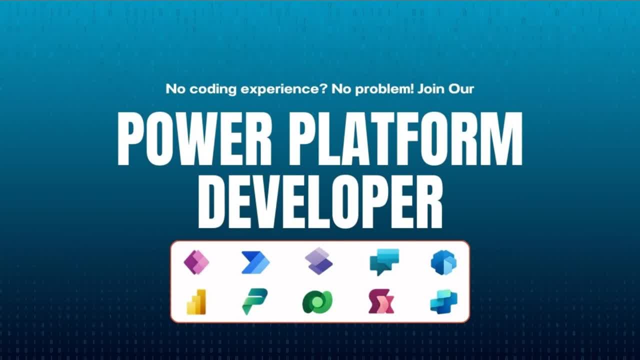 15 days, uh, in a in a month. i will take 15 days, uh, in a in a month. i will take mock interviews, mock interviews, mock interviews. and you know, and you know, and you know, basically i am asking you some questions, basically i am asking you some questions. 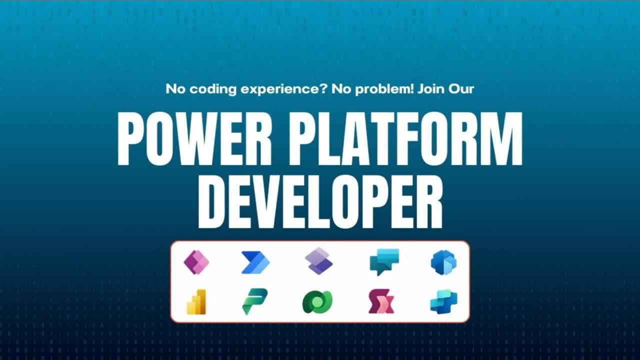 basically, i am asking you some questions in the, in the between the classes, in the in the in the between the classes, in the, in the in the between the classes. those questions only as it is. you will those questions only as it is. you will those questions only as it is. you will get in an interview. 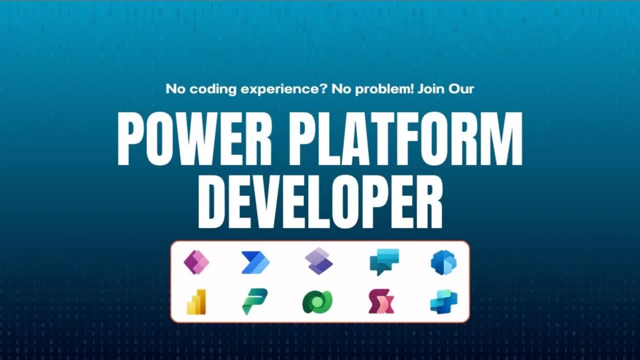 get in an interview, get in an interview, okay, okay, okay. so out of 10 questions, seven questions. so out of 10 questions, seven questions. so out of 10 questions, seven questions. what i am asking you in the class where. what i am asking you in the class where. 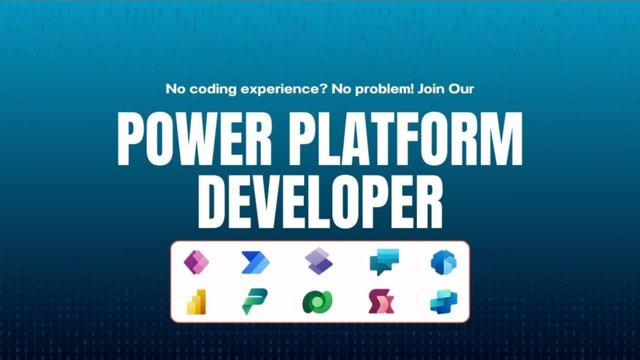 what i am asking you in the class where i am like, i am like, i am like uh pointing more and more. they are only uh pointing more and more. they are only uh pointing more and more. they are only part of your interview questions. part of your interview questions. 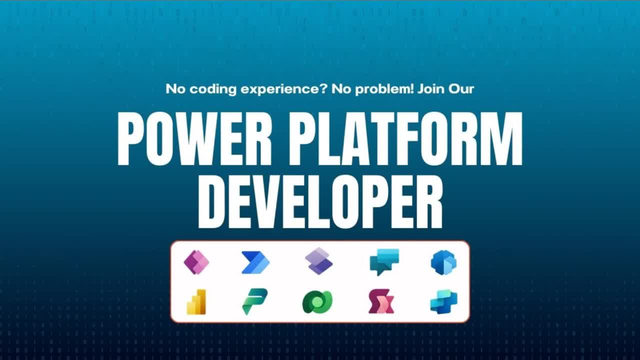 part of your interview questions i'm stressing some point is at the- i'm stressing, some point is at the i'm stressing, some point is at the interview question, interview question, interview question. and today also i have an interview with: and today also i have an interview with. 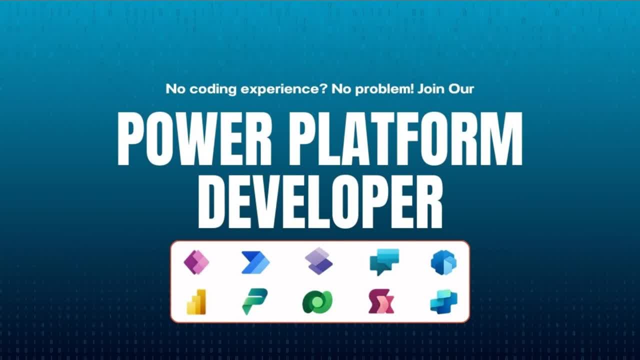 and today also i have an interview with bb company. i do interviews bb company. i do interviews bb company. i do interviews, even my team do in case. i do interviews, even my team do interviews, even my team do interviews, along with our students. you just get the, along with our students. you just get the. 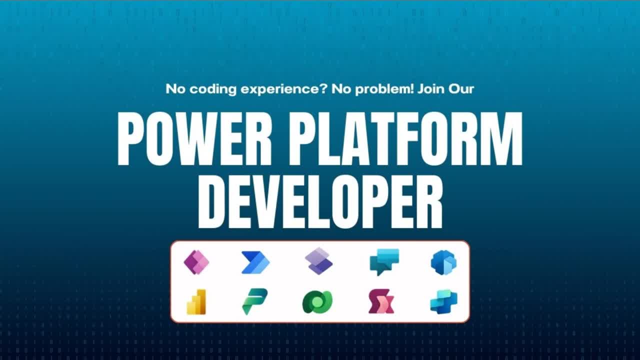 along with our students. you just get the questions for you guys, questions for you guys, questions for you guys. so it is also going to be very practical. so it is also going to be very practical. so it is also going to be very practical. the questions which are lively asked in: 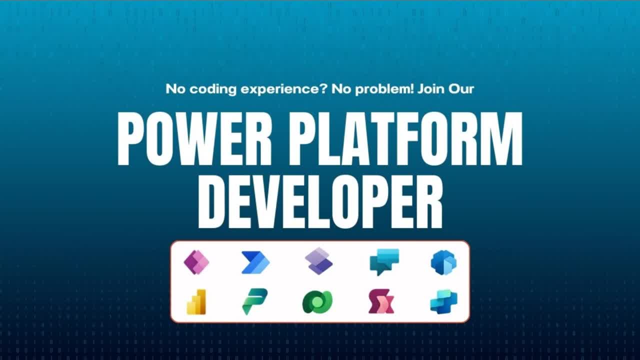 the questions which are lively asked in the questions which are lively asked in the interviews, those only the interviews, those only the interviews, those only uh. i'll make. is this clear? is this clear? is this clear? what about the certifications like uh if? what about the certifications like uh, if? 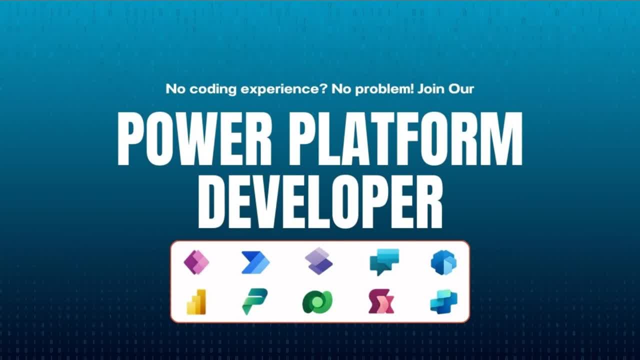 what about the certifications? like: uh, if you need any certifications, you need any certifications, you need any certifications. very good question. so we are a very good question. so we are a very good question. so we are a microsoft certified partner, microsoft certified partner, microsoft certified partner. if you, some certification is costing 5000. 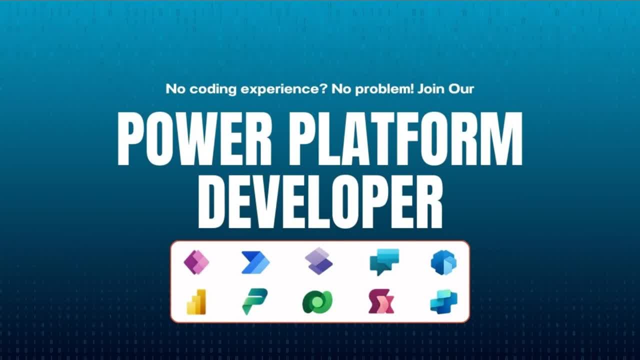 if you, some certification is costing 5000, if you, some certification is costing 5000 for you, for you, for you, we will give you a coupon code once you. we will give you a coupon code once you. we will give you a coupon code once you register. you will get a 50 discount. 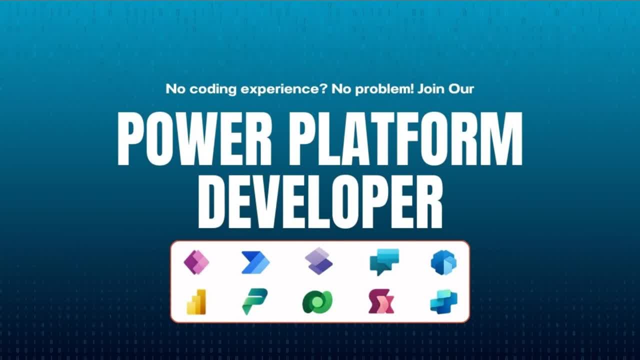 and the certifications which you can, and the certifications which you can and the certifications which you can prepare. so if you complete, if you give prepare, so if you complete, if you give prepare, so if you complete, if you give me 100 from your side, from your side, 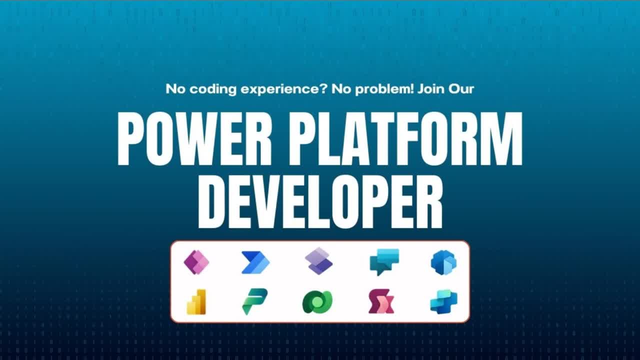 me 100 from your side, from your side, me 100 from your side, from your side, through to my entire training, like uh, through to my entire training, like uh, through to my entire training, like uh. submitting the assignments, submitting the, submitting the assignments, submitting the, submitting the assignments, submitting the task and doing the documentation which 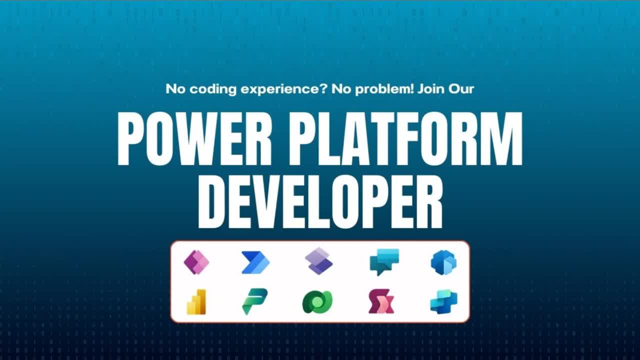 task and doing the documentation, which task? and doing the documentation which i ask you to do. if you do properly, you i ask you to do, if you do properly you i ask you to do, if you do properly, you will be eligible for pl 900, will be eligible for pl 900. 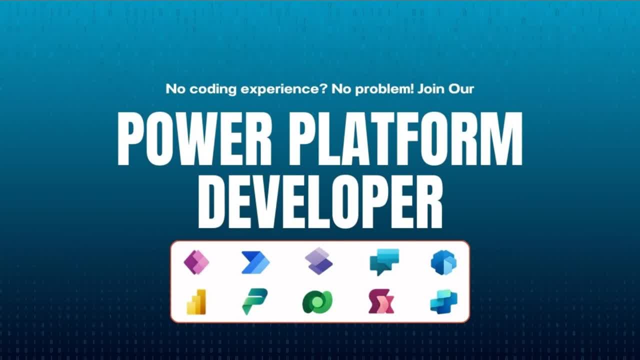 will be eligible for pl 900, pl 100 and pl 200 but pl 100. they are pl 100 and pl 200 but pl 100. they are pl 100 and pl 200 but pl 100. they are like removing it's power up maker. but. 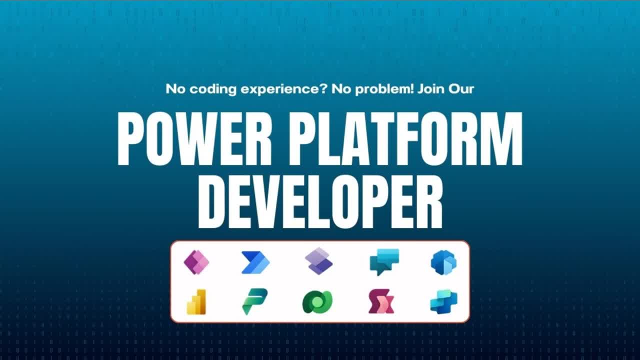 like removing it's power up maker, but like removing it's power up maker. but pl 200 power up consultant. so these three: pl 200 power up consultant, so these three. pl 200 power up consultant, so these three you can easily cover bl100 and pl uh. 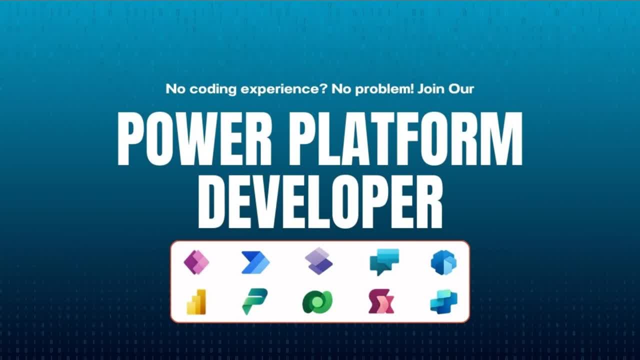 you can easily cover bl100 and pl uh. you can easily cover bl100 and pl uh. 200.. 200.. 200.. okay, okay, okay, we'll be, i can guarantee you, sorry, we'll be, i can guarantee you, sorry, we'll be, i can guarantee you sorry. pl 300 is power bi and in this power bi, 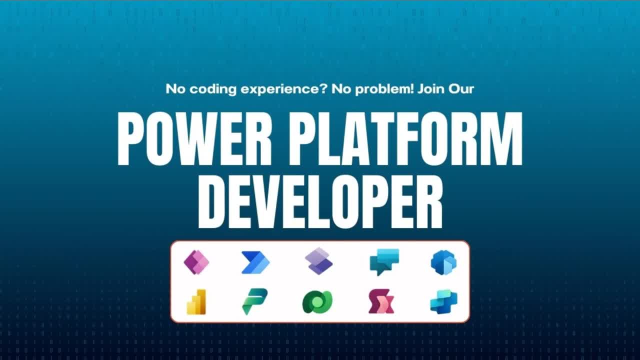 pl 300 is power bi and in this power bi. pl 300 is power bi and in this power bi uh in this uh particular uh power uh in this uh particular uh power, uh in this uh particular uh power platform. no you, actually there are a lot. 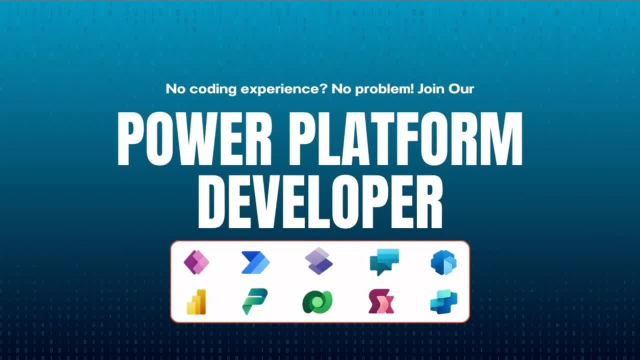 platform. no, you, actually there are a lot platform. no, you, actually there are a lot of power bi developers, actually of power bi developers, actually of power bi developers, actually. so if you want to clash with them, no, uh. so if you want to clash with them, no, uh. 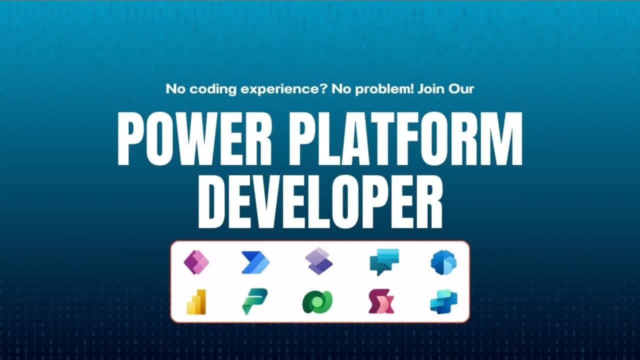 so if you want to clash with them, no, uh, it becomes difficult. that is why we have it becomes difficult. that is why we have it becomes difficult. that is why we have certain modifications. so, even if you are certain modifications, so, even if you are certain modifications, so even if you are going with a power bi course also we 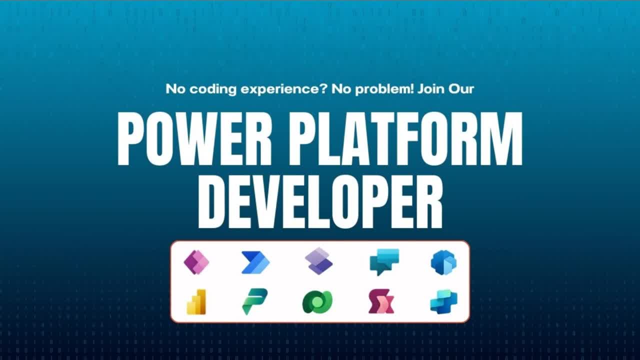 going with a power? bi course also we going with a power. bi course also we are. we are doing it with fabric. are we are doing it with fabric? are we are doing it with fabric? our main focus is to clear the market. our main focus is to clear the market. 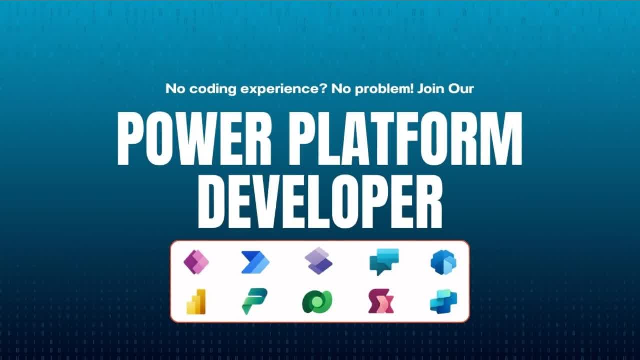 our main focus is to clear the market and get the job here. if you focus on and get the job here, if you focus on and get the job here, if you focus on just power bi- no uh, there will be like. just power bi- no uh, there will be like. 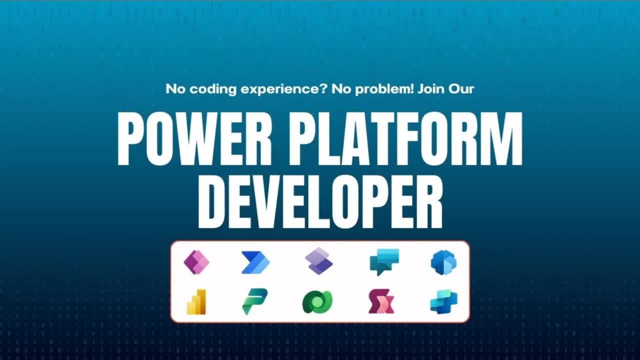 just power bi. no, uh, there will be like: in pl 900, power bi questions will be in pl 900, power bi questions will be in pl 900, power bi questions will be there. so if you have pl 900 there, so if you have pl 900. 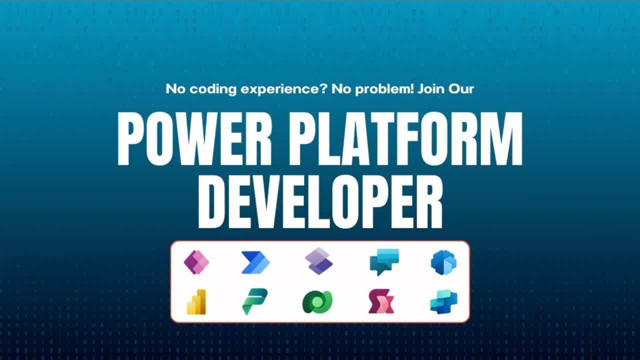 there. so if you have pl 900 or pl 200, you will be validated, you will. or pl 200, you will be validated, you will. or pl 200, you will be validated, you will be automatically validated. power bi uh be automatically validated. power bi uh be automatically validated. power bi uh, engineer. no questions in that. 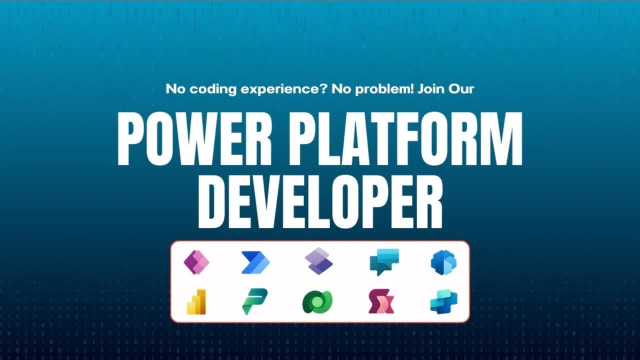 engineer. no questions in that. engineer, no questions in that. if you go over pl 300, the topic is only if you go over pl 300. the topic is only if you go over pl 300. the topic is only power power bi. if you go with pl 900. 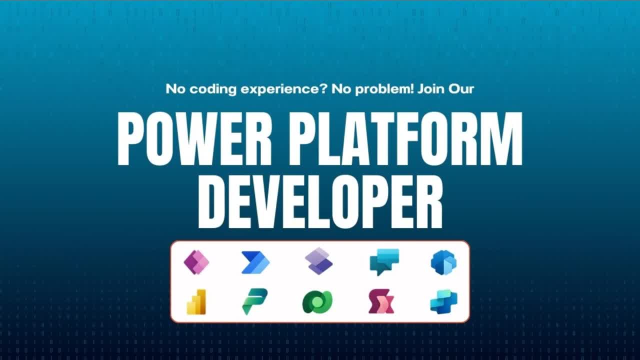 power power bi. if you go with pl 900. power power bi. if you go with pl 900. fundamentals of power apps- power fundamentals of power apps. power fundamentals of power apps. power automate power bi: all are covered if automate power bi, all are covered. if automate power bi, all are covered. if you go with pl 200, consultant related. 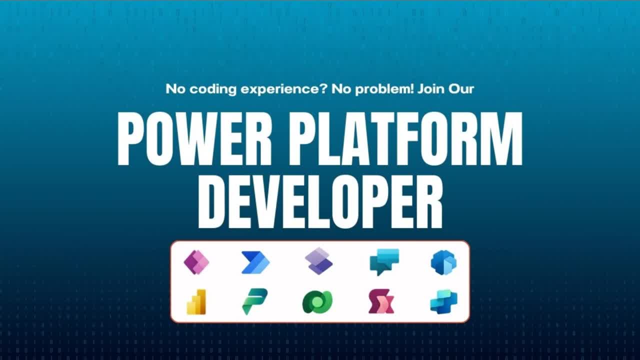 you go with pl 200 consultant related. you go with pl 200 consultant related. power bi power apps. power automate ai. power bi power apps. power automate ai. power bi power apps. power automate ai. builders- uh, every tool will be covered. builders- uh, every tool will be covered. 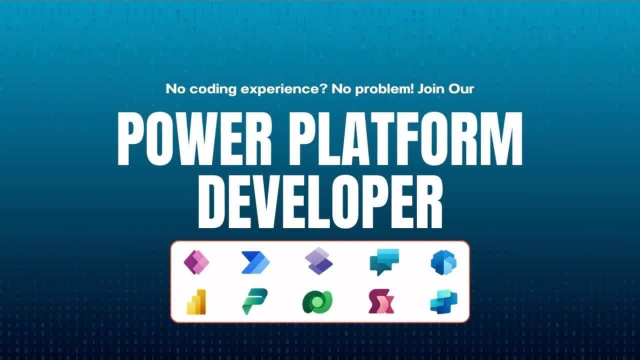 builders: uh, every tool will be covered. model revealed data verse- correct action. model revealed data verse- correct action. model revealed data verse correct action. okay, yeah, uh, uh, uh, raj, raj, raj, yes, yes, yes, okay, so, um, um, um, will you going to cover uh data verse? if so, 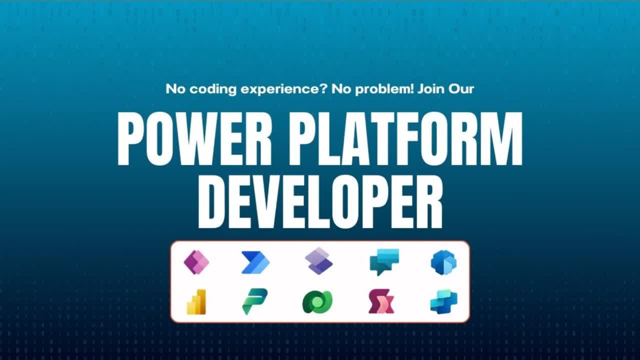 will you going to cover uh data verse? if so, will you going to cover uh data verse? if so, right, how right, how right, how yeah, yeah, yeah, yeah, yeah, yeah. data was complete from scratch. data was complete from scratch. data was complete from scratch, from scratch. to creating an app. uh model you. 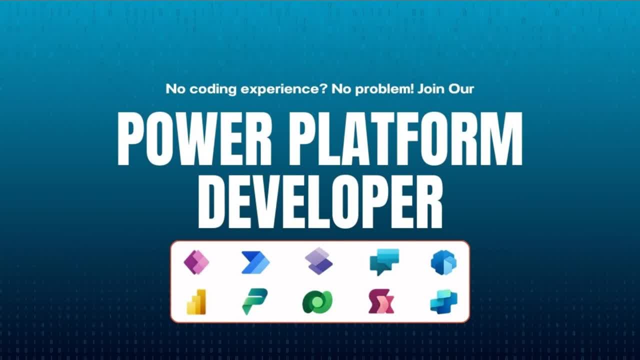 from scratch to creating an app. uh, model you from scratch to creating an app. uh, model you an app from that. we'll cover an app from that. we'll cover an app from that. we'll cover everything, everything, everything. okay, is it? uh are we going to cover? 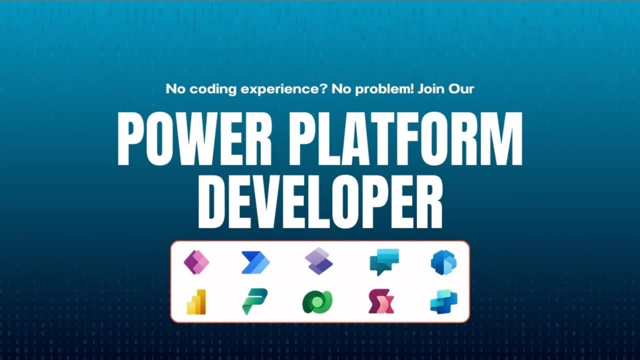 okay, is it uh, are we going to cover? okay, is it uh? are we going to cover? plugins, something plugins, something plugins, something plug-ins. are you a c-sharp developer? are plug-ins. are you a c-sharp developer? are plug-ins? are you a c-sharp developer? are you from crm background? 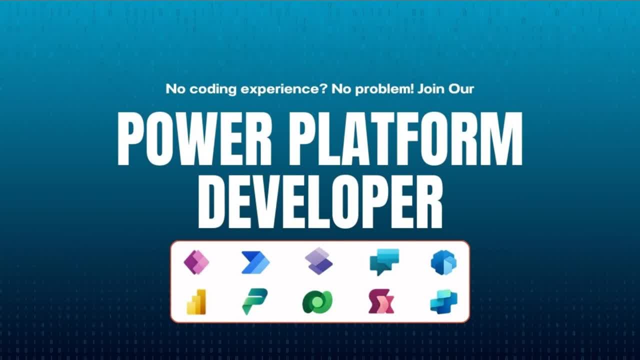 uh, i'm c-sharp developer. uh, i'm c-sharp developer. uh, i'm c-sharp developer, c-sharp. okay. so i will give you some c-sharp. okay, so i will give you some c-sharp. okay. so i will give you some assignments separately, because 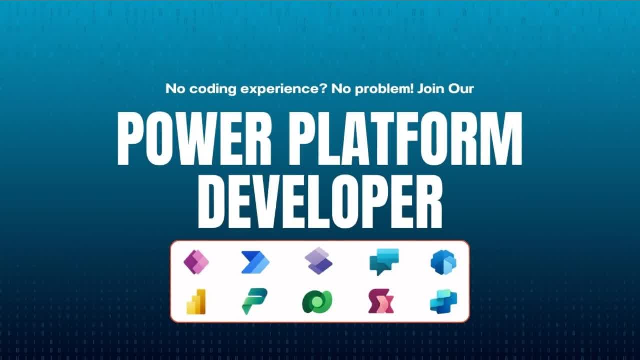 assignments separately. because assignments separately? because most of the students, you know uh, if i most of the students, you know uh, if i most of the students, you know uh, if i introduce c-sharp code and all those introduce c-sharp code and all those introduce c-sharp code and all those things at the earlier stages it is. 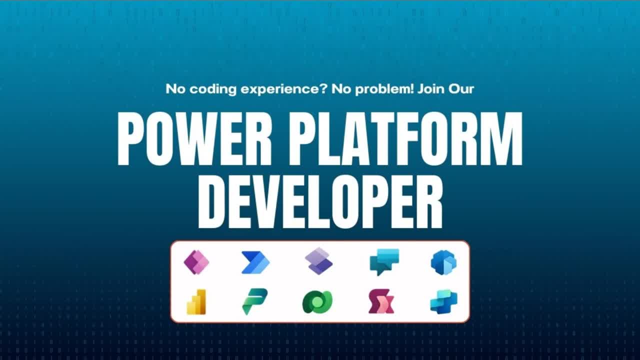 things at the earlier stages. it is things at the earlier stages. it is impossible. so i will give you separately impossible. so i will give you separately impossible, so i will give you separately those things and you can work on that, those things and you can work on that. 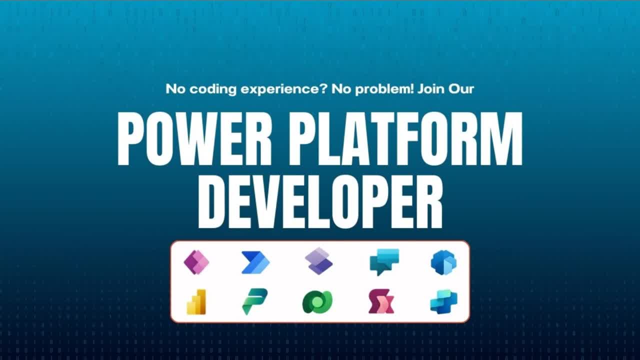 those things and you can work on that and implement, and implement, and implement. no and no and no, and in most of the first crm developer only in most of the first crm developer, only in most of the first crm developer only. uh, it's like plugins are asked in. 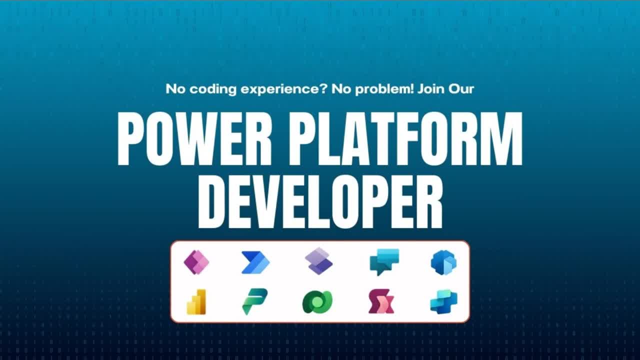 uh, it's like plugins are asked in. uh, it's like plugins are asked in interviews, or else interviews, or else interviews, or else ask. but there will be a separate team for ask. but there will be a separate team for ask. but there will be a separate team for uh making plugins. that is crm. 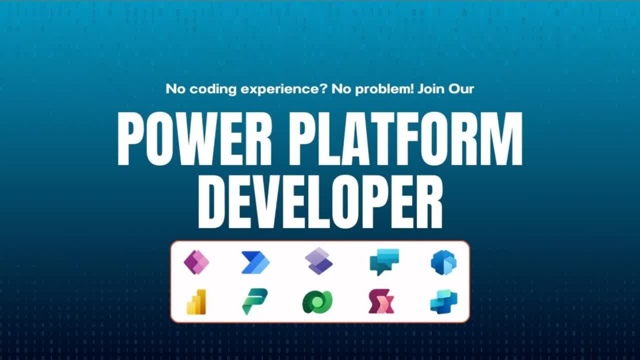 uh, making plugins, that is crm. uh, making plugins, that is crm. developers, developers, developers. they will make the plug-in and give it. they will make the plug-in and give it. they will make the plug-in and give it to you, to you, to you. okay, if you want to give a, introduce a. 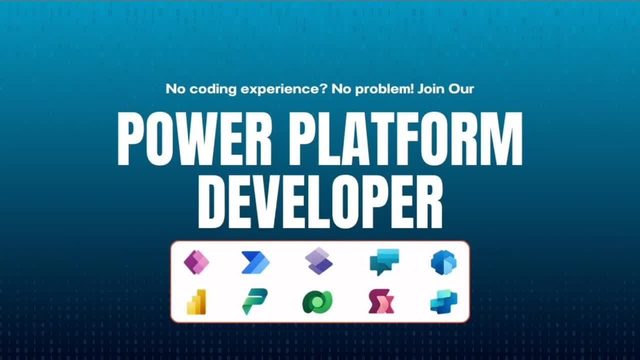 okay, if you want to give a, introduce a. okay, if you want to give a, introduce a custom custom code, we will do it with custom custom code. we will do it with custom custom code. we will do it with a javascript which is related to uh. a javascript which is related to uh. 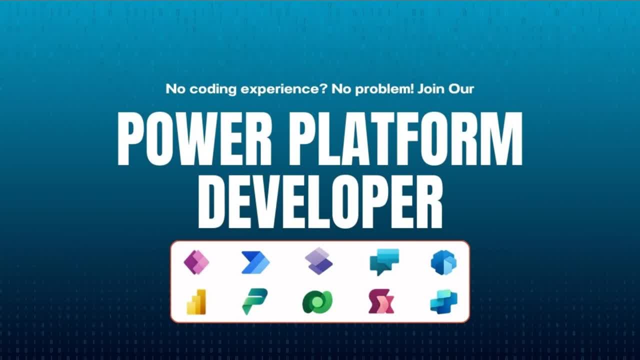 a javascript which is related to, uh, dynamics javascript. we will implement so dynamics javascript. we will implement so dynamics javascript. we will implement so that thing when, when we are doing model that thing, when, when we are doing model that thing, when, when we are doing model d1 application in the customization of 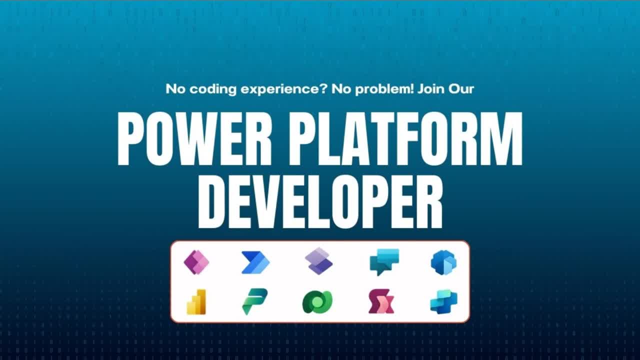 d1 application. in the customization of d1 application, in the customization of the model d1 application, we will come to the model d1 application. we will come to the model d1 application. we will come to know that you will cover right, that you will cover right. 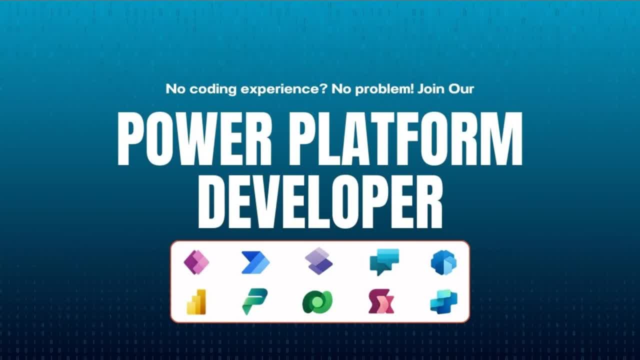 that you will cover right. yes, yes, yes, okay uh. crm means uh, you said like uh uh. crm means uh. you said like uh. uh. crm means uh. you said like uh. say, say, say, force like that, force like that, force like that right, application like that. we have a. 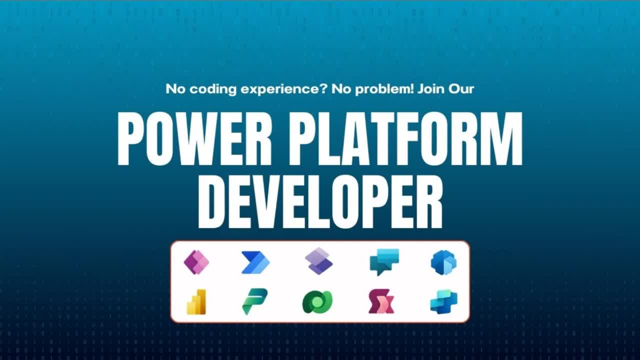 right application like that. we have a right application like that. we have a same competitor in microsoft dynamics, same competitor in microsoft dynamics, same competitor in microsoft dynamics. that is called ms crm dynamic crm. that is called ms crm dynamic crm. that is called ms crm dynamic crm. but all the features, what you have in. but all the features, what you have in, but all the features what you have in, dynamic crm we will have. we will cover dynamic crm, we will have. we will cover dynamic crm, we will have. we will cover it in the model d1 application as the. 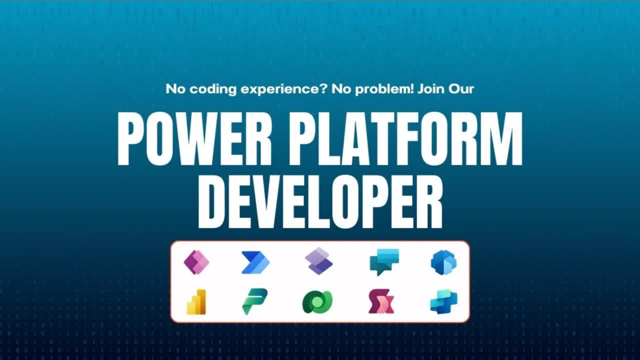 it in the model d1 application as the it in the model d1 application as the power platform developer. power platform developer. power platform developer. so if you take a crm application, now you. so if you take a crm application, now you. so if you take a crm application now you can make an hr application, you can make. 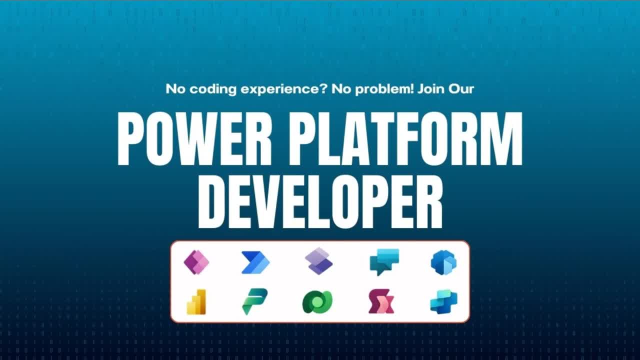 can make an hr application. you can make can make an hr application. you can make a production application. you can make a a production application. you can make a a production application. you can make a manufacturing application possibilities. manufacturing application possibilities. manufacturing application possibilities are high. you can make a shipping. 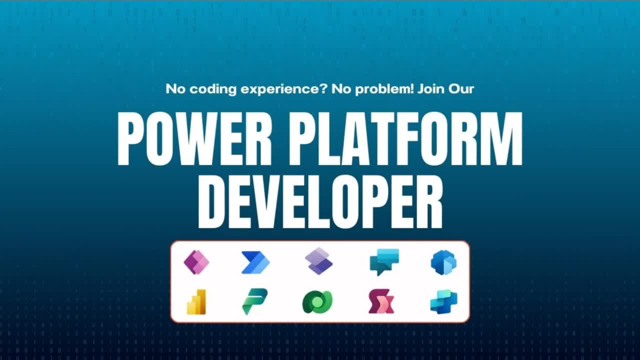 are high. you can make a shipping are high. you can make a shipping application application application. if you do it from scratch and that, if you do it from scratch and that, if you do it from scratch and that hours. but if you buy the dynamic crm, you 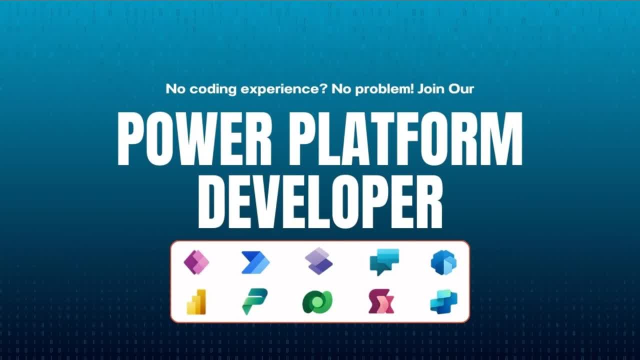 hours, but if you buy the dynamic crm, you hours, but if you buy the dynamic crm, you can only cover the sales modules, can only cover the sales modules, can only cover the sales modules. so that is a disadvantage. okay, okay, okay, power automated cloud will be covered. 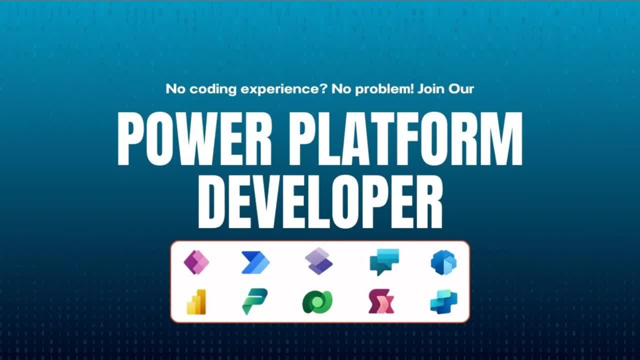 power automated cloud will be covered. power automated cloud will be covered because you are a power platform. because you are a power platform, because you are a power platform developer. if you are an rpi developer, we developer. if you are an rpi developer, we developer. if you are an rpi developer, we. we will focus on power automate desktop. 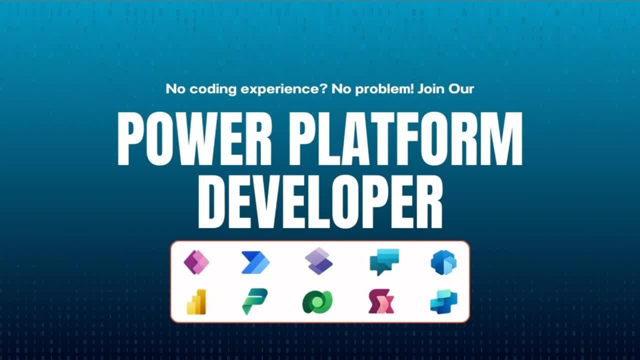 we will focus on power automate desktop. we will focus on power automate desktop, but i will give some. i will take some, but i will give some. i will take some, but i will give some. i will take some sessions on power automate desktop. sessions on power automate desktop. 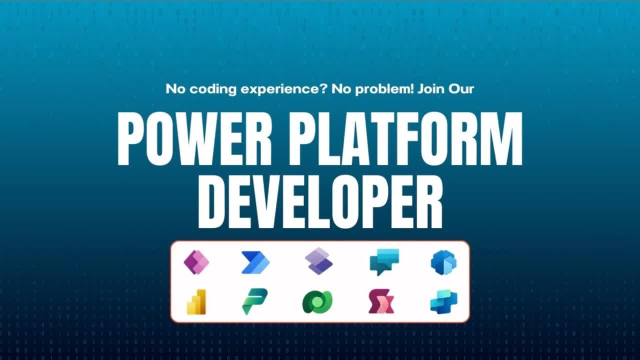 sessions on power automate desktop and, if you want to, and if you want to, and if you want to, if you have self-motivation, if you have self-motivation, if you have self-motivation, you can uh learn it from internet, i can. you can uh learn it from internet, i can. 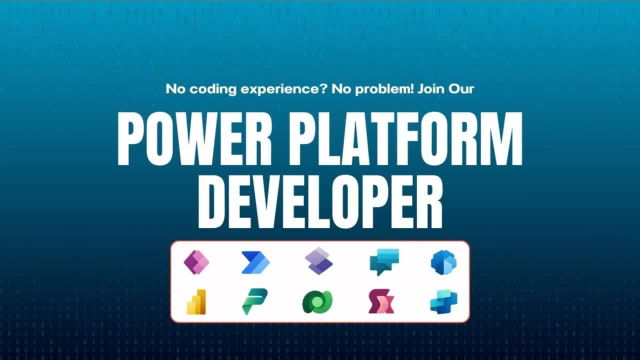 you can uh learn it from internet. i can guide you on a power automate desktop, guide you on a power automate desktop, guide you on a power automate desktop. but we will soon launch a course on rpa. but we will soon launch a course on rpa. but we will soon launch a course on rpa in that we will cover both uipath and 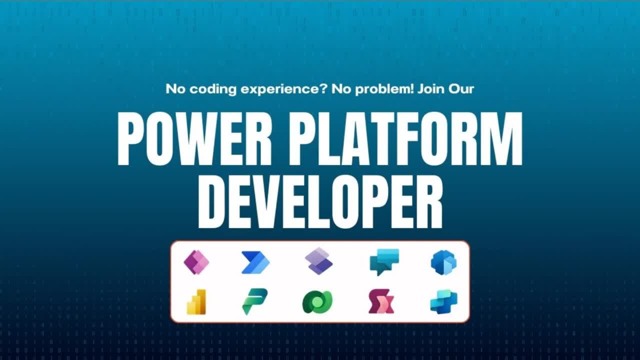 in that we will cover both uipath and in that we will cover both uipath and power: automate desktop power. automate desktop power. automate desktop, master, master, master. so in this course we will cover cloud only. so in this course we will cover cloud only. so in this course we will cover cloud only and some basic topics of desktop. 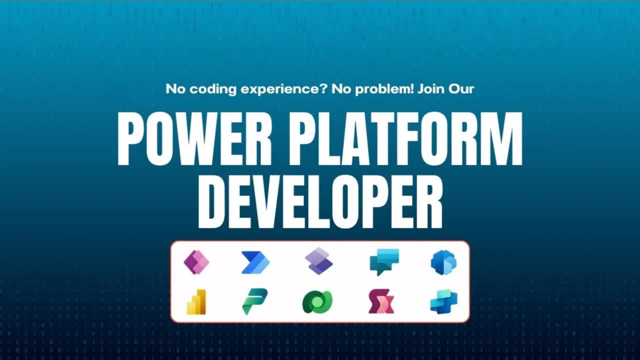 and some basic topics of desktop and some basic topics of desktop, which is enough for you, which is enough for you, which is enough for you. so there will be a lot of similarities, so there will be a lot of similarities. so there will be a lot of similarities between power, automate, cloud and power. 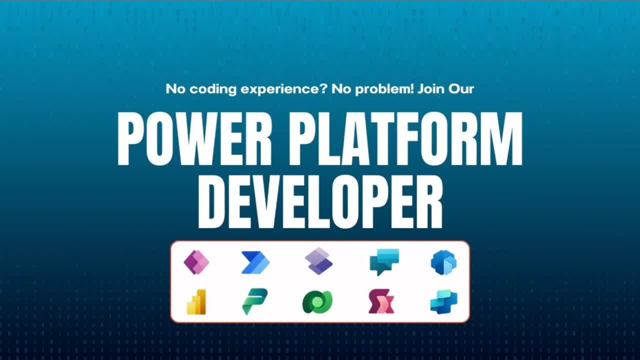 between power- automate cloud and power. between power- automate cloud and power- automate desktop- automate desktop, automate desktop. if you are in a position to identify, if you are in a position to identify, if you are in a position to identify those uh, those uh, those uh changes by keeping some time on power. 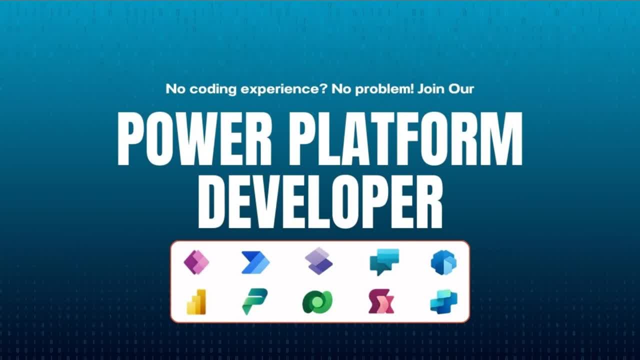 changes, by keeping some time on power changes, by keeping some time on power automate desktop, automate desktop, automate desktop. uh definitely, uh definitely, uh definitely, how you start and how you develop, uh, how you start and how you develop, uh, how you start and how you develop, uh, what's in the power automate desktop? i? 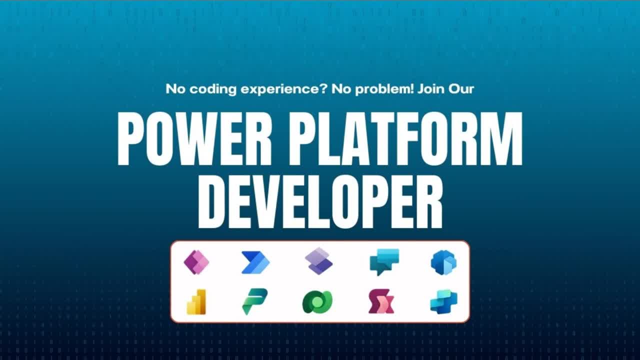 what's in the power automate desktop i, what's in the power automate desktop? i will definitely give insights. okay, basket, but not the entire desktop. okay, basket, but not the entire desktop. okay, basket, but not the entire desktop, because desktop only will take me 45, because desktop only will take me 45. 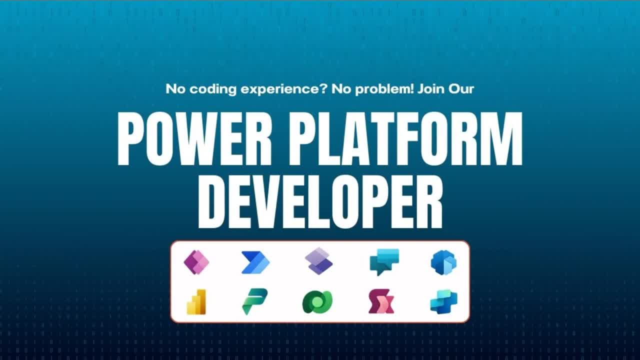 because desktop only will take me 45 days, days, days to compete 40. any other questions? yeah, i have a question. yeah, i have a question. yeah, i have a question. so, so, so, for example, for example, for example, i'll consider like power b, i'll consider like power b. 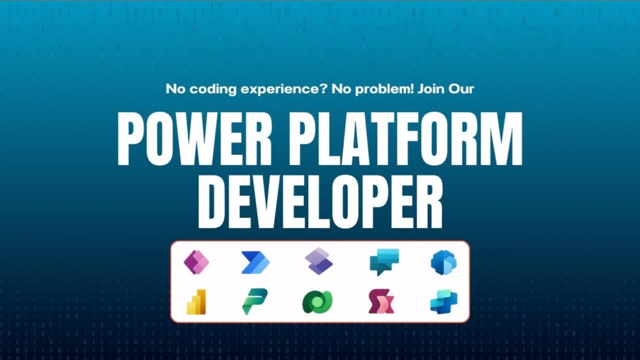 that have been created a report, so the data source is like: i'll cancel some sql, so there will be. there will be a manual testing going on, like every day. a tester used to develop do the testing. it's like a regressive testing or something like that. so can we automate? 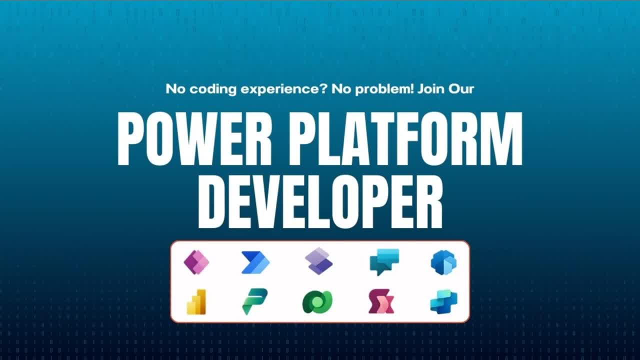 the testing. whatever he picks, like manually writing the sql code, whatever he do, he writes the test cases. can we automate that one using power apps? about automate testing use cases: till now we didn't got to automate. okay, testing is something which is done rigorously from point to point. if there is a screen, so in this screen i will see karti, i will. 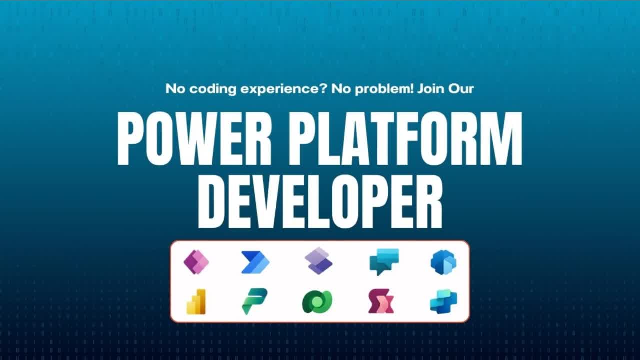 i will screen praveen, i will screen anna purna, i will screen emma. if i want to do a functional testing, as a tester, i need to check your spellings, i need to check the card. if the card, the card is coming properly, if this card is a responsive, if this card is correct and if this card is placed in the 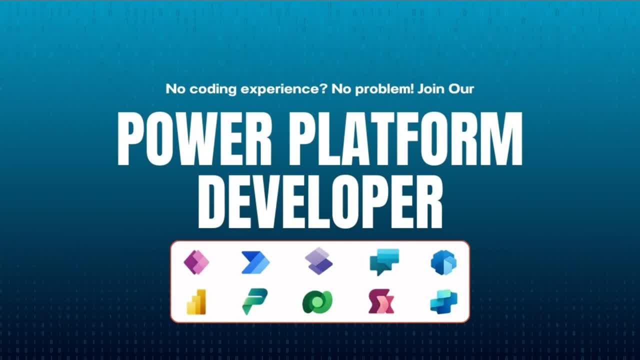 proper way. my speaker name is coming in the center or not. these things can be done manually only by the tester. okay, and if you automate the process, if the spelling name is changed, if the spelling is mistake. but in that we have like kept kartik c-r-a-r-t-h-i-k. 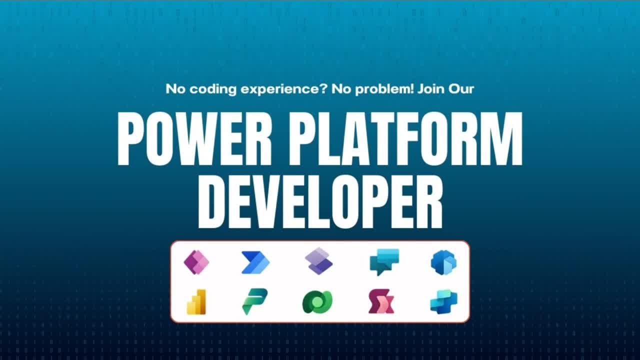 i. i have kept in a document to test the check it kartik, but as per you, kartik is also correct t-h-i-c-k. now what happens here? no, my uh bot will recognize this as a wrong and a complete flow will stop correct. again. i need to restart the flow and i again i need to go to change and release process. 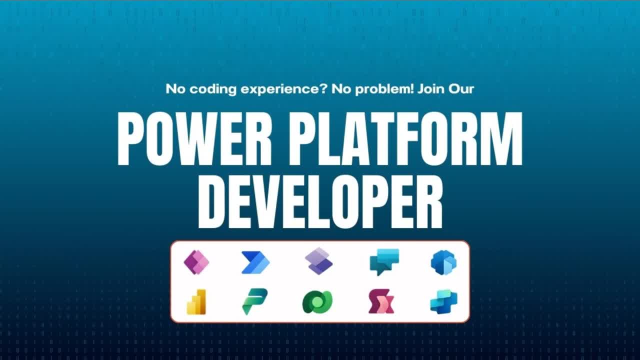 so any kind of testing use cases? still no, in my career i haven't created bots for testing. we have done excel automation. we have done windows automation. we have done, uh, browser automation, uh, we have done. letzten been doing some json jobs. we have Bart and in reading. 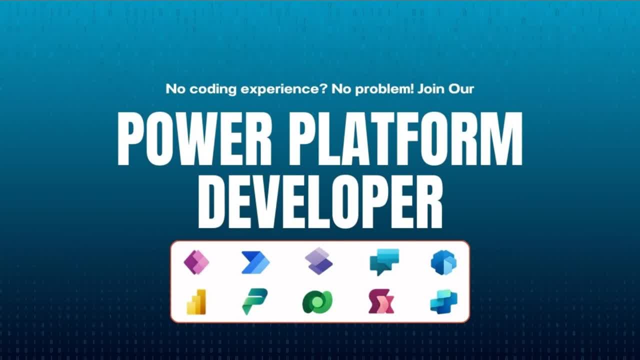 holds up the site nowPoint. sorry. sorry, i had no ns西 parce i will do it tomorrow. אם the device is damaged, fire meço. i wi laughed at the speech. you or ever write it on facebook. done sales force automation. we have done sap automation using rpa, but you know testing. 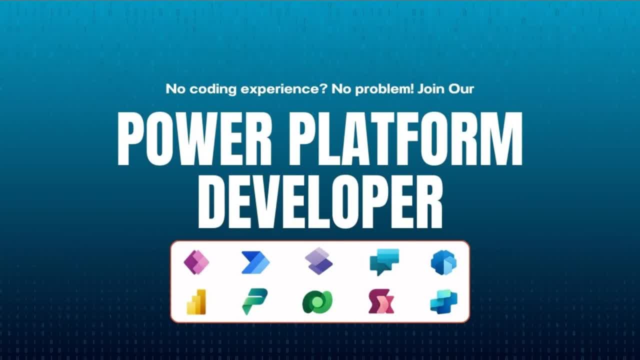 automation. no company have given me that, but it's a good question. uh, your, uh. your question definitely deserves and asked. but you know there are not no such use cases. so, for example, if i have a sql code, so i'll be validating from sql, i'll be running the those sql code and i'll be. 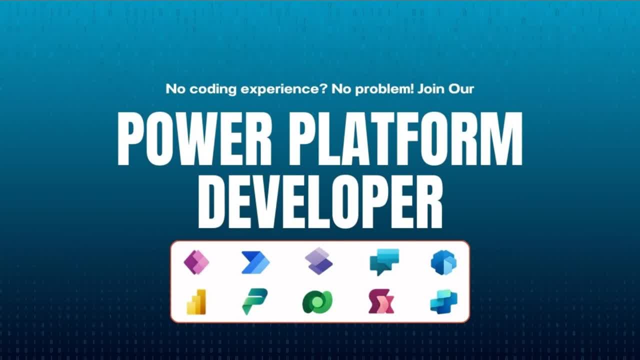 checking with the power bi ui the values, the insights are matching or not, if it? if it is that case, can i, can i do any automation using power apps or power automate? ah, probably see here again, it's going to be a severe task for the bot, okay, so usually what are the use cases for uh bots? is that? 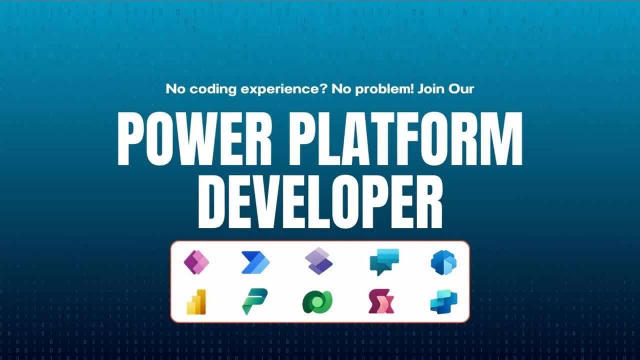 which are repetitive tasks, like if someone goes to excel sheet. so some uh something like some, you take a kia showroom, you take a bmw forum, they are like selling from each showroom in india. in india suppose there are like 100 showrooms. they are selling documents, they are selling the. 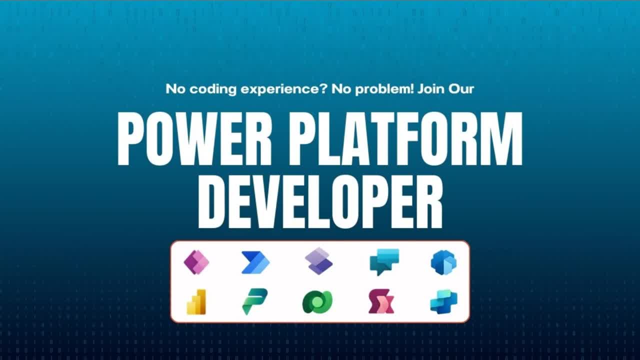 vehicles and they are selling, they are creating invoices and they will be giving this to some manual uh, manual manual person to enter in the main central uh central database. okay, they will be storing uh. so once i, once i invoice is generated, they will be storing in them. 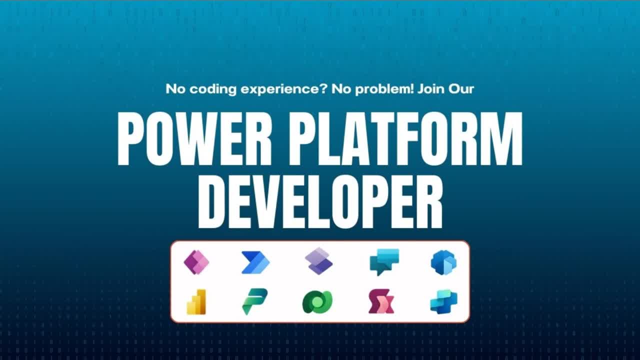 their in their respective shared drives and some manual person will go and pick those columns and will, uh, pick them in the central database. these kind of things. we will create bots using rpa or, or we can do it with power automate, specifically, not much with power automate, but power automate desktop. we do this kind of sales automation and we will do. 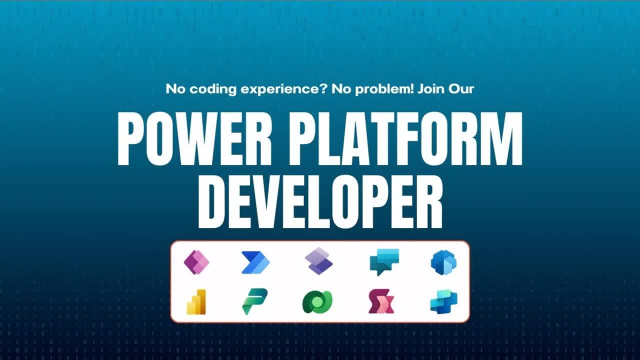 the default: uh play uh kinds of uh commands and uh and uh, something like we want to get. so some, some invoices, uh, some sales taxes are generated in sales reports, main invoice is generated. so someone need to go and log in every day and collect these two invoices. 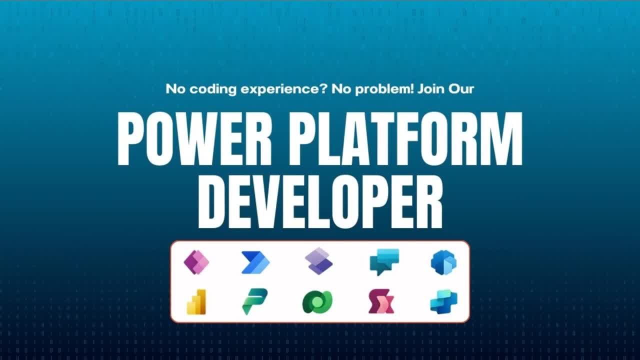 and store them in a another uh database. this kind of things we can automate, okay. but uh, we are good Annapurna, I am working in one of the MNC which I would not like to record. yeah, I worked for various clients, like in a non-recorded session, we will. 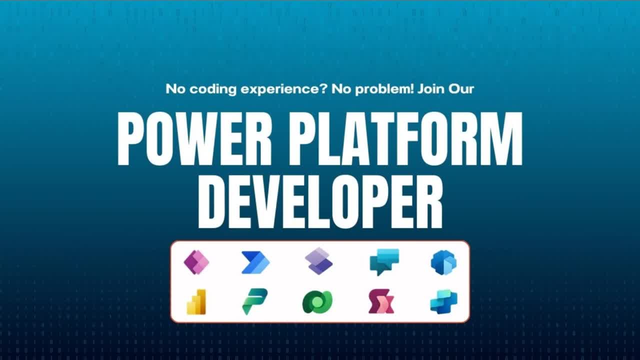 do. okay, we will have a greet and meet and that I will give you more insights on where we have worked and what we have done. okay, so I would not like to reveal my company directly here due to some policies. okay, Annapurna, Annapurna. 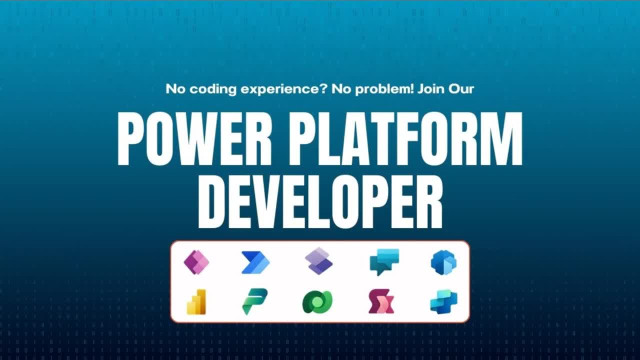 last question: I have, yes, Suraj, not Suraj Bala here. yes, Bala, hello. okay, so in power to make it okay. okay, so in power, into power, power upstarts. are we going to cover le the third party? okay, uh, SharePoint is a third party integration. uh, we will integrate that. 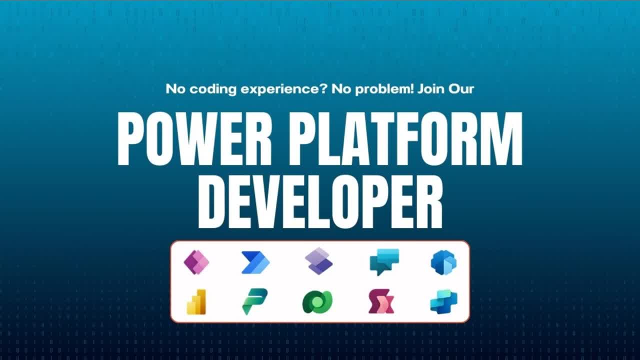 one. if you know integrating SharePoint, now it will be easy for you to integrate a sales force. it will be easy for you to integrate SAP. it will be easy for you to integrate SQL in the same way. Dynamics also you can Dynamics. FN also you can do any other kind of SAP. 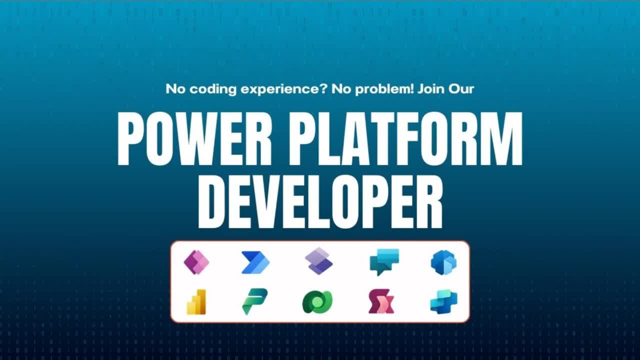 you can integrate. to take any of other, I will show you the credentials of SAP and say it supports based on your project. I will integrate it, okay, hello, yes, yes, I'm Sapna. I have a long, 15 years of break. I am in teaching side. I am trying to learn software side. 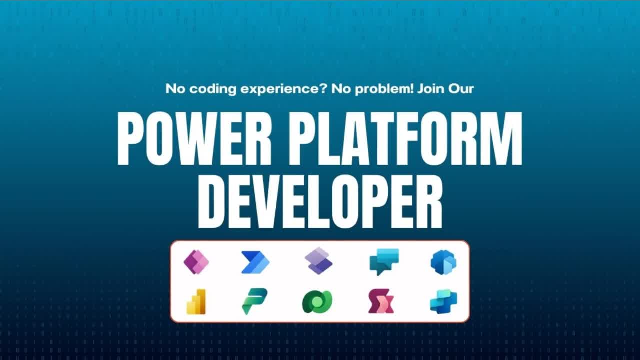 is it possible? we will discuss about the possibilities separately. Mahesh is there, we will guide how it works, okay, sir. thank you. hello Rajesh. yes, yes, Bhaskar, but thanks, there are Telugu people. I think there are no Telugu people, but it's a combined session. we can have it in interaction. 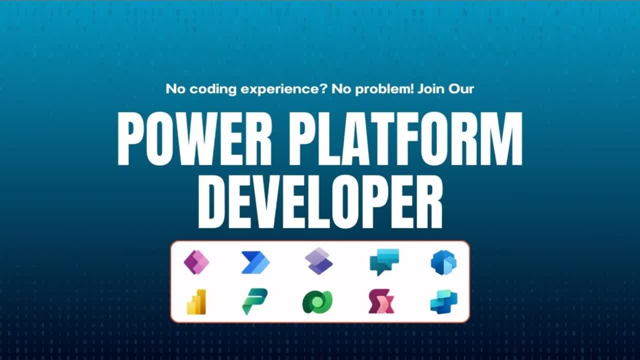 no problem, atleast no problem. I also have a small doubt, as same as Swapna. last time I was in UiPath I worked for 2 years, but from 4 months I have been doing power apps for 3 years. I have done 2-3 interviews, mostly about SQL. 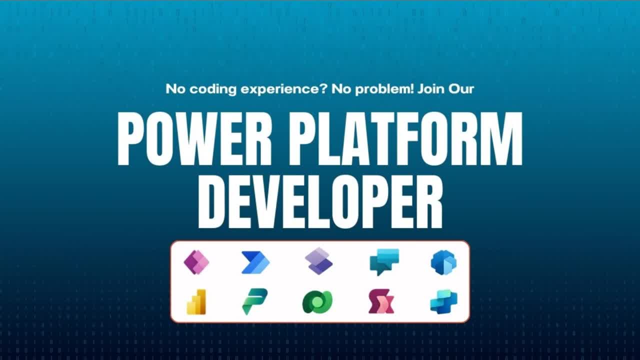 about SharePoint, about Power BI, then next to cloud, desktop cloud- sorry, power automatic cloud or desktop- about plug-ins. I am getting more questions, so can you completely explain about one project or two projects in overall touches in every tool. this is for everyone. I am answering in every tool. I will do basics. 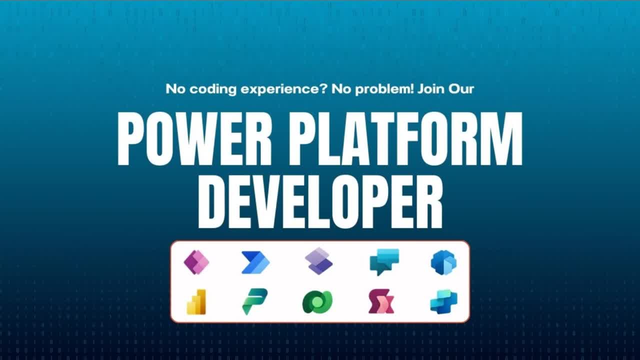 and I will create an end-to-end project, correct? yes, every tool, not only just one tool in every tool. I will first teach this fundamentals, then an end-to-end product. by the end of the complete 3 and half months, you will get what you want. you can easily clear the any kind of interviews. 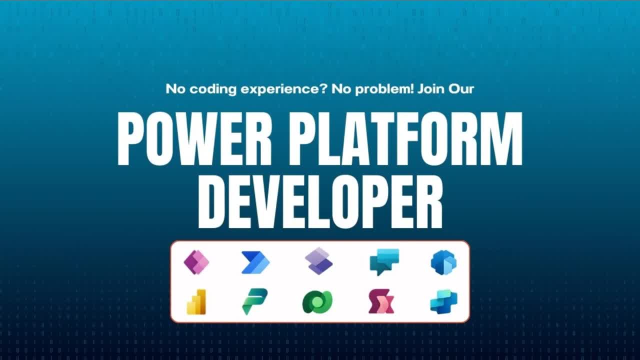 thanks and for everyone who are new: after our one month, one and a half month of training, we will push your resume to the job sites. it may be linkedin, it may be naukri and it may be indeed, etc. whatever we have, then your real game will start. 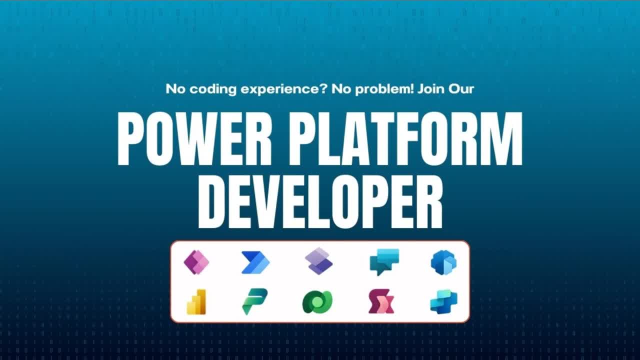 immediately after one and a half month. so that's the reason: by the one and a half month you will get what we call some tools. we will perfect. you will get perfect insights and some tools. you will have an overall understanding and based on that only I will give. 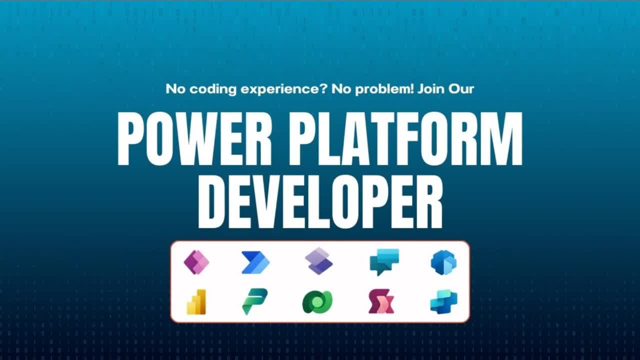 at least keeping the scenario that you should clear a screening round. what I will do is I will conduct the lectures, and this is most effective, and this is only I am following and the success rate is also high. at least two tools I will fully complete- ok, and remaining tools I will give. 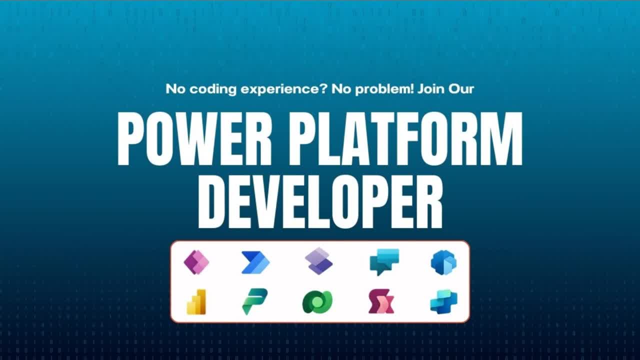 I mean, like I will give you some overview and some integration part, because all the tools in power platform are interrelated. interrelated. you cannot like dismantle one tool and no, no, no. I just want to work on power app, only. I want to vacancies in power app, only nothing. 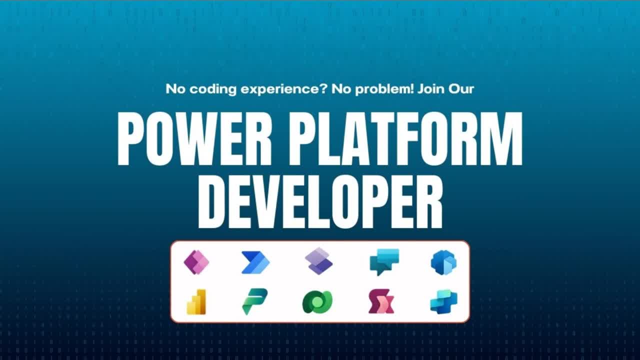 no, no, no, no. I don't want. I want to just work as an admin, because there will be no coding part. no, no, no, this is not possible at all. I like power automate cloud. it is having triggers and triggers and actions, actions. this is very easy for me. 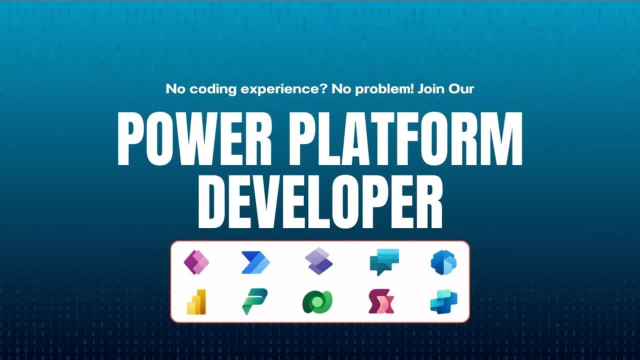 never come with that attitude. you come. you give equal importance to each and every tool and within one and of one, your confidence will be such high if that too, if you come regularly to the class. don't miss the class and kindly connect from mobile. don't connect from mobile from tomorrow. 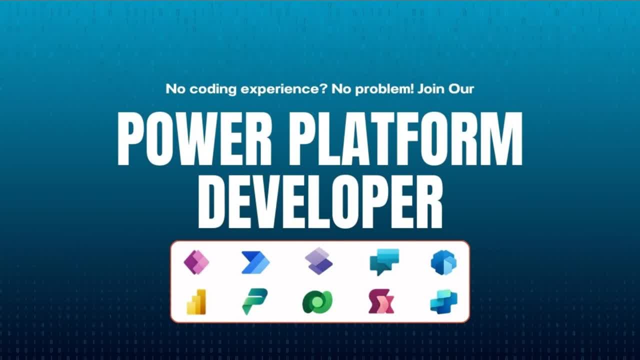 since these are free sessions. I even didn't ask till today, but from tomorrow you should be able to connect. you should be doing hands-on along with me, at least for some days, after getting some grip. yes, these concepts are covered. it is, I am strong. then you can attend, because this is a morning session. 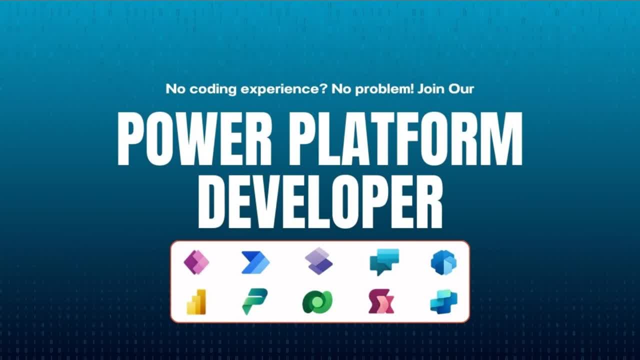 I can also. I cannot also not insist you. some people may be working till the night and some people may be doing their household works. sometimes we may get some special occasions, like some relatives might come to our home. in this scenario, you take it into consideration and you can connect from your home. 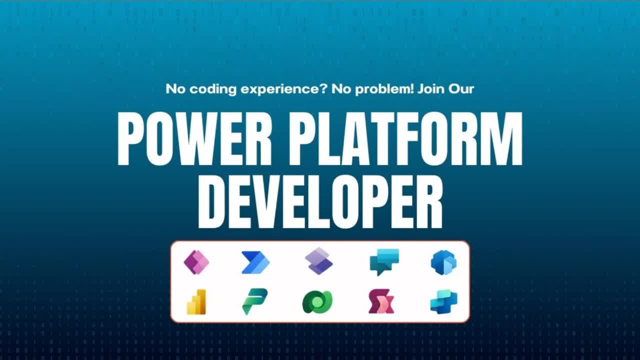 with the convenience of the mobile, but especially for the one and a half month. for one and a half month, don't use mobile phone to connect, connect with the laptop and whatever. I am practicing here based on the availability you do practice here, at least if I am covering 100% as a practical. 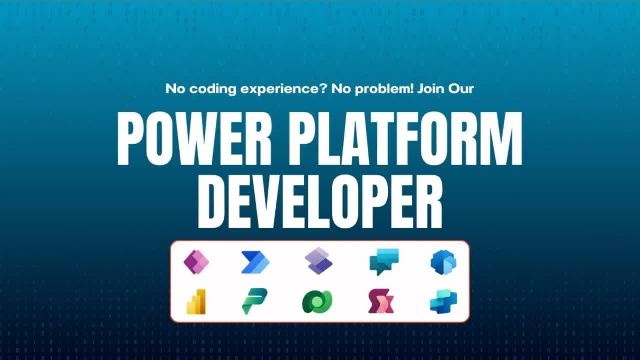 you should complete 50% in your laptop simultaneously. so this is my expectations from tomorrow. okay, so, Raj, only power. so power app is not enough. so you are saying, like Suraj, it depends. it is totally yes, yes, Annapurna, each and every class is recorded. 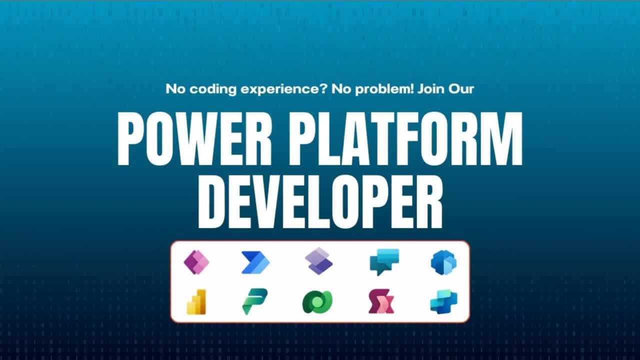 and in your login you will have all the videos, no issues, every class you will get. okay, yes, Suraj, yes, until you get job. until you get job, you equal importance to everything. but once you are in the job, your manager will recognize your skill set. based on that, he will assign the task. 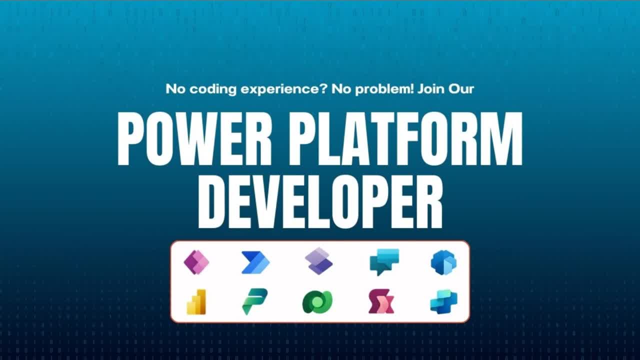 but I am saying you clearly based on the situation, based on the company. if you have more skill set, if there is project in power apps for three years they will continue as a power app developer. but suddenly they got a project into power automate. they don't have a power apps project. 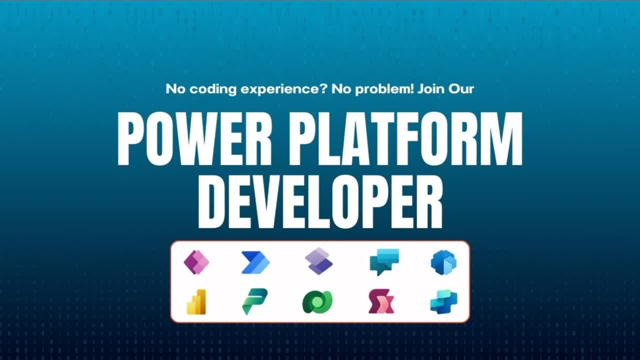 if in that situation also, if you stick, even suggest with just a power apps, no then it may. it will be like a trouble to you only, but my sincere advantage is you equal importance to everything and everything is like easy only if you understand and get the use cases correctly. 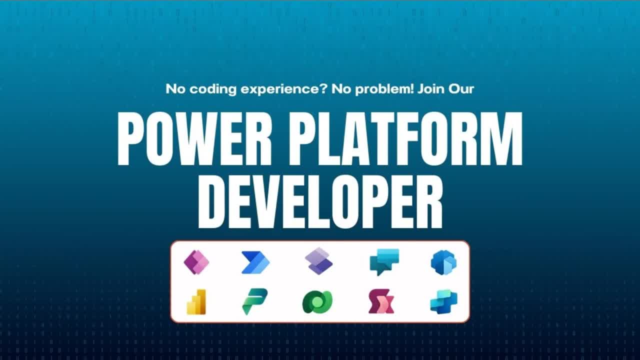 and understand the basics. believe me, everything is easy. only in the three and a half months. definitely you will become more perfect than me. you will ask more questions than me, you will. you will work more than me, because this is going to be all fun. no coding, low code. 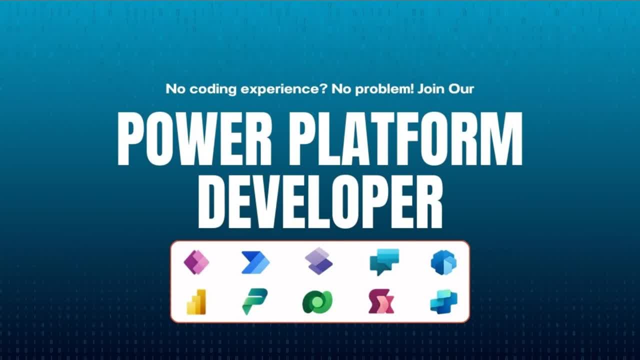 okay, Suraj, never keep, at least until you get the job. at least you get until you get the job. give equal importance to all tools. okay, after you get the job, you say to the manager: I am work, I worked 10 projects in power apps only. I give me power apps, power apps project only. 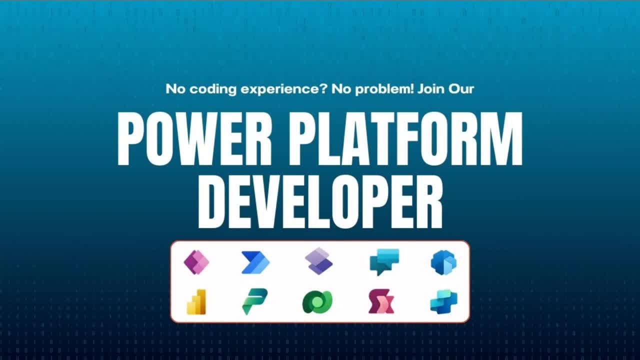 this is becoming tough for me. in this way, you can ask and based on that, also based on the availability: if there is an equal availability of that project, you will get, but don't dare. also getting a job is our main scenario and satisfying your client or your manager. 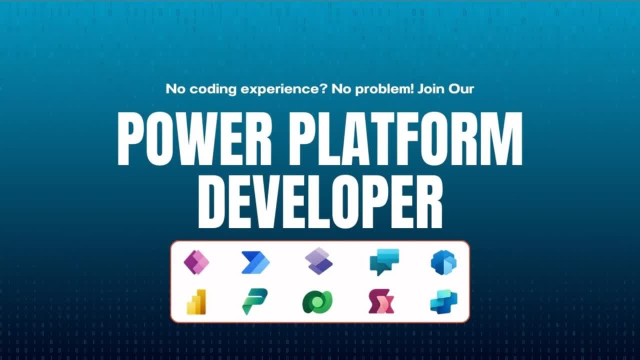 is the main important thing. but you can express what you want, even your. some managers will ask in which tool you are perfect. at that time you can openly say okay, but until you get job, don't give equal importance, because, based on their project requirement, they will shoot questions on. 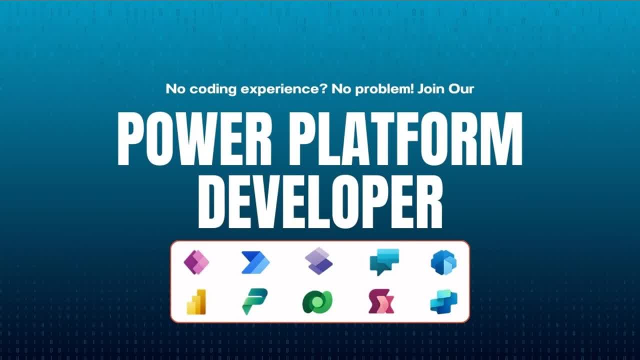 the respective tool higher. but power apps and power automate, you will get more questions. okay, and model driven application- this three, these three will have major portion of questions and after that you will get questions on PVA. after that you will get questions on AI builder, after that you will get questions on 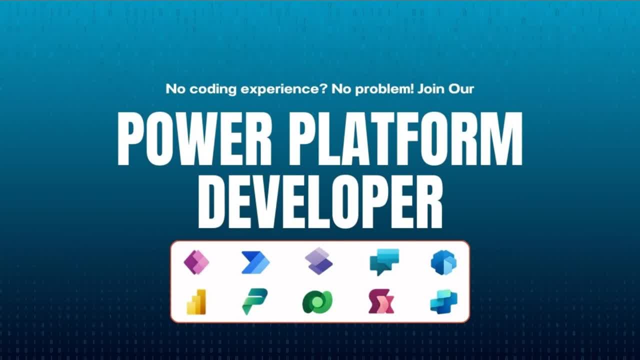 power BI. okay, power BI is a last, very less, very less, because already power BI developer will develop something and they will give it to you. just you need to understand that dashboard and you need to integrate it. that integration, if you know, that is enough, okay, and minimum basics. 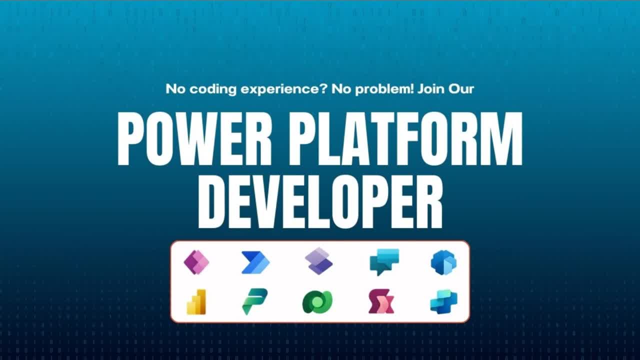 and what is required for a power BI, for a power for developer, how much skill and how much basic knowledge is required. that I will provide. okay, somebody said that SQL also asking SQL. here we will be covering two databases: one is SharePoint list and one is- huh, if you know, SharePoint integration. 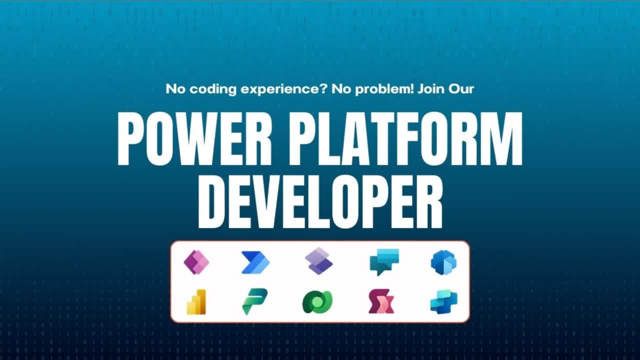 you can integrate any kind of database in the world, thousand plus connectors you can integrate. okay. okay, you, as a power platform developer you is, you will integrate a SQL server. you will not develop an SQL server, but if you want, you can get the recording access. we will provide the recorded sessions of SQL. 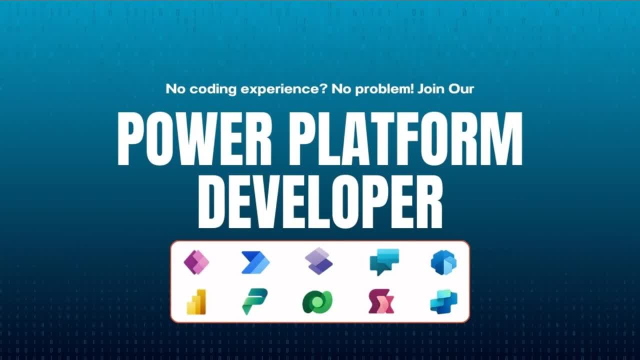 you can also you can go through your database- will be become stronger. that arrangement I can give. okay, yup sir, hello, yes, yes, who is this? hey, man, sir, I am Shiva Shiva. yes, Shiva, sir, I am from non technical brand. okay, coding software. about the coding. 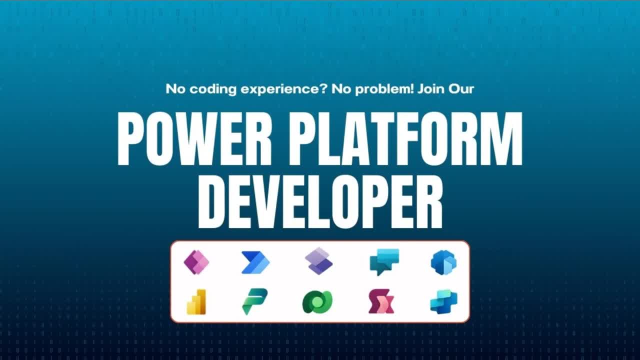 here. no coding is required, Shiva, just your analytical skills and your what we call mathematical skills are required. you told me that you report class about the C sharp. that is for a. he is an advance. he is already working. no, he is working as a CRM developer. 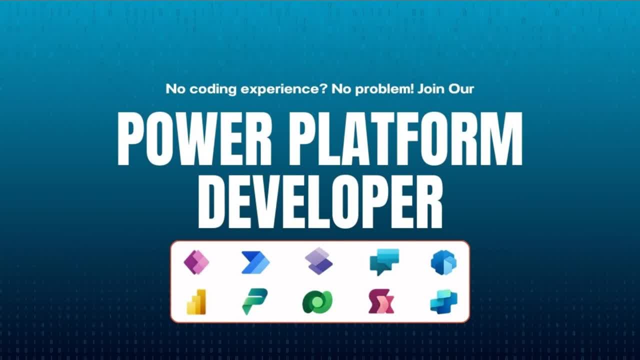 that is a reason they are asking him more on a C sharp and dotnet. you will be introducing yourself as a power platform developer only, and interviewer also will know a power platform developer will integrate plug ins- okay, plug ins, but not create plug ins- okay. thank you sir. 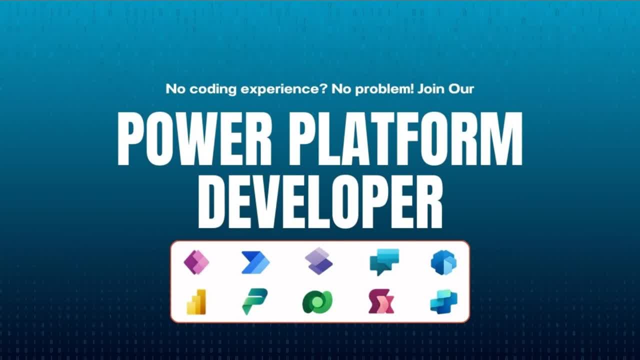 but it is better that you work on. don't go to C sharp you in your free time. just learn javascript to build logics. to build logics, you learn javascript. no one will ask questions on javascript. don't fear, in interview no one will ask you questions on javascript. 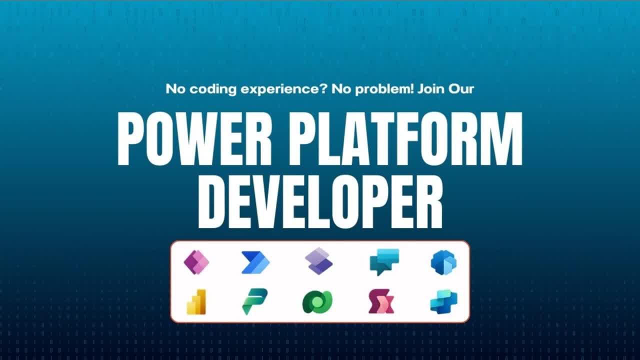 but in order to handle some situations in your job profile, at least few basics of coding are required. Shiva, okay, sir, but since you are from non technical, no, just try. I mean, like you just play with those kind of javascript. okay, javascript will be useful for you. 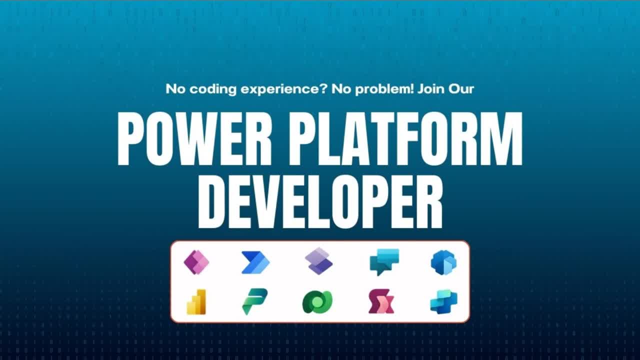 everywhere. okay, sir, got it, thank you. can we go with rather than with python? sorry, can we go with python rather than java script? here? we're not data, already python. what python will do? all those things are integrated in our PVA. okay for virtual agents and builders. already they were okay, uh, and when you are like you, uh, did you have? have you seen? uh? 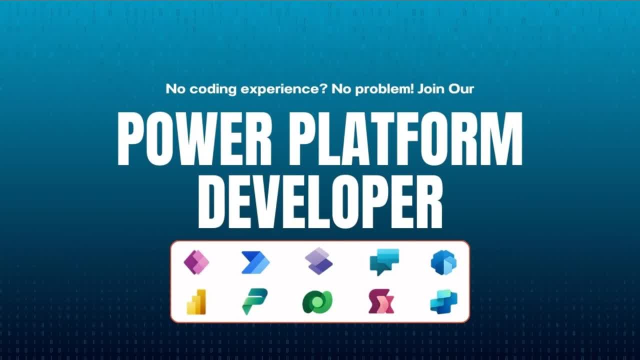 our, our, when we are creating. have you seen our demo like when we are taking the picking the controls? yes, yes, yes, uh, when we are picking a controls, an unknown language- that is a, uh, machine learning language- only an unknown language- will come into the picture and it will. 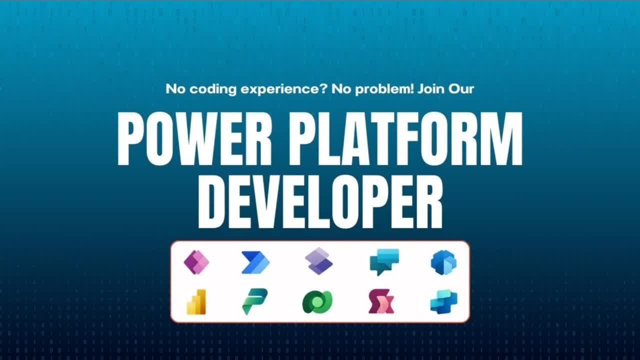 create a code backend and that code i will show you one day. so we have created just one or two screen apps, but for those two screens nearly there will be a thousand codes of line which will be created by already some ai language like typically like python, and we are not pretty sure. 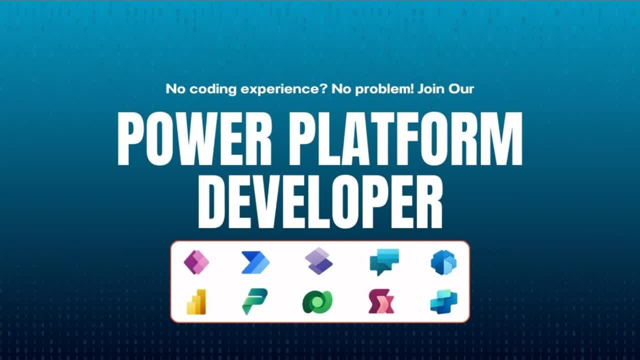 that is the business logic of microsoft, and we are not pretty sure, but we can see the code. so it's like we took just 20 minutes or 15 minutes to to create those two ui screens. but besides that, a css code will be written by itself, only by the power platform itself, only a, a html code will be. 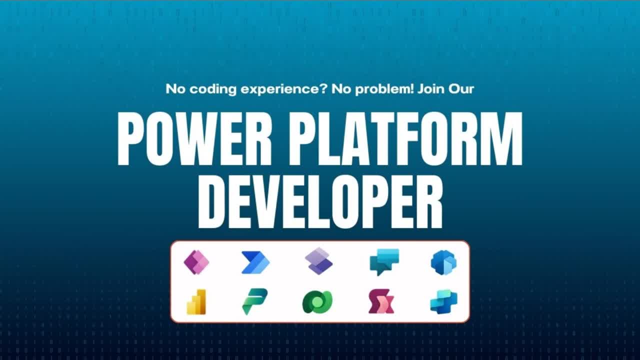 written and a yml file will be created by aml. okay, these are all done already by that tool. okay, now you need to guide that tool in a proper way, what your business required. so, if you have time, go with python, it's not wrong. if you are learning something, no, uh, it's always good, only. 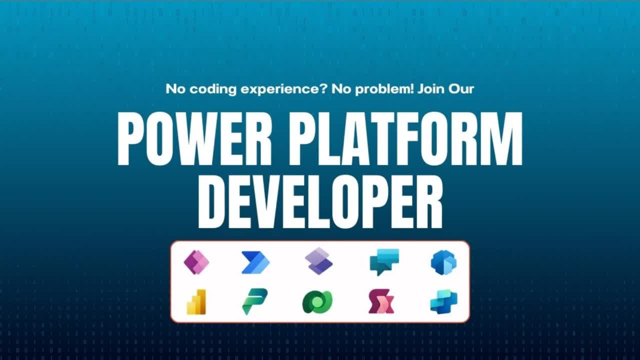 if you are more into programming, go with c, sharp and dot net and if you are less into programming, go with javascript. this is my recommendation as per the market and as per the requirements across the globe. we'll be covering f and o. uh, f and o. i will cover three, three parts, and i will try to 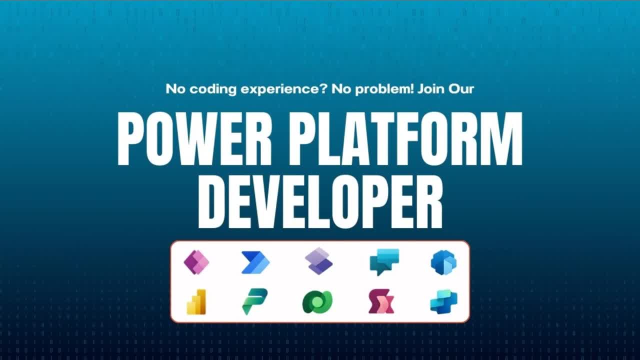 and i see more openings on will see more openings for power platform, dynamic crm. but power platform f and o combination is a very less uh. yet i will try to show you how we will integrate, how we will integrate f and o. but for this i valid uh, f and dot uh. i mean like f and o license is required and fno uh the remote. 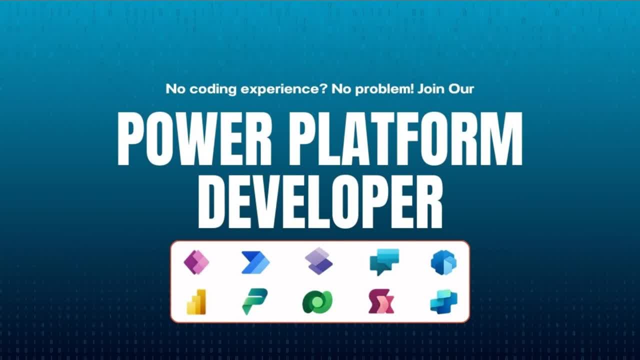 desktop rds connection is required. we will try to fetching it from our end. but especially this is a very costly tool, so we will try to fetch it from our end. but especially this is a very costly tool, so we will try to fetch it from our end. but especially this is a very costly tool, so we will try to fetch it from our end. but especially this is a very costly tool. 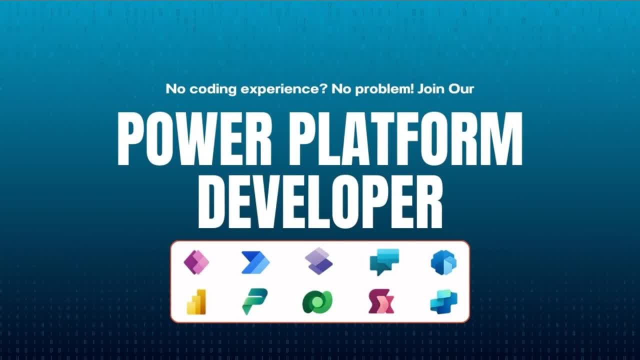 uh, but integration, how we can do, i will show you. no worries, fndo is something different. annapurna fndo is. it's a separate universe. okay, in power power platform we are having- and no one will ask a power platform developer to do a fndo work- that is a finance and operation.